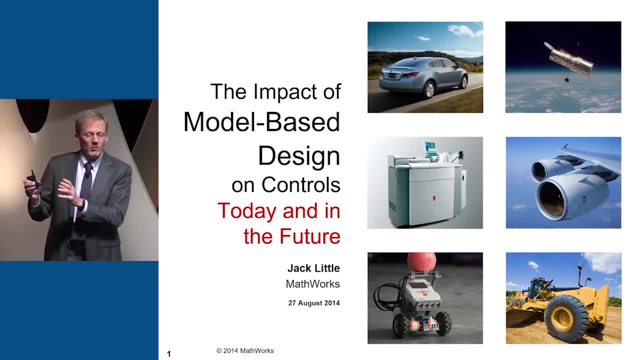 area. Simulink oddly worked in the reverse. It really was driven by industry. Industry kept on saying: here's these things we really need, We really want this, We want this. We worked with industry over really a period of about 15 years trying to respond to the 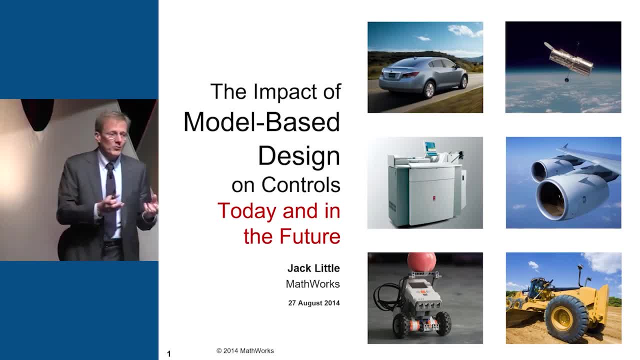 needs that industry had. It's actually been a little slow. moving back to education, It's kind of odd. Our product families each come from two different areas I want to talk a bit about again the model-based design and the Simulink side, and what I see as opportunities for. 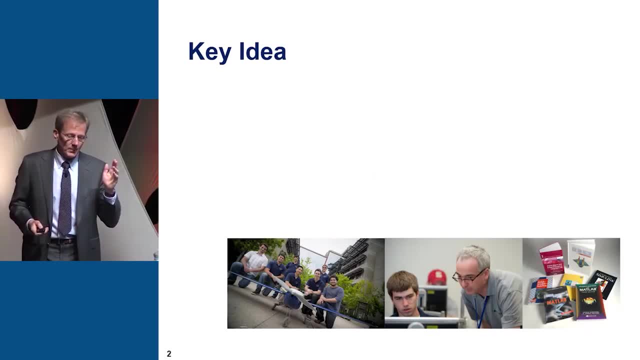 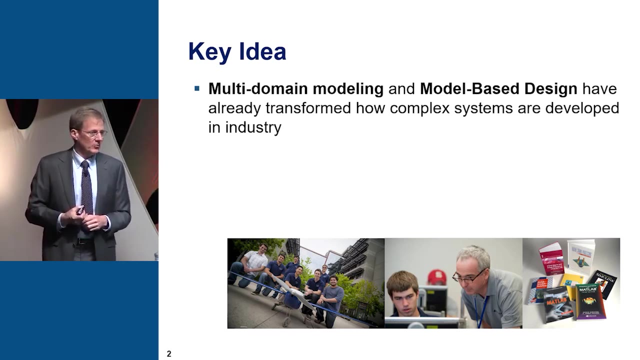 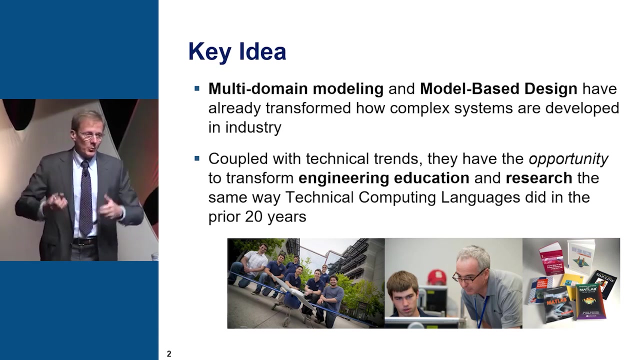 education here. I have a premise here and a suggestion for the future. My assertion here is that multi-domain modeling and model-based design have already transformed how complex systems are developed in industry. I'd like to share that with you. Really, the other part of my key idea that I want to share tonight is coupled with technical 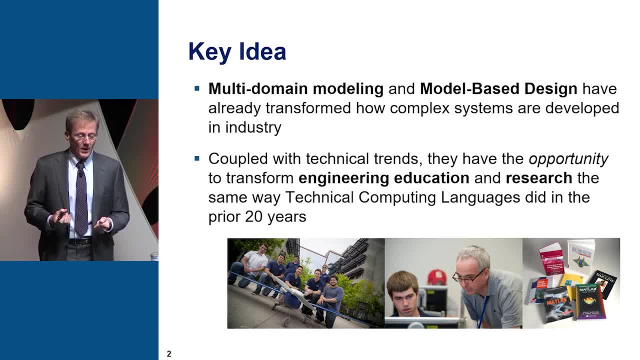 development. They really have a big opportunity to transform education and research and control systems, the same way that the MATLAB environment, the tech computing, transformed how things were done 20 years ago. I think there's a big opportunity. I'd like to talk about that. 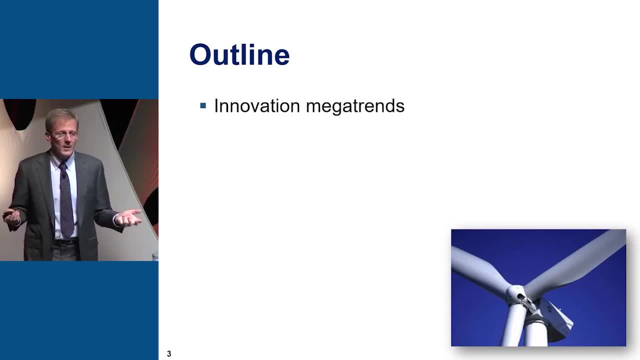 The outline of my talk. I'm going to start by talking about some innovation megatrends from the past 10 or so years, ones that really drove model-based design in industry. Industry ran into some trouble. There were issues that ran into. 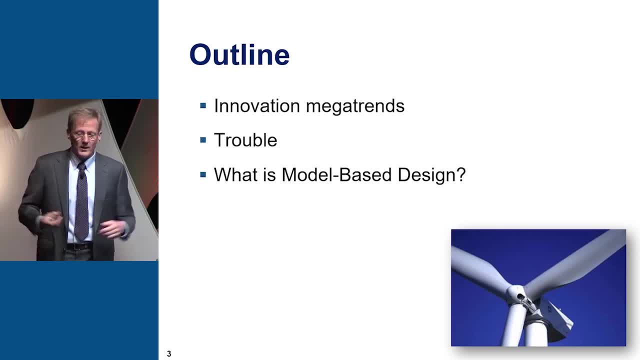 The solution arose in the form of model-based design and I want to talk about that. I'd like to share with you the impact it's had on industry and some insights based upon industry learnings. Finally, I'd like to suggest what the future impacts in industry. 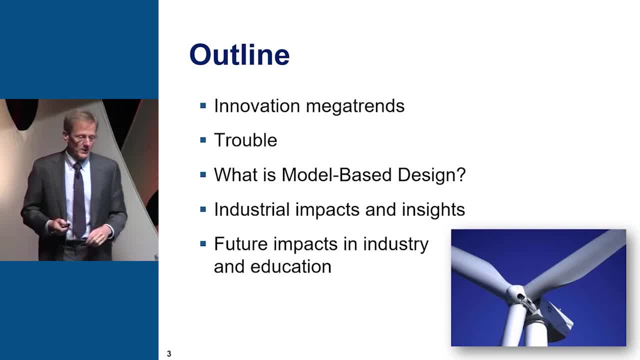 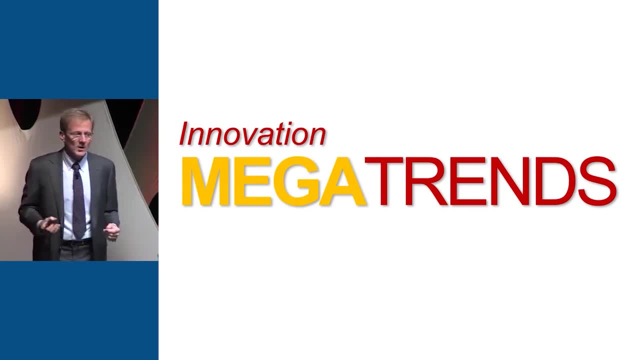 and education could be, and leave you with some take home ideas at the end. Okay, I'm going to start by talking about what I call Technology Innovation Megatrends. These are big megatrends that drive the world. These are things that businesses come into. 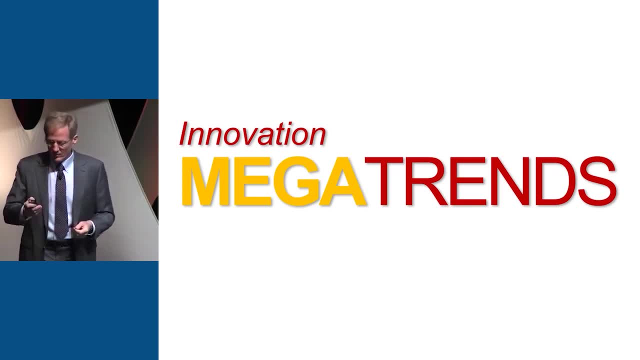 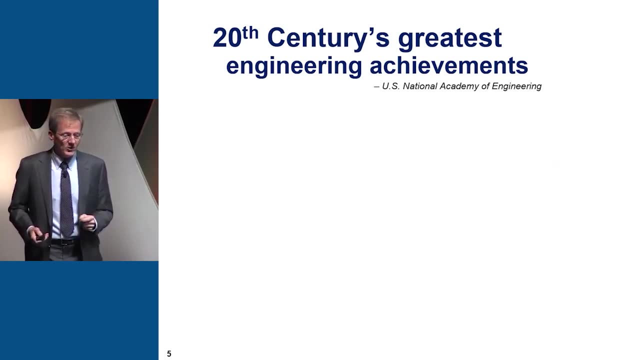 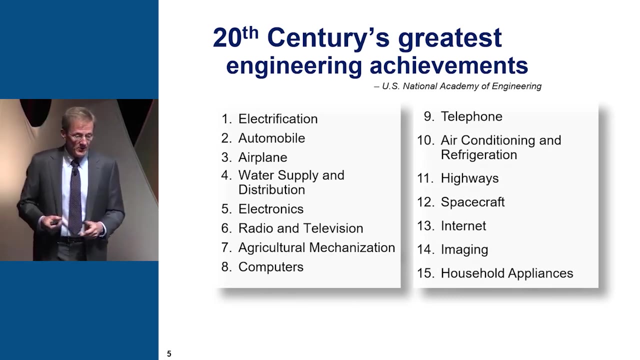 in being. whole industries come into being around these megatrends. So what's a megatrend? Well, the US National Academy of Engineering made it easy. They have a list of the 20th century, 20th century's greatest engineering achievements, And here's the top 15.. And it's: 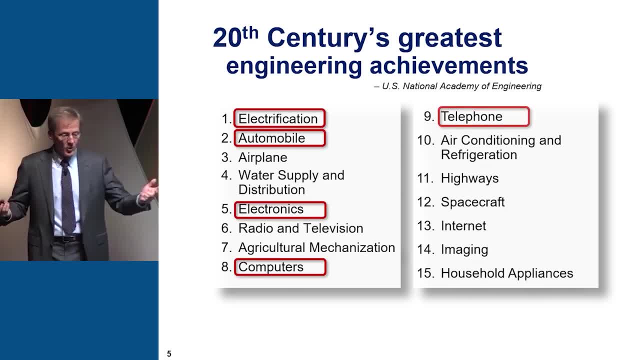 amazing stuff. I mean, look at this: Electrification, the automobile, electronics, computers, telephones, spacecraft. Now, these all happened in the 20th century. You know, basically in the 19th and 18th century science made fundamental discoveries in biology and chemistry and physics. 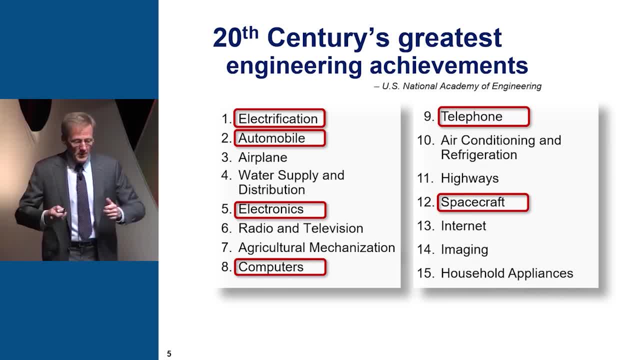 But in the 20th century the engineers turned these into amazing set of things that affect all of us in this room. A hundred years ago, we'd all be riding horses. The Model T first came off the production line about a hundred years ago. Prior to that, you know, cars weren't. 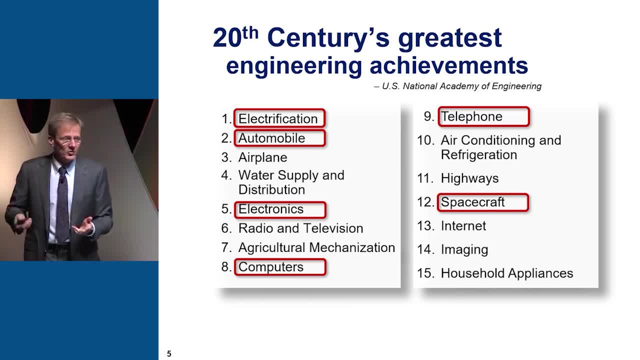 available widely And you know incredible transformation to where we are here, coming from all over the world. You know lighting and air conditioning, computers and all that. It's really, really cool. It's quite remarkable. If I could add one more to this list, of course. well, actually. 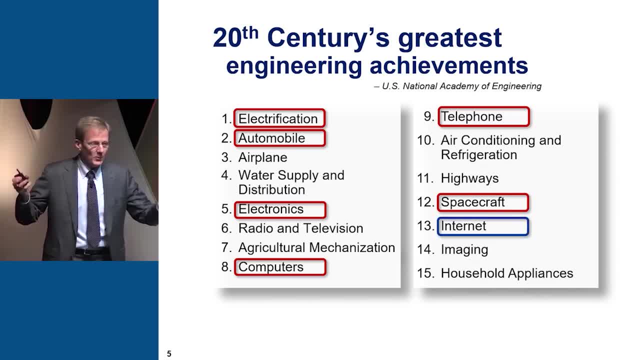 one other thing. Look at the Internet. The Internet, of course, which is a more modern thing that we all think is such a huge innovation. The National Academy of Engineering only gives that 13th on the list of things there. just to put it all in context, If I could add one: 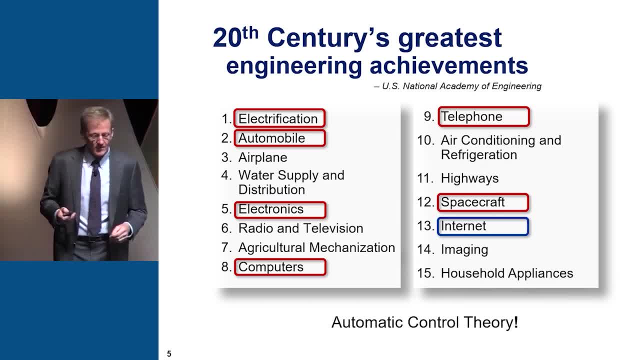 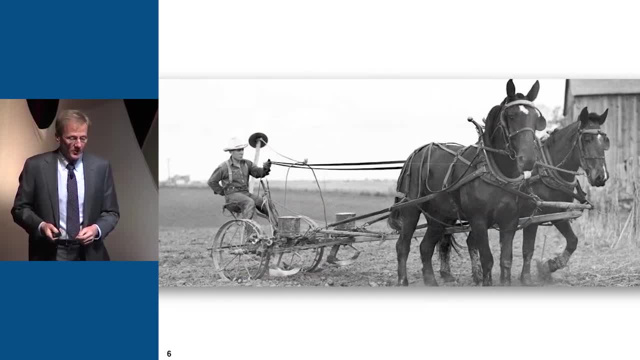 more. of course, I'd add automatic control theory to this list, but I'm biased. Okay, so, truly, these things transformed the world a hundred years ago, From this, you know, to where we are today. You know, it's just, it's really a technical marvel, if you. 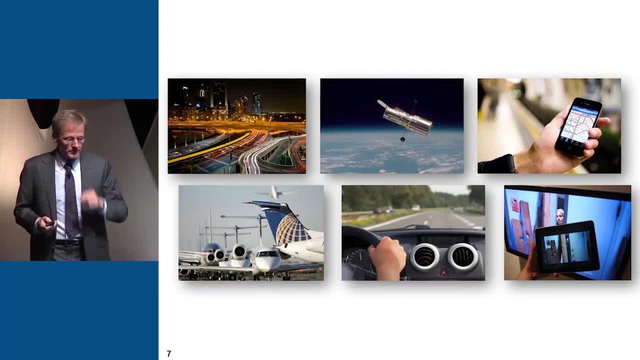 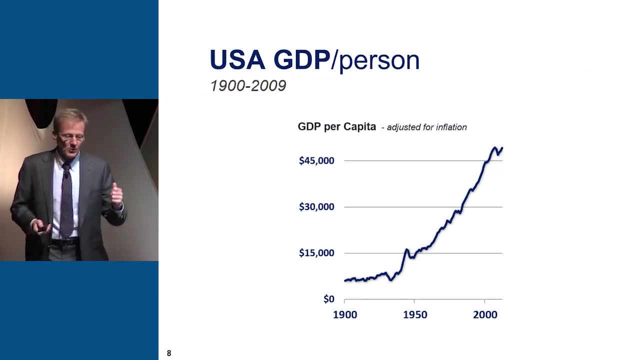 sit back and think about these changes that happen in the world. If you have any friends that are economists, they'll tell you. these are important, too, to economies and standard of living and quality of life. This is a chart that shows the growth in gross domestic product. 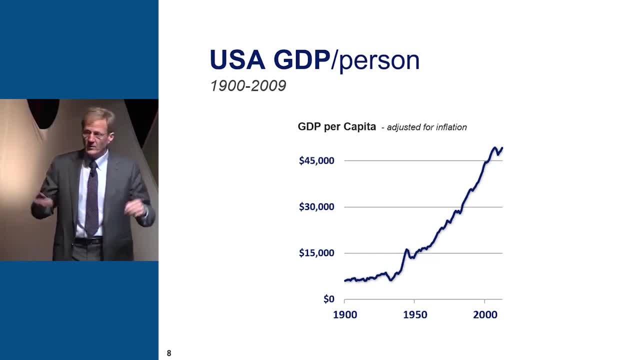 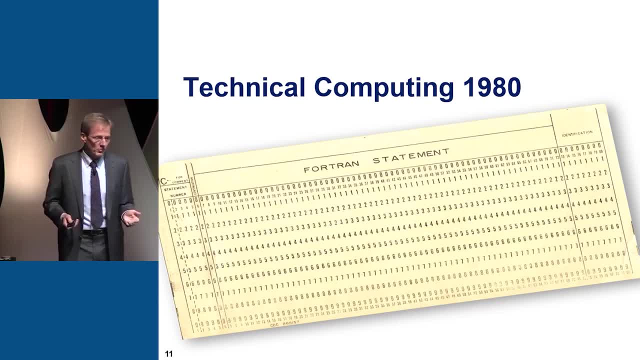 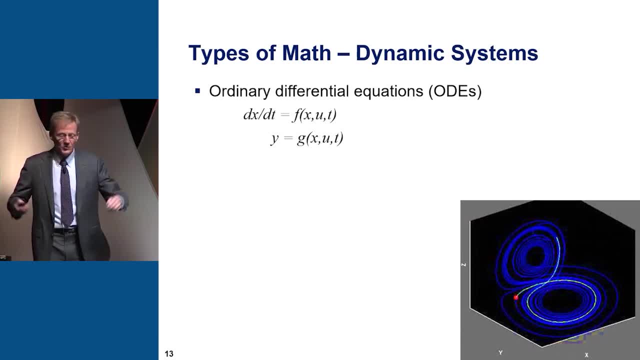 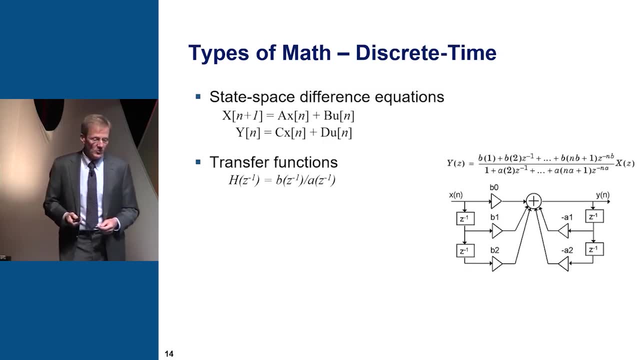 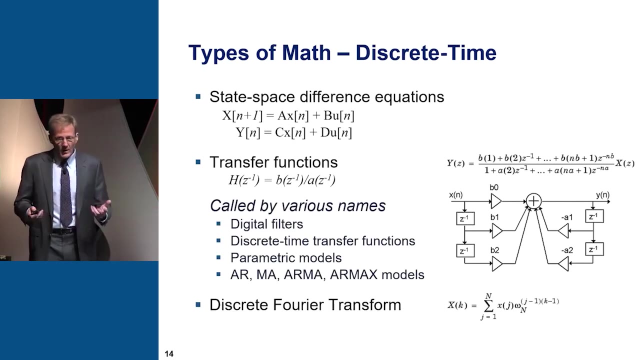 from linear algebra differential equations, their state-space form in linear, the transfer function form. Also important were discrete time models, state-space difference equations, transfer functions, all the different names they're called in different areas The FF transform. So a lot of these computational tools were new and understood. but this is 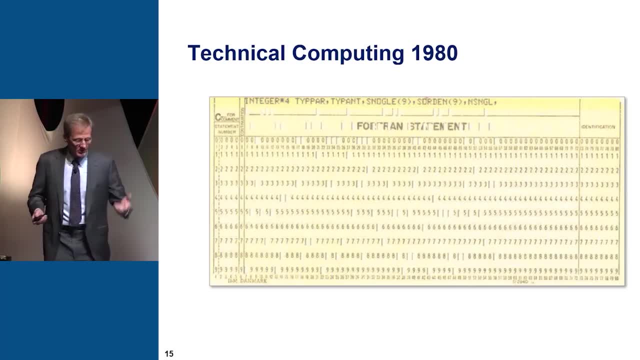 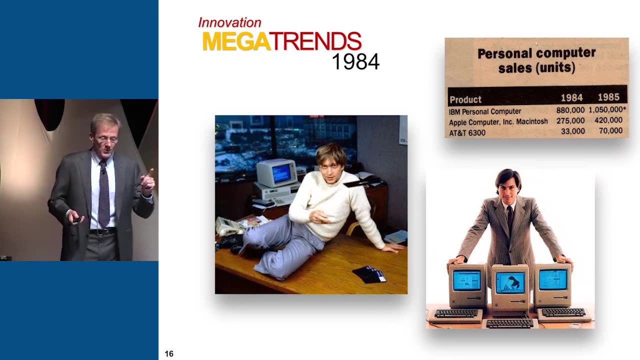 what we were using And what came along. The big technology megatrend is shown by this: a young Bill Gates and Steve Jobs and really the birth of personal computing. You can see in this clipping from the newspaper at the time that there were a million PCs sold that. 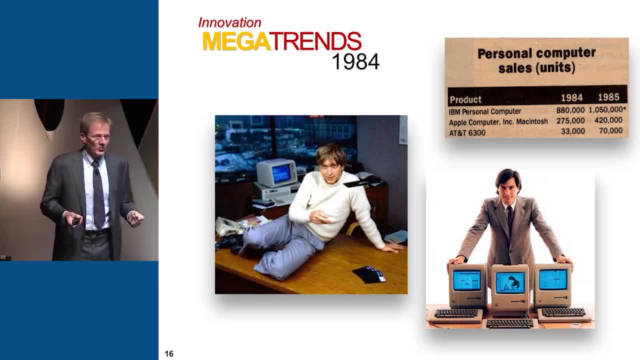 year. Today there's over 300 million sold every year. So if in this room full of about this many people, if you divide by 300, you know maybe there would be four of you in the room that would have used a PC in the room. You know this was an early-stage thing. 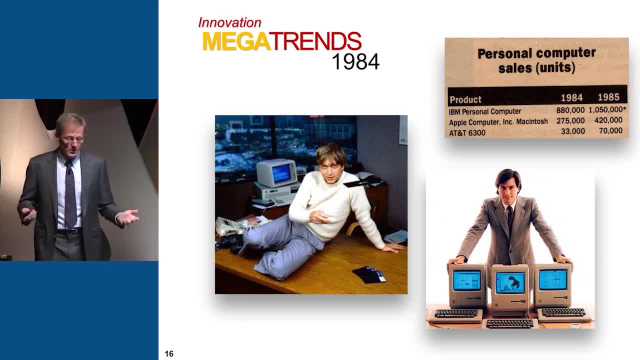 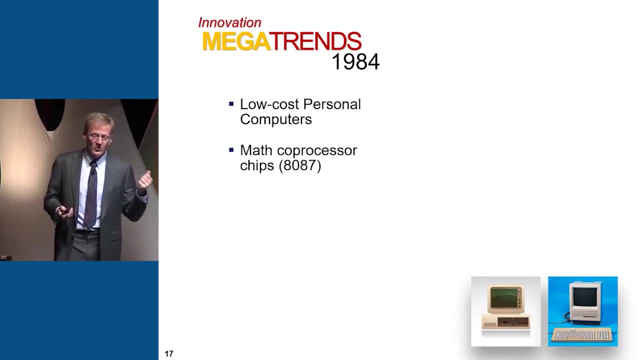 that not many people were using, And so the megatrend that MathForce took advantage of is low-cost personal computers. The fact that there was now chips that supported the type of calculations that were built right into the chip that we needed to do The whole birth. 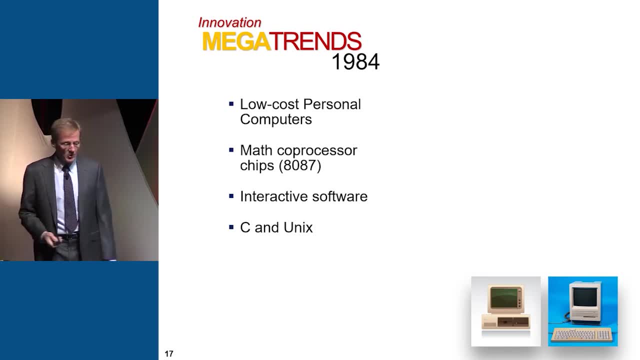 of interactive software, because prior to that it was Fortran, Birth of C, and Unix helped out, And then, of course, bitmap, graphics, Windows systems, mouse and so forth, And that led to creating MATLAB written in the C language. 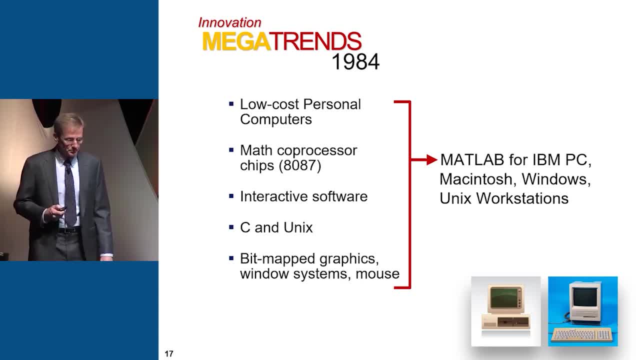 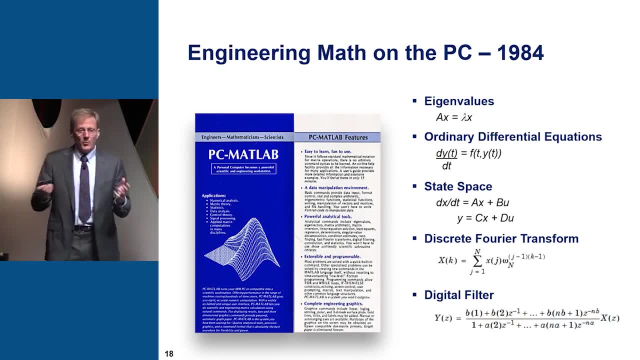 For a bunch of personal computers there. And actually here's the brochure for the first version of MATLAB in 1984. And it supported all these golden equations of control system engineering that were so important. It really focused on those types of things. 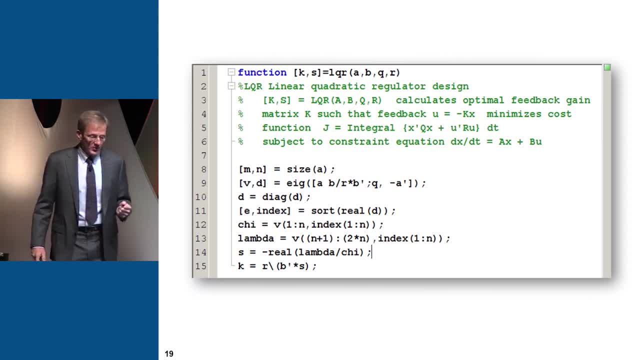 This is one of my favorite examples of the power of MATLAB. This eight lines of code here solves the linear quadratic regulator control solution, the infinite time solution. There are several thousand lines of Fortran code that were in a PhD thesis in 1970 at 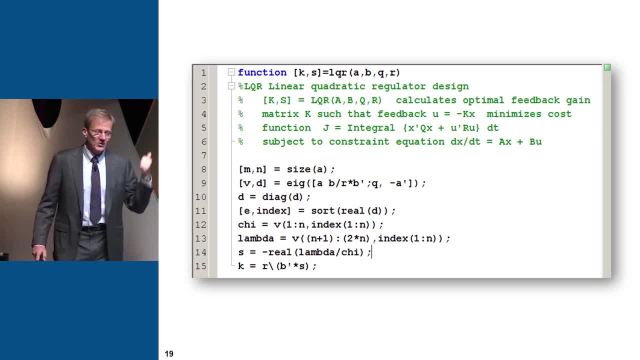 Stanford that sort of first provided a code to do this. So a 1970 PhD thesis at Stanford is reduced to eight lines of MATLAB code about 15 years later. And it shows. the power of MATLAB is that these are all matrices. You can work in a matrix form, which is a natural. 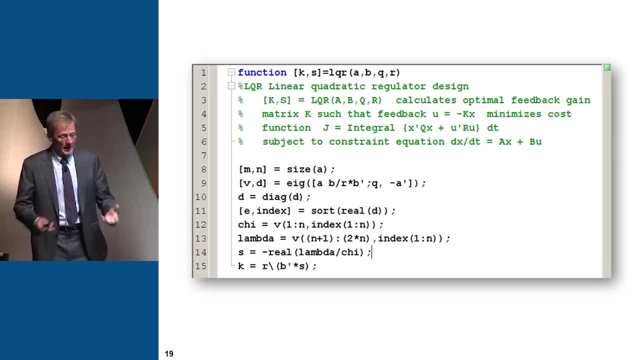 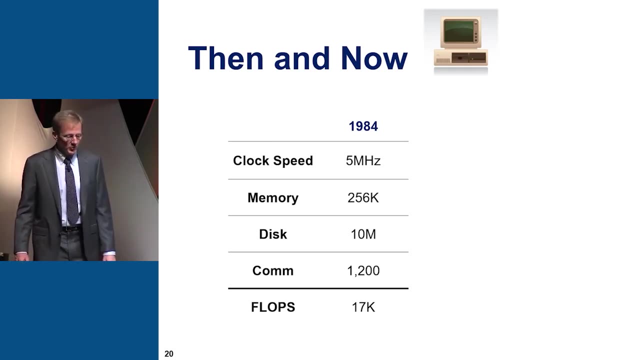 way to express it. So this is one of my favorite examples of why MATLAB caught on in the controls community. So this is the performance specs for a PC of that era. At the bottom it did 17,000 floating point operations per second. You can see it's 256K of memory and so forth. But then a wonderful 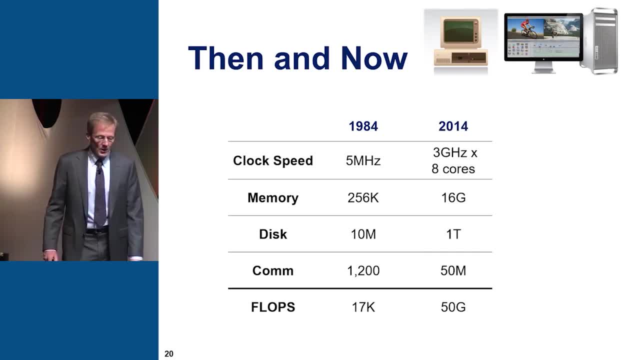 thing happened that few people appreciate. the extent of Today's computer has increased obviously by leaps and bounds in terms of performance, But if you divide those two to find out how much it is, they're extraordinary numbers. You know, the memory is 60.. 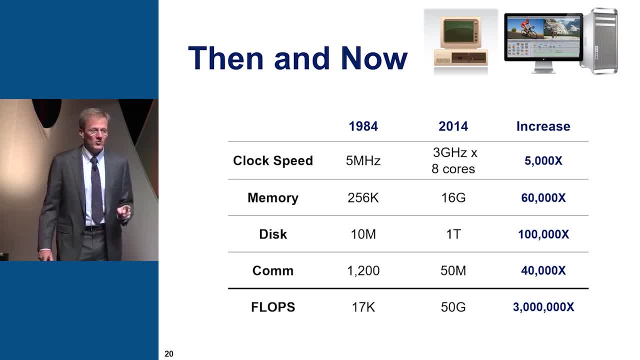 60,000 times more. The most impressive one, though, is the floating point operations per second at the bottom. That's over 3 million times more than those first PCs. okay, And that's truly extraordinary and enables a lot of the advanced controls. calculation enables. 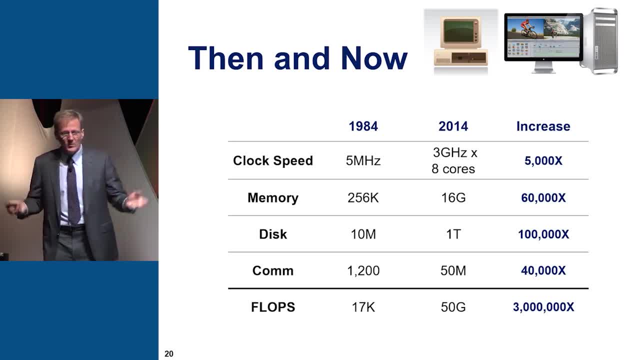 you to do amazing things in terms of software design and simulation and modeling. that wasn't possible back then and has been great for tools and great for embedded implementations. Okay, So that's what an innovation megatrend is. I'd now like to talk about some of the 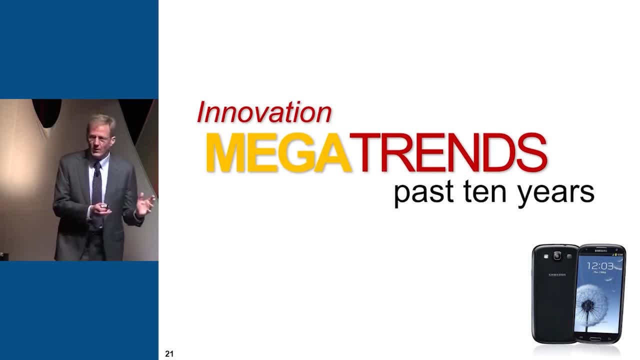 trends in the last, say, 10 or so years. I'm trying to set the clock back a bit and talk about what led to model-based design, And so I want to roll it back and talk about, you know, things that the world had, And really a big trend in the last 10 years is the beginnings. 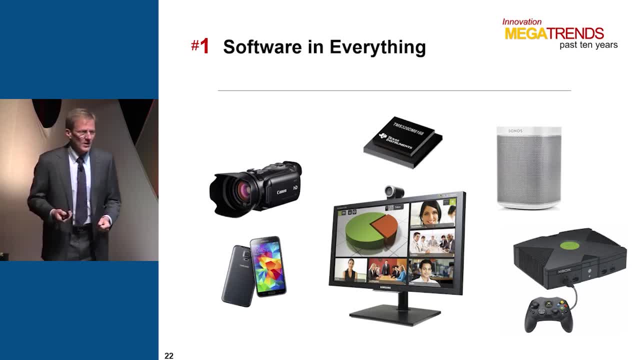 of software and everything. Software used to be on desktop computers, but over the last 10 or so years we're starting to get software in all sorts of things, And also not just any software, Also more math, more algorithms, more advanced things that have mathematics. 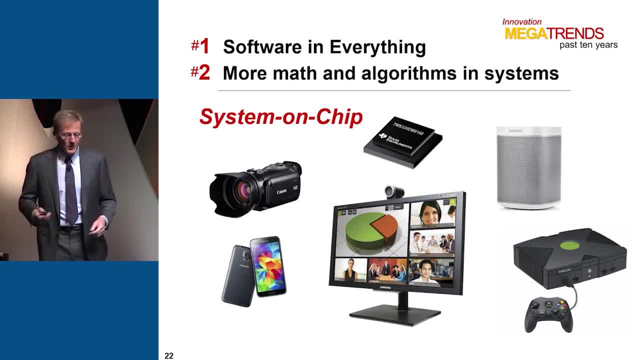 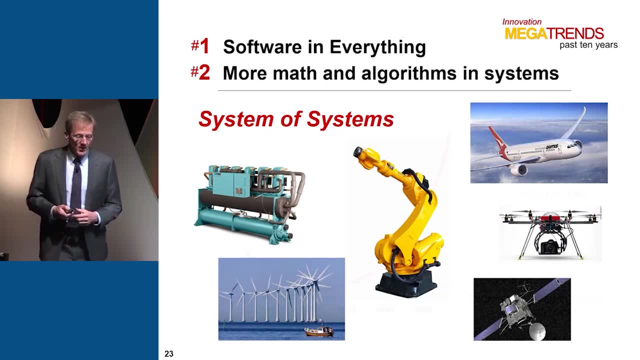 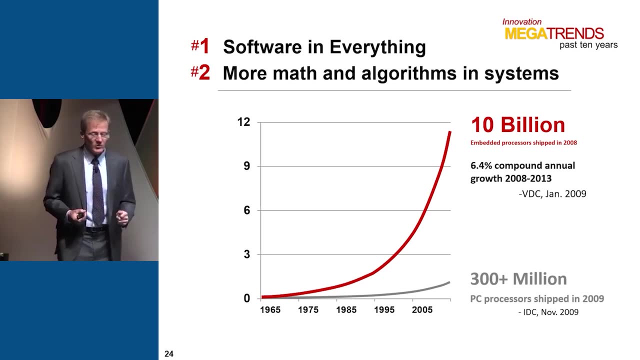 enabled by that And there's both systems on a chip. there is systems of systems where they're more complex and put together into larger systems. This chart shows illustrates the extent of how much this is happening. The curve at the bottom is the growth in processors. 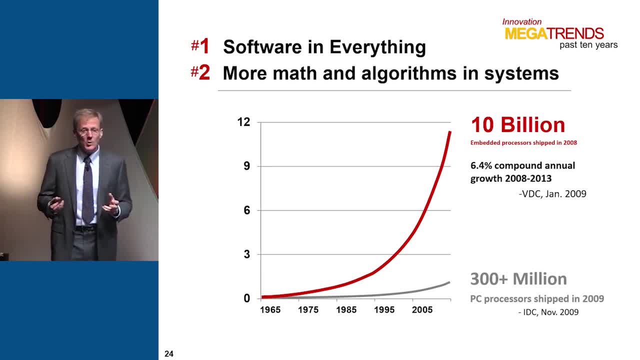 that are put into standard PCs, laptops and so forth. And while that's growing quickly, it's clearly swamped by the growth of embedded processors. And you just look at this and you say: is the world going to need more software and embedded systems? Is the world 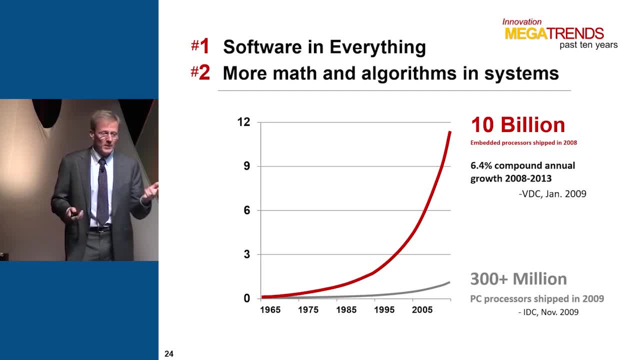 going to need more controls and more algorithms, Absolutely, And this is just an amazing megatrend that's facing, that was facing industry, you know, very clearly, suddenly, about 10 years ago, And it really is transforming. you know, here's a picture of a car, you know, maybe 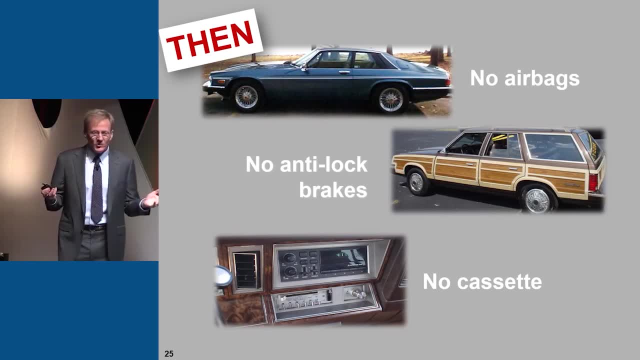 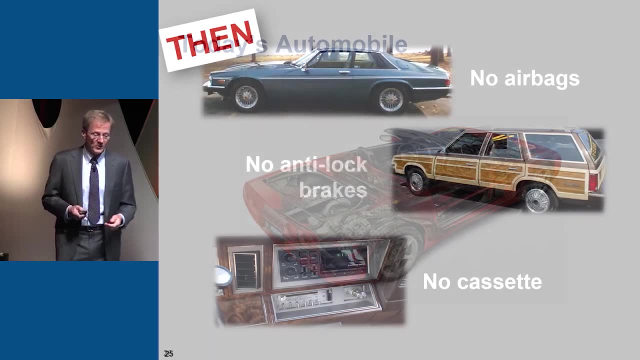 around 1980, a little before that, And I think the only transistor in the car was in the radio. okay, And you know, no airbags, no, any locked brakes, And that's over. the past 10 years has transformed to today's automobiles. 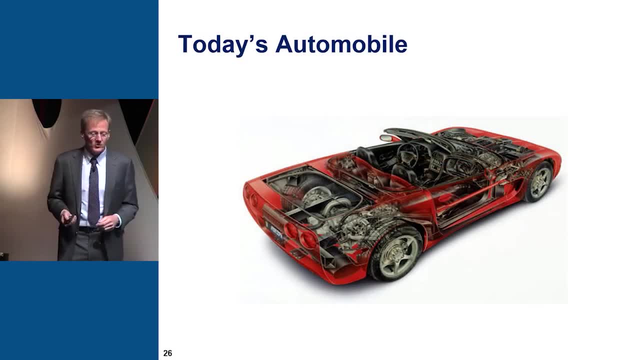 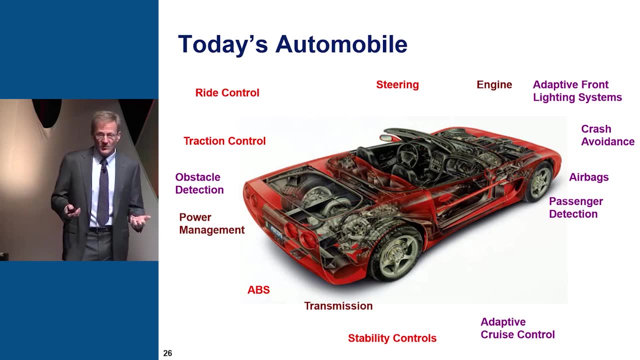 Where, where you have 40, 50 microprocessors, maybe even more, There's a set for doing powertrain, There's a set for doing chassis control, There's a set for safety systems, which, and then there's a set for comfort and convenience. Most people these days are buying cars based 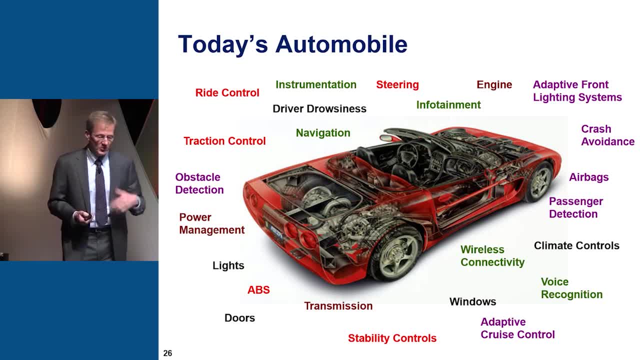 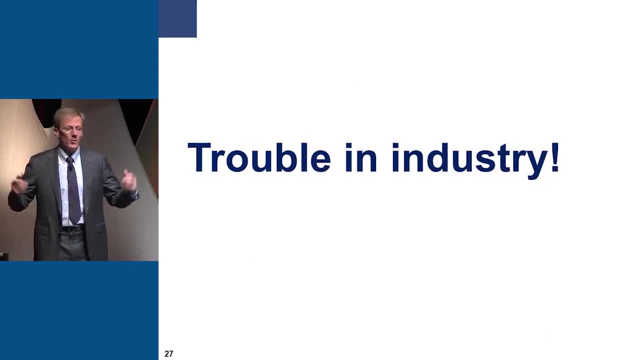 upon all these software features. You know, the basic car is pretty standard, but it's the software that differentiates, And and and, so there's enormous transformation Along the way. industry ran into some trouble, though. okay, It wasn't so easy to scale. 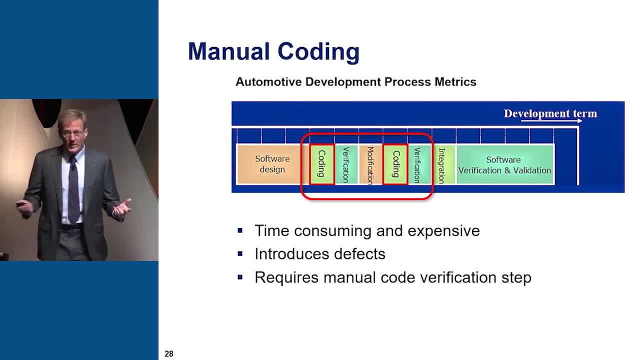 It wasn't so easy to scale up like that. Here's one element of the trouble: Manual coding in order, in order to write all that software. Here's a chart of the development process in in a, a automotive company, And the part in the circle was the part, was the coding part, And this was time consuming. 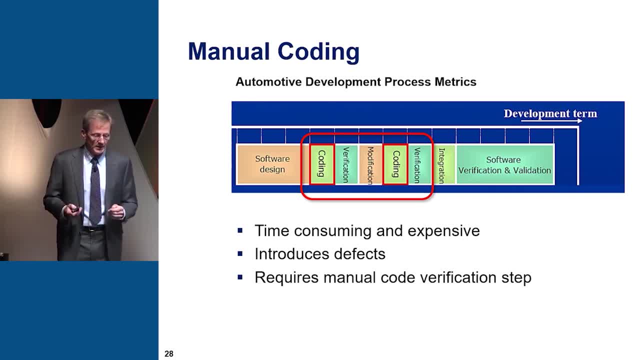 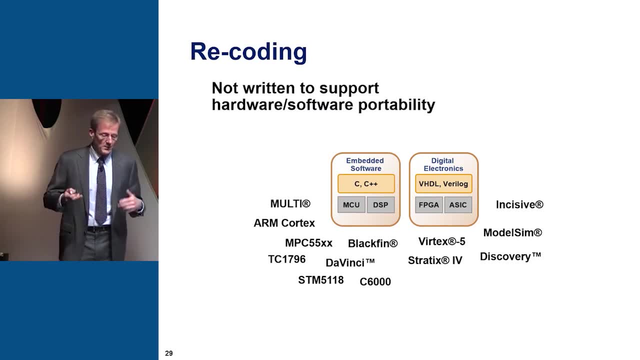 expensive, put in defects And they they were interested in reducing that or perhaps even eliminating that. Another problem was re-coding When you move to a different platform and the design for these different platforms- and there's lots of different hardware platforms that people use. 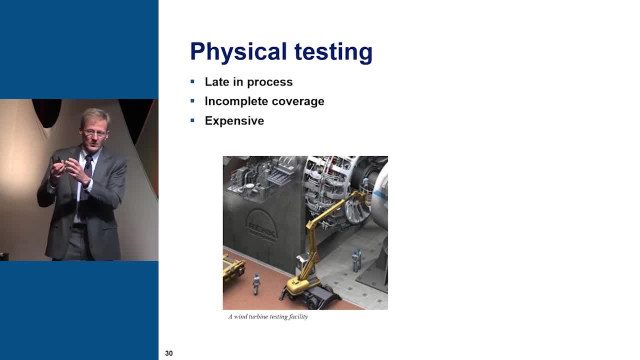 Another problem: physical testing. You have to build these hardware test setups. It happens late in the process. It's very expensive to do. This chart shows the cost to correct bugs and you can see during testing and integration they're 150 times more costly to correct. 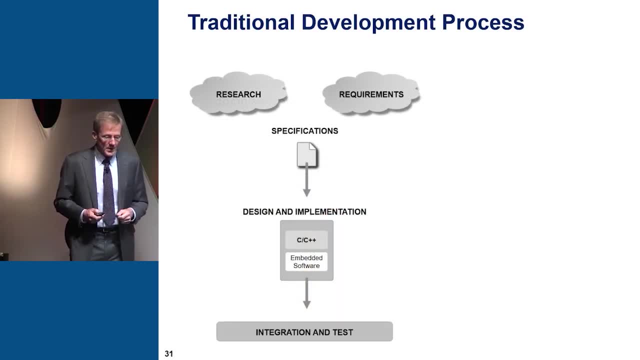 than if you get them earlier. in the design phase There was a traditional development process that industry used. It started with research and requirements, They wrote paper specifications, That was turned into design and implementation and then finally, it was all integrated and tested. 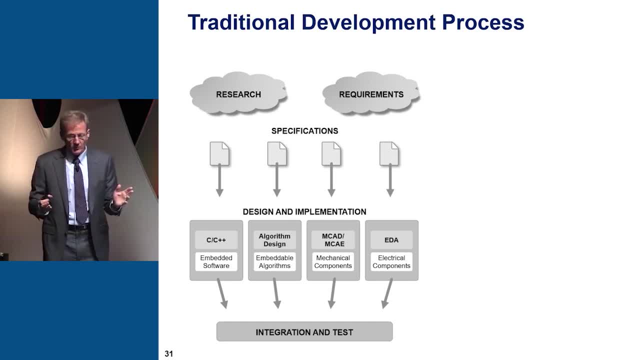 It actually was worse than that, because there were several different groups. often that went into some final system. the mechanical design, the algorithm, the coding, It all went together And problems arose because, in fact, the paper specifications were used to pass these on. 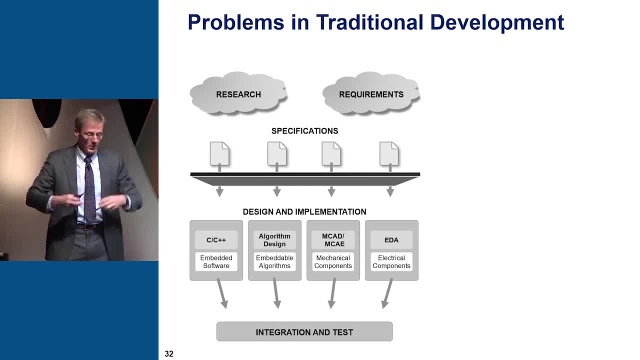 And also there was. So there was And there was a different set of people, But they wrote the specs than they did the coding in the C And there were barriers between the disciplines, And this led to no end of problems. The requirements documents are always difficult to read. 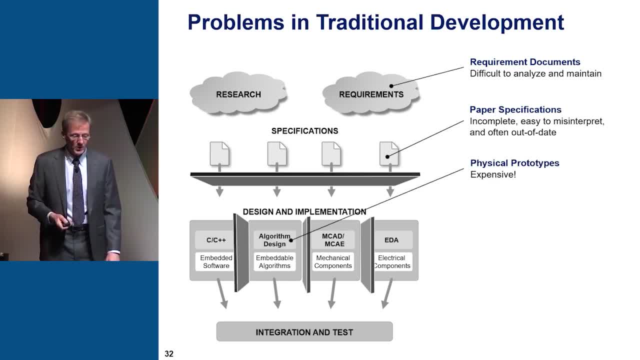 Paper specs are always incomplete, out of date, easy to misinterpret. The physical prototypes were very expensive to do, The manual coding- I already talked about that- And the traditional testing found the design issues late in the game there. So tons of different issues. 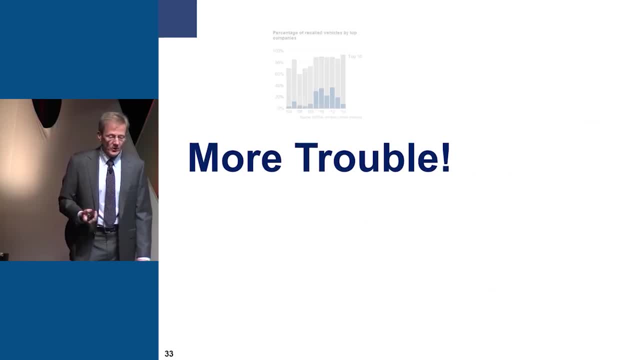 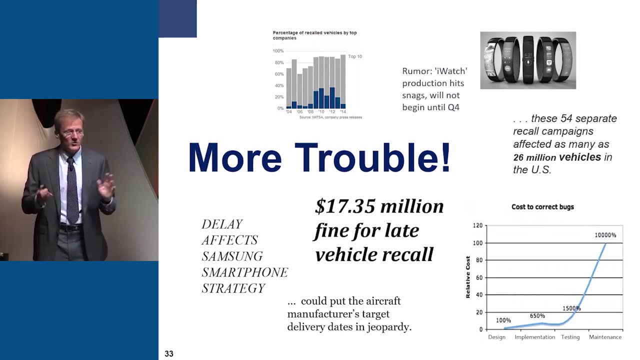 There was more. There was more trouble in chipping some of these systems. There started to be fairly large recalls. If you're increasing the algorithmic complexity and not a software starts to be recalls, And this is You know. industry is starting to be. 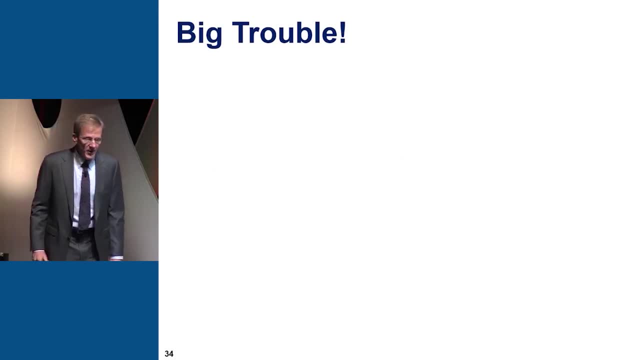 It was very worried about these types of things, And then, finally, there's always the possibility of big trouble And I have a, I have a, Something, A design I want to share with you that I think every control engineer ought to see. 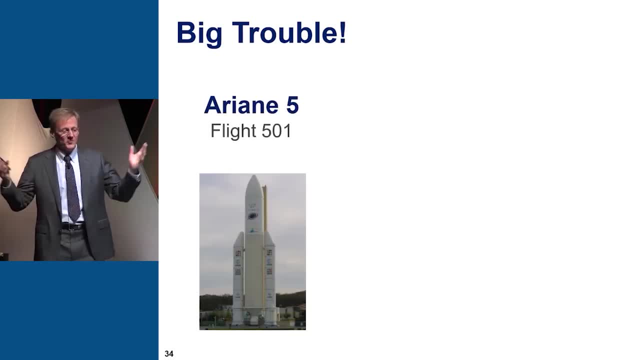 before they go out there and practice. This is sort of the most famous failure in control systems, which is the Maiden fright of the Ariane 5.. How many people have seen this video? Okay, a few. Okay, The Ariane 5 was a new vehicle. 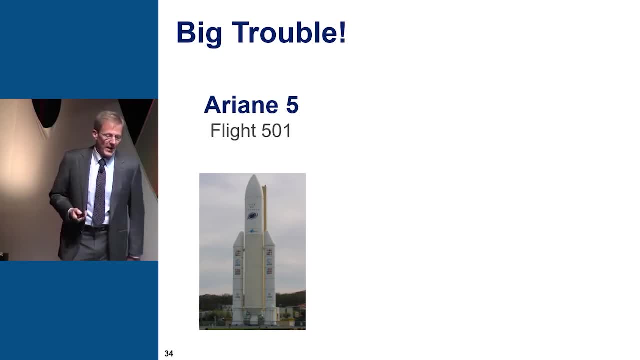 There was an Ariane 4 before it, And this was the first flight of the 5 series, And it Well, I'll tell you what. Let me show you the video of the first flight and then I'll talk about what happened there. 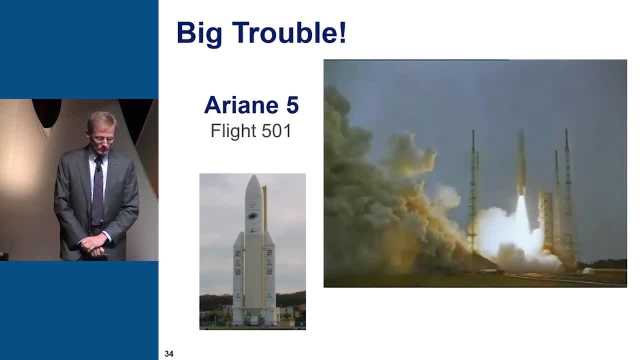 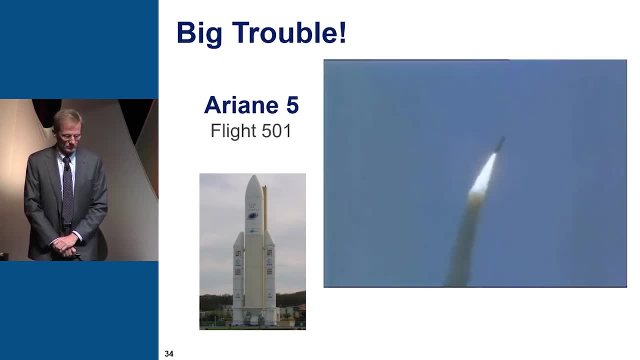 This is about 20 seconds Décollage. You can hear the control room there. It's pretty quiet in here, isn't it? What happened there is they took the controls package, which was hardware and software, from the Ariane 4,. 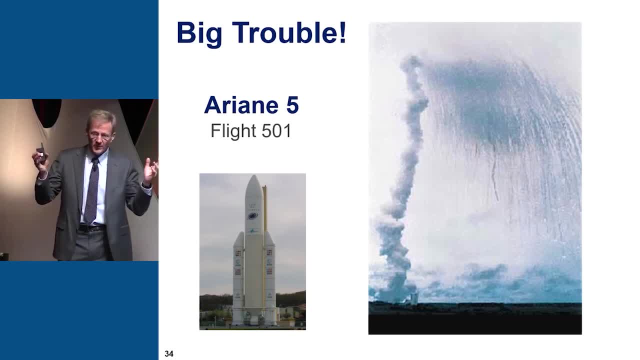 and they slapped it on the Ariane 5.. Okay, Ariane 5 was a bigger launch vehicle, though, But they And And what happened is during the flight there were larger The nozzle gimbals at the bottom. 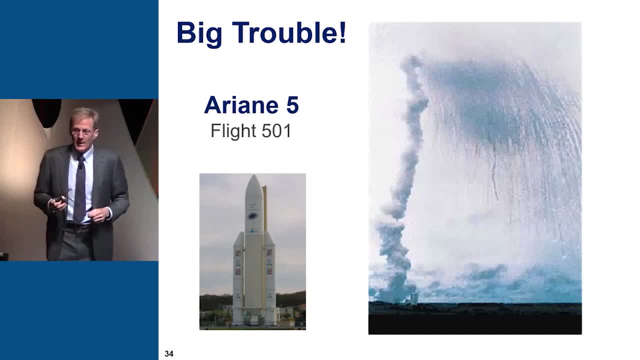 and there were larger extensions because of the bigger system And that caused there to be the larger numbers floating around in the control system and they overflowed the fixed-point registers on the PC, on the computer, which they were designed to hold. Okay, 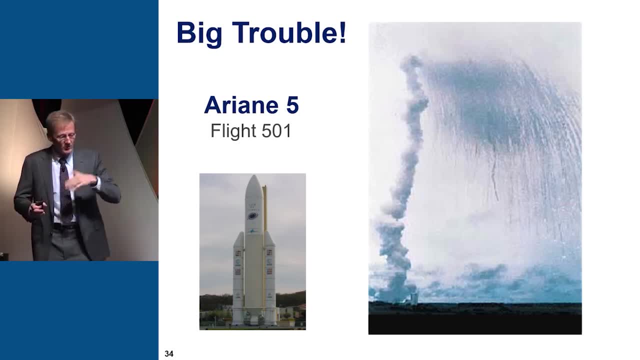 And so So it was a. It was a controls failure, It had to do with an overflow And really what it was a failure is the picture I showed you before in the process. If there had been a process that could have found this in testing. 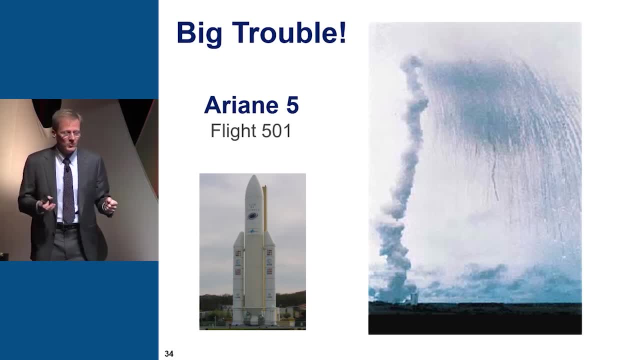 it's just too complicated to test all these parts in all the right ways with the right prototypes and all that, and they just couldn't get all that stuff organized. This was about a half-a-million-dollar launch vehicle that was lost here And it's a great example. 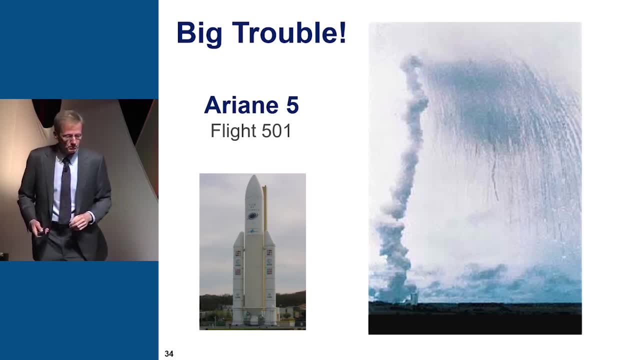 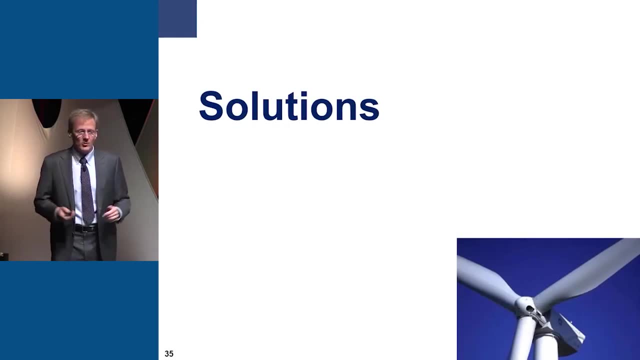 of what you don't want to see. if you're a control engineer, Okay, And so it's a very famous thing, a good thing to You know, for controls people to see Okay Solutions. So solutions started to arise to this. 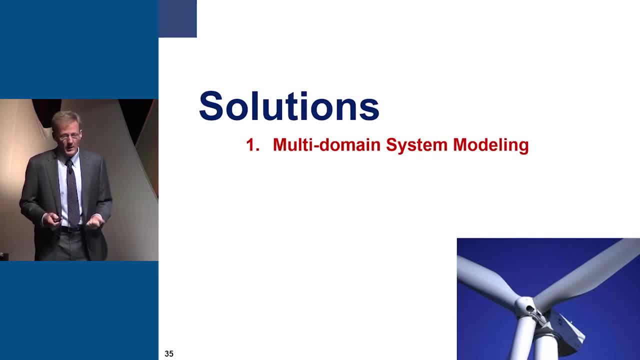 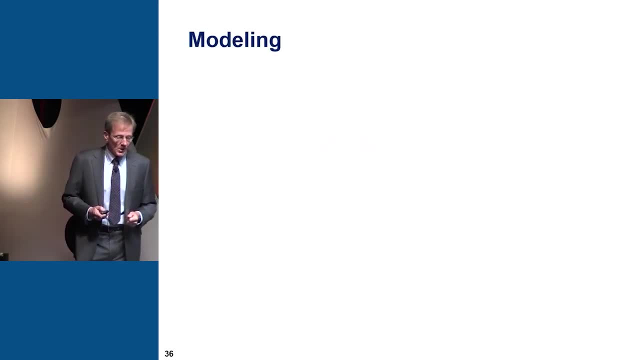 And mainly there's two elements to the solutions. The first one is multitasking The main system, modeling to help solve industry's problems. here Let me talk about what this is. So modeling: it's not surprising that modeling would be a way to help out of these things. 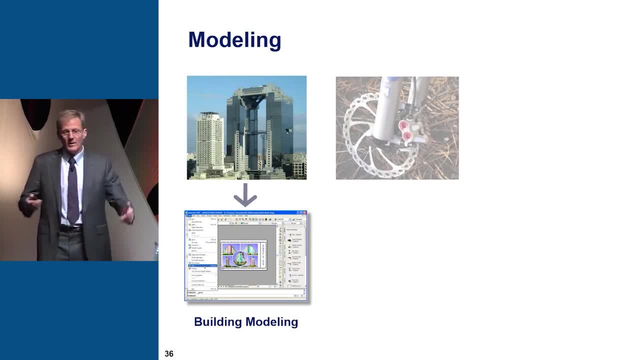 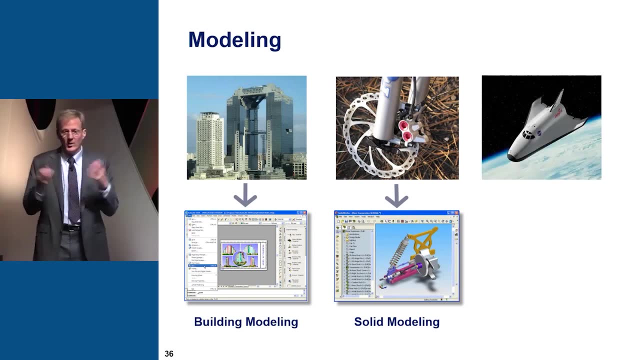 After all, you know, if you look at building buildings, there are building modeling systems. If you try to go build a bicycle braking system, there's obviously solid modeling systems there. So it makes a ton of sense that if you're trying to build a system, 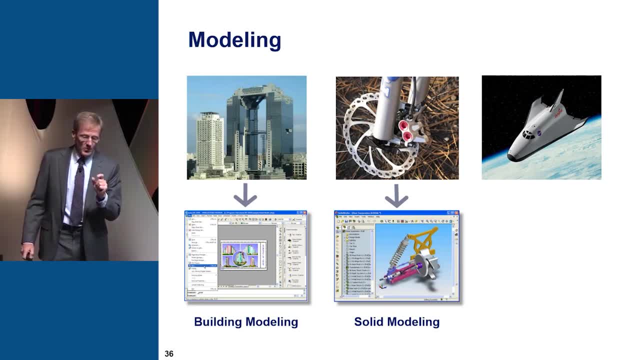 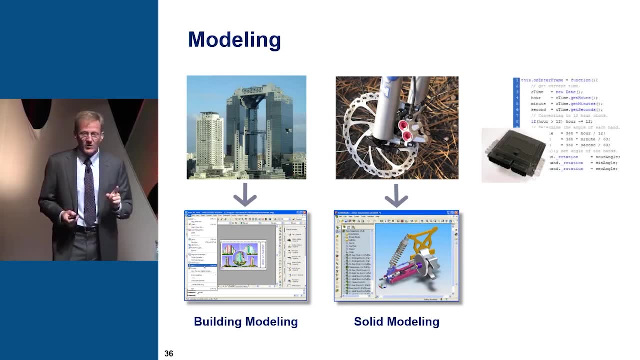 that there be system modeling. Now, to have system modeling, it's important to be able to model the object being controlled, the plant, But what's a little less obvious is you also need to model the software and to model the hardware as part of that. 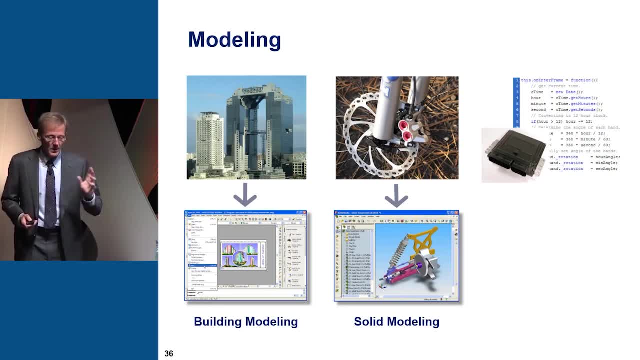 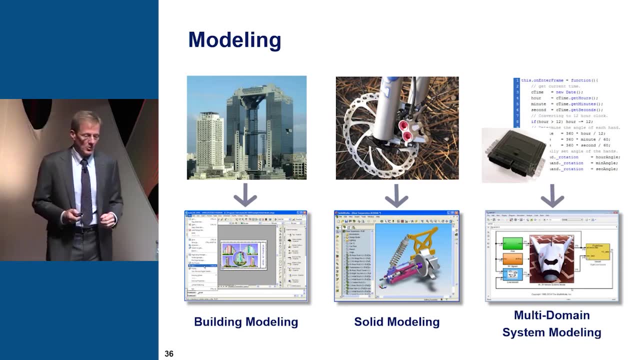 if you want to model a complete system, Okay, This is one of the key elements of this, And so if you could do that, then you've got multi-domain system modeling that can capture all elements of the system that you're creating. The roots of this came in fact. 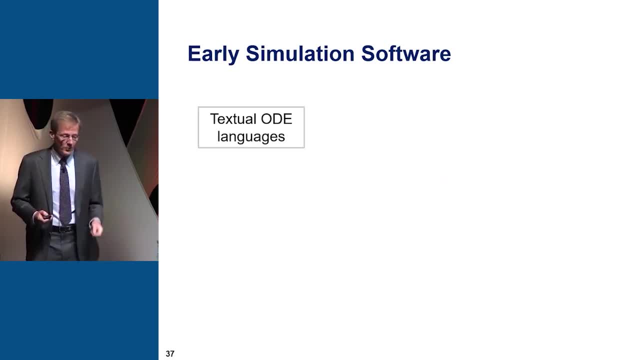 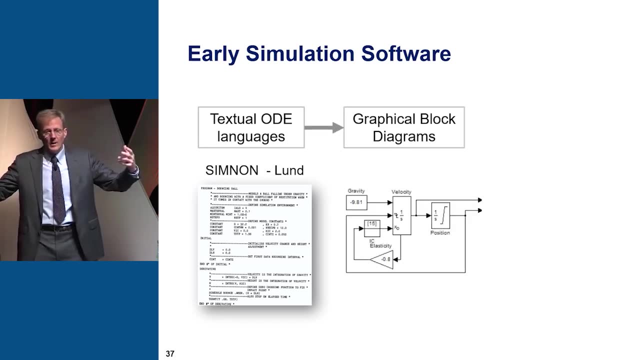 from education, from academia. Some of the earliest simulations software that I used were textual ODE languages. I used Simnon from Lund University When computers developed graphical capability. graphical block diagrams emerged and were used for simulation. But really what was needed to solve industry's problem? 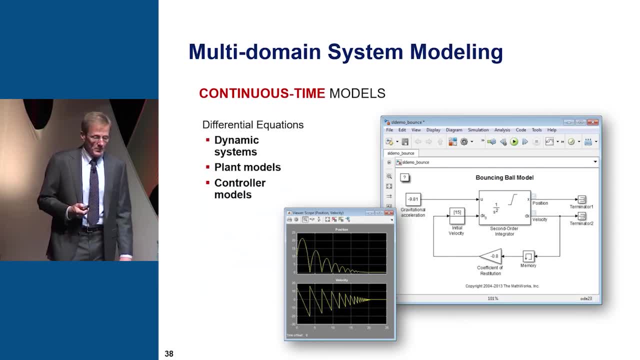 was a multi-domain system modeling package. Now let me talk about what I mean by that. By multi-domain, I think there's like seven domains here Certainly needed to handle continuous time models. you know, for plant and controller modeling You need to handle continuous time models. 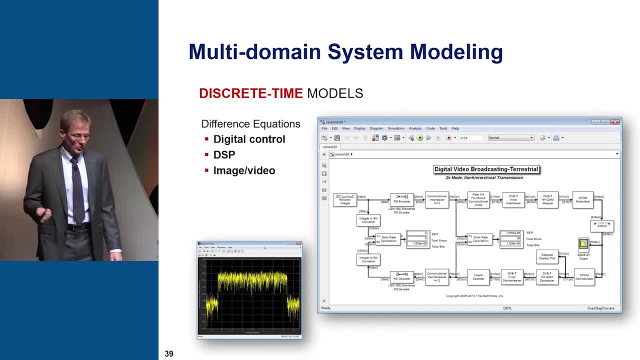 dynamic systems. You need discrete time models so you can do digital control Also. it's also helpful for people doing DSP, signal processing and image processing. You know image is just a matrix and so there's image applications you can do. 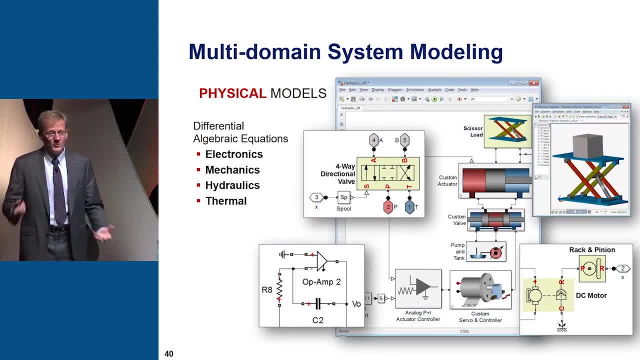 with this type of modeling. Physical models are important if you want to model the aircraft or the hydraulics or the landing gear or whatever you're doing, And the basic domains there are electronics, mechanics, hydraulics and thermal- On a block diagram. 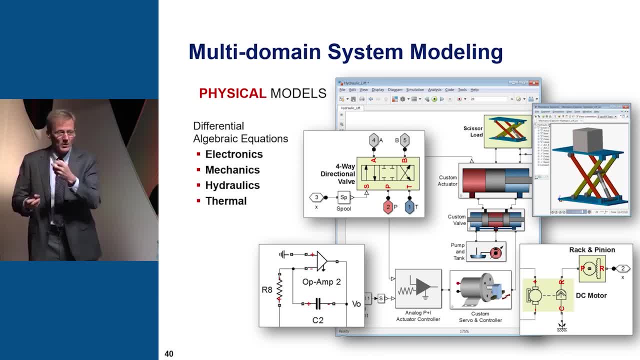 these are differential algebraic equations. You know the lines are bidirectional, you know, with a circuit and a voltage or current or something like that, rather than just the flow diagram the control system has. Now here's where it comes to the software. 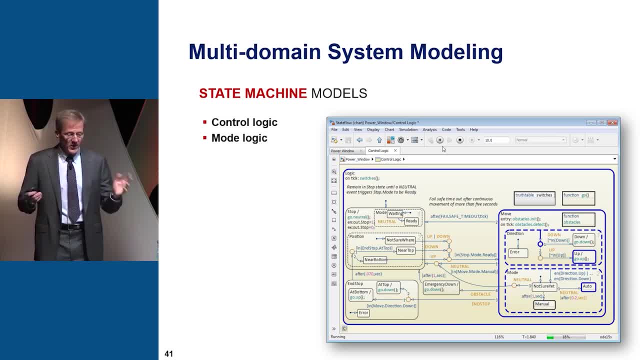 Another important aspect to be able to model is to handle state machines, And state machines are things like: you know, the- I don't know the windshield wiper controls your window on your car. They have different modes that you have to go through. 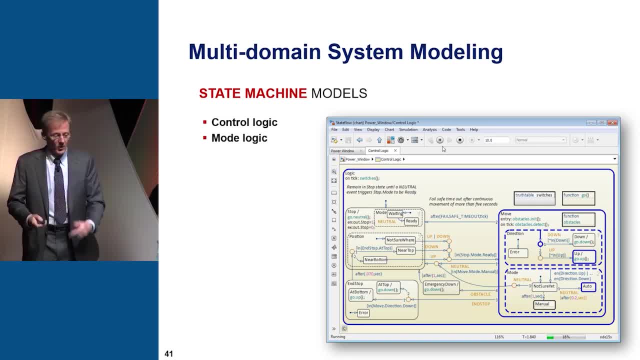 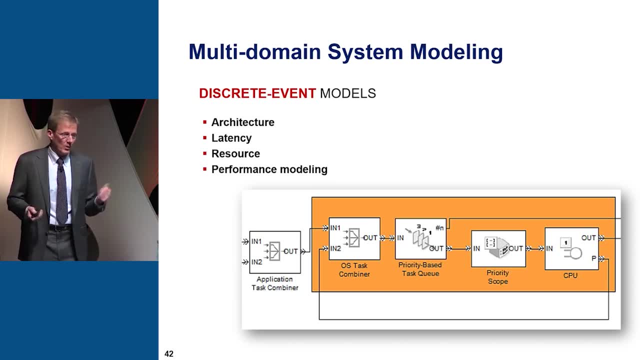 And that's very common, obviously in control systems, And it's also how software is written, And if you want to model software, that's required Also. you know you can model software. There's also discrete event models, Queues. servers are important in terms. 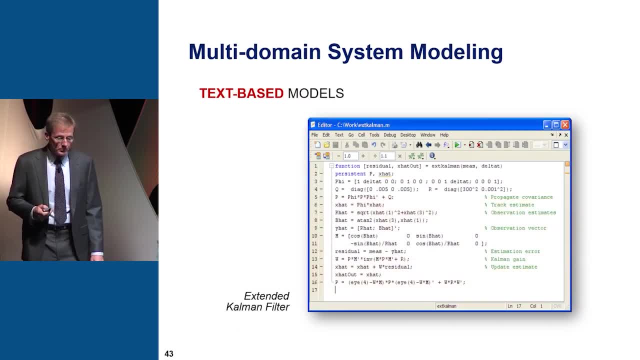 of modeling- computer systems, performance modeling and things like that. And then, finally, text-based models are still important. You know, despite the fact that graphical modeling is a great way to go, there are some things that just don't look good if you try. 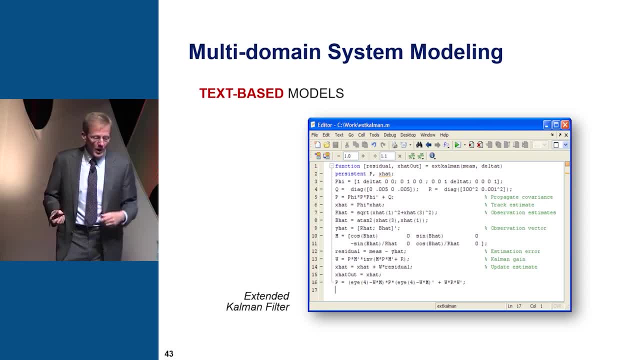 to wire them all up. You know, this 11 line, this dozen or so lines, is an extended column and filter And this is just the right way to write this. You know, if you try to do this with a wiring diagram, 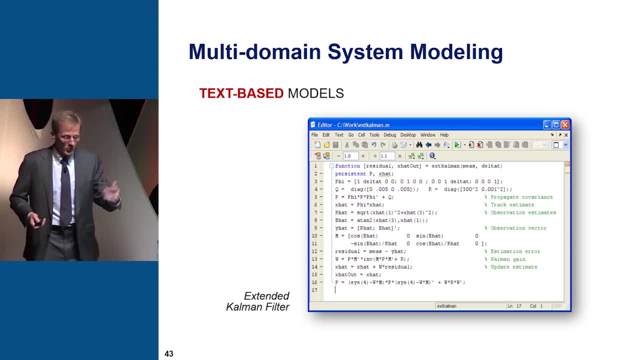 it's going to look like spaghetti and you won't know what's going on. But this is a straightforward common filter, extended common filter here- So textual- is an important part of any multi-domain system modeling. I'd like to give you an example here of a multi-domain model. 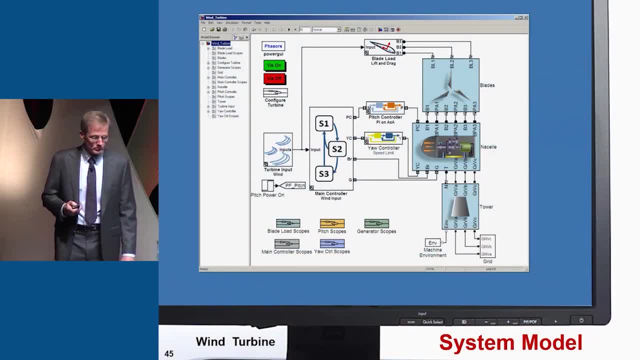 I'm going to choose a wind turbine to show you. Okay, here's the top level diagram, multi-domain model, a system model of a wind turbine. This is the model for the blades. This is the nacelle, That's the unit at the top of the that spins around. 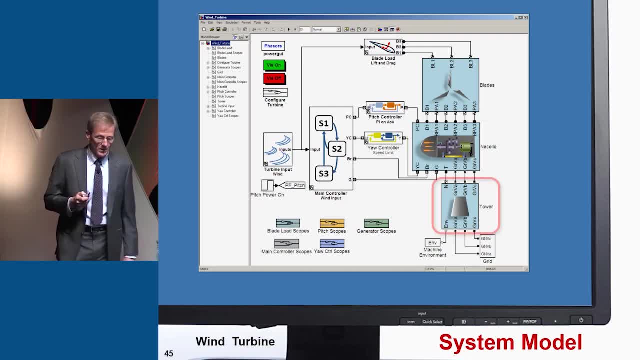 That houses the gears and the rotor for the fan. There's a tower model. There's a model for the grid. in this case, This is the pitch controller for the blades on the turbine. This is the yaw controller. It controls the position the housing is porting. 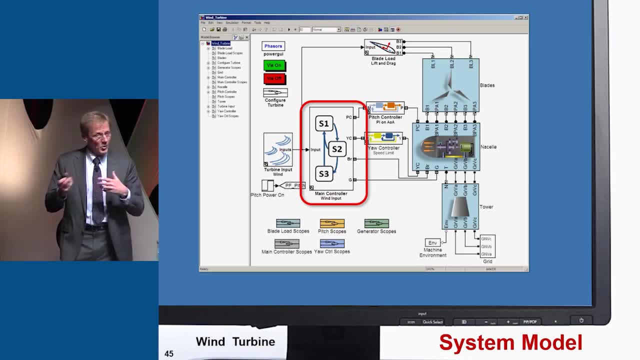 Here's the main controller. This is going to have multiple modes, because there's going to be some modes we need to take the windmill through And then, finally, we need a wind input in order to drive this simulation and test it a bit. 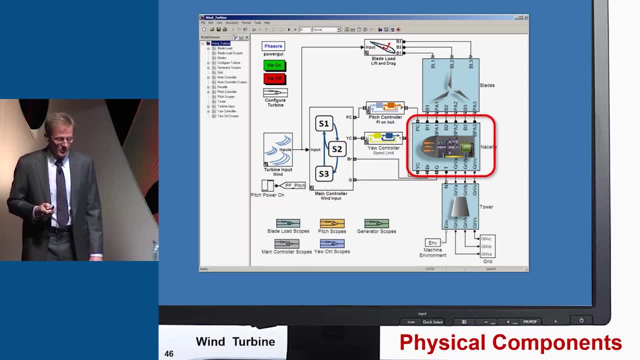 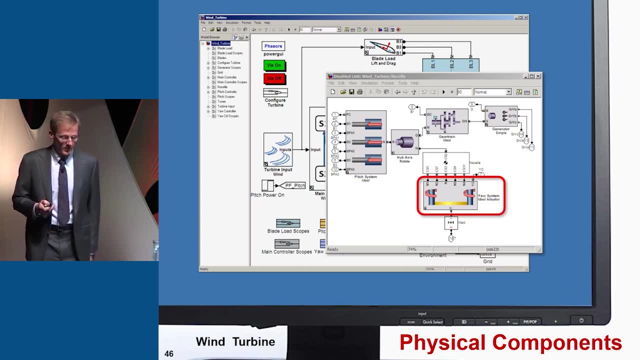 Okay, let's look inside the nacelle and see what we see. Okay, in here we have a gear train model, We have a generator and we have an actuator model for the yaw system. We can look at the wind input model. 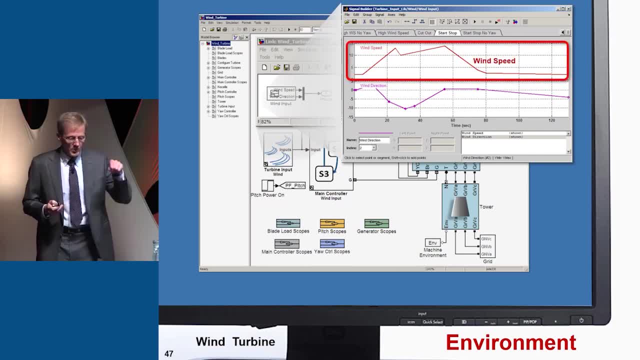 This is going to be fairly simple. for this example, The wind speed- we're simply going to put in a piecewise set of winds, So it's going to start at zero. The wind is going to ramp up to 10 or 12 and fluctuate. 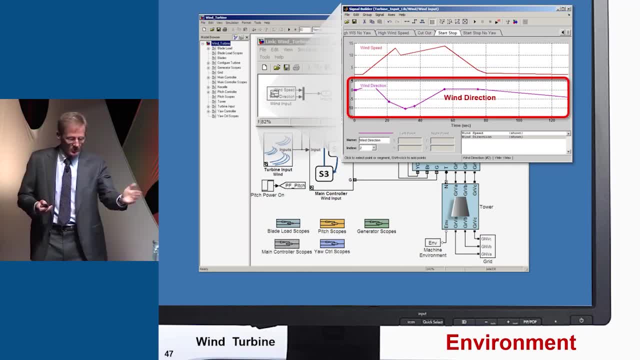 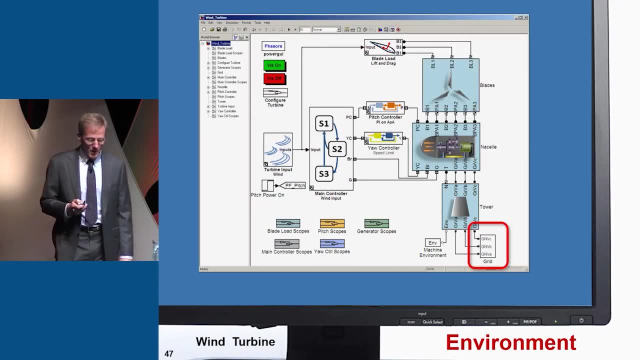 and then it's going to drop down to zero again, And then the wind is going to change direction. It's going to start at zero, It's going to move around over the course of this simulation that we'll do, And then down here there's a grid model. 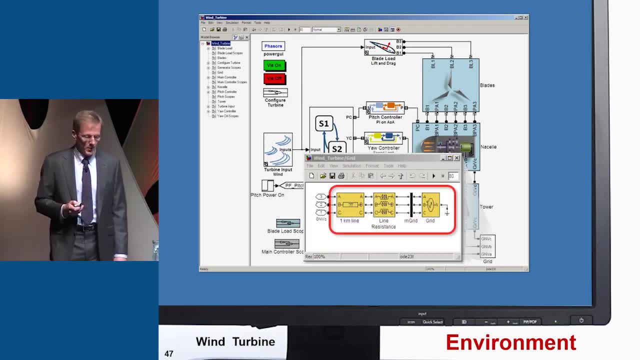 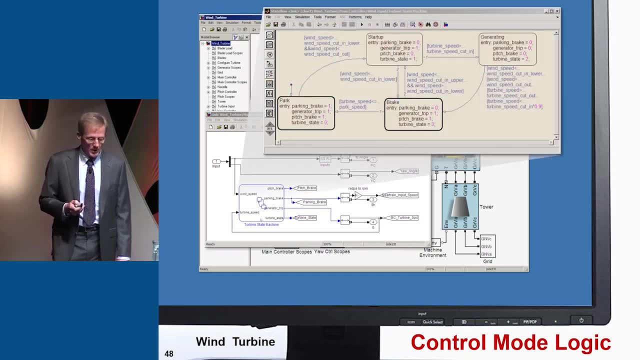 This is a transmission line and resistance there as part of the model. Okay, Okay, here's the mode controller. In here we have a finite state machine model and it's got four states. This is the park state, sitting there waiting for the wind to start. 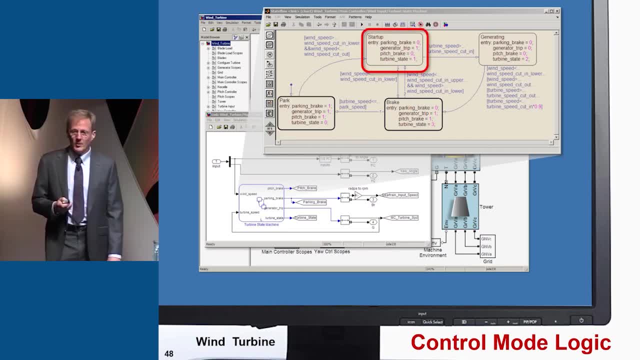 The wind starts to pick up. At some point it becomes strong enough. It goes into a startup mode, which is one that's trying to bring it up to speed And that's going to try to get it up to 15 RPM, which is the speed it likes to run at. 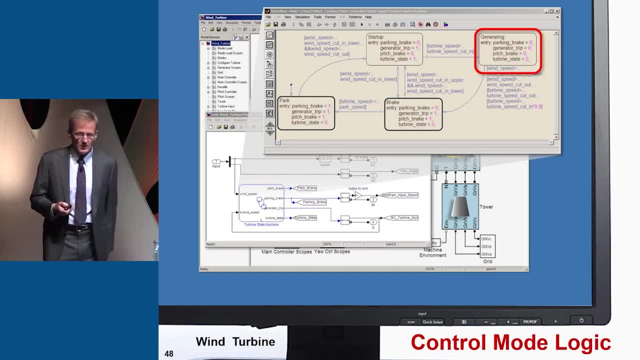 Here's a generating mode. That's when you've reached that and you're just operating and maintaining a regulator. And then, finally, there's a breaking mode. The wind gets too strong or it dies. You need to break it and slow the whole thing down. 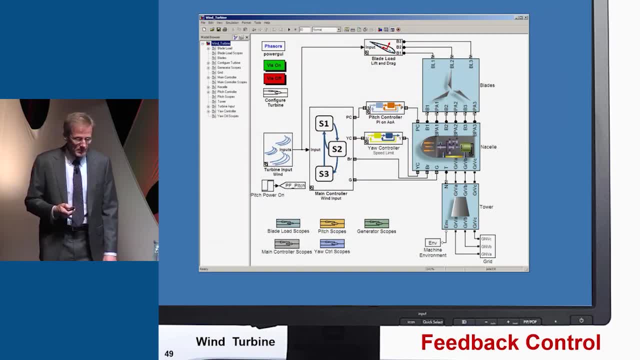 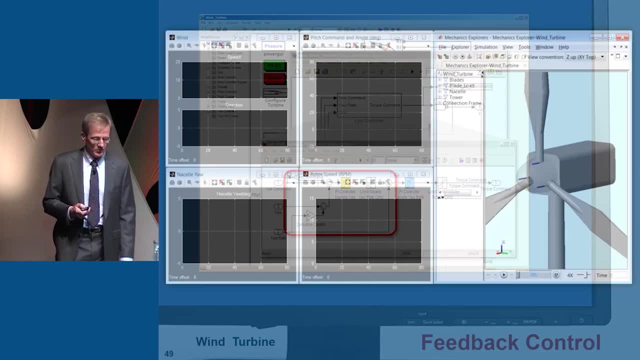 And so there's going to be different control behaviors in each of those. And then here's the awe controller. We can look inside that. In this case it's just a simple PID controller in this case, So this is a tremendously multimode model. 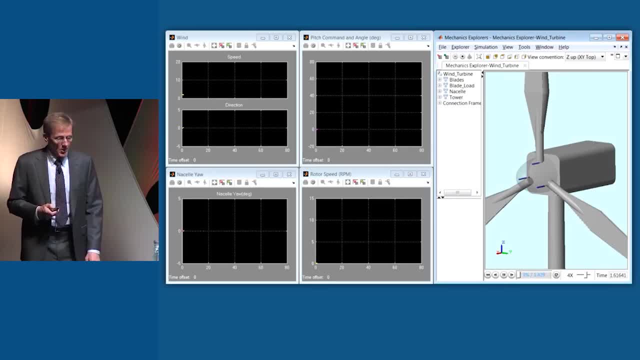 There's a lot of things that we can do. There's a lot of things that we can do. There's a lot going on here in this. Okay, We're going to run the simulation now. If you look in the upper left corner here, you'll see the upper. 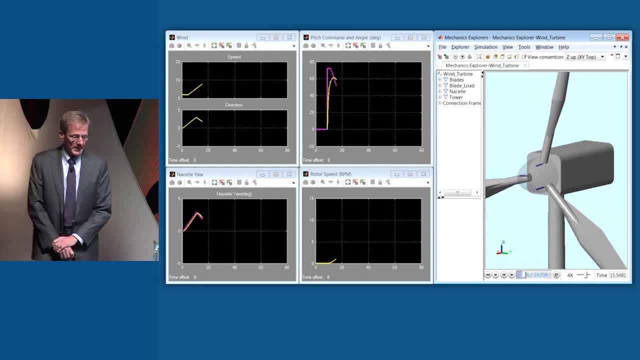 chart there is wind speed And you can see the wind is picking up there. The chart right below that is the wind direction. You can see that's fluctuating around. If you look in the bottom left that's the direction of the nacelle so it pivoted to point into the wind. 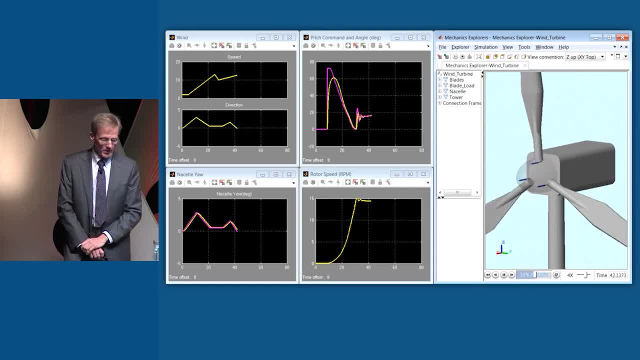 On the lower right you can see the speed of the turbine and you can see it ramped up to around 15 RPM And it's now being regulated at that as the wind is changing direction and changing speed. In the top right you can see really the control input. 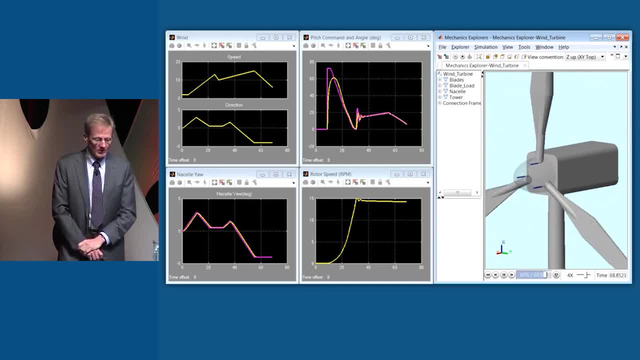 which is the pitch of the blades, and then the pitch that's achieved. So there's the command and what's achieved there, And you can see that regulating the speed. Okay, The wind is starting to drop and at some point it can't hold on, and it has. 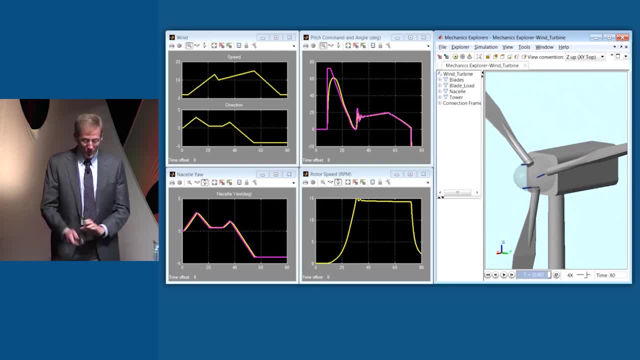 to just feather the blades and break and come back down to a stop. So tremendous amount of stuff going on there. This may be the most multimode simulation you know a lot of you guys have seen here. I mean, you know people don't normally build models. 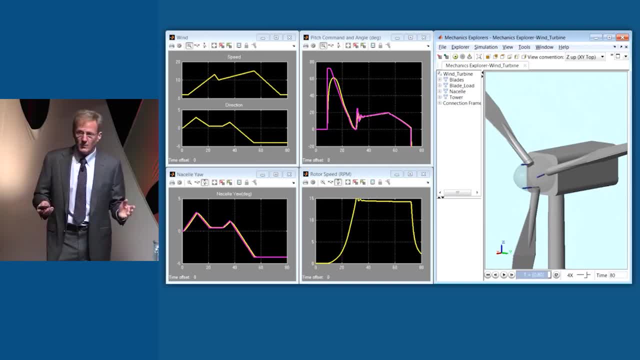 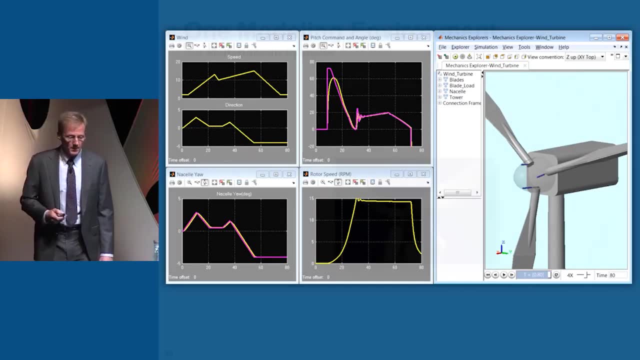 this complex that have every single type of mode in it, But this is often. people focus on a subsystem, But this is an example of a highly multimode, multi-domain system. Okay, So the goal of this is to have a single modeling environment. 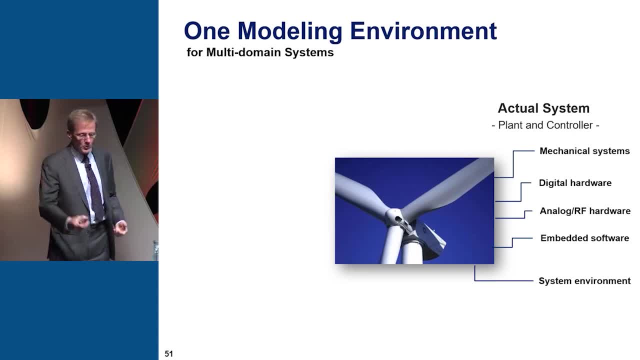 that can model the full system: The plant controller, the mechanical digital hardware- analog RF, if you need it- the embedded software, and then the environment, the wind and things like that, And and, if you can, then you've got a model system that models the whole thing. 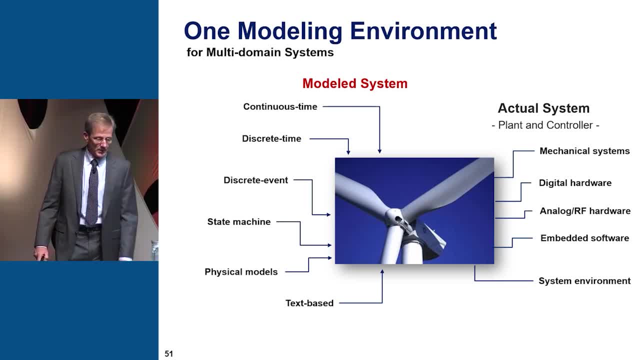 And it includes the various domains that I mentioned At MathWorks. this is the name of the different software packages that we've developed. We have a team of about 500 people that's working on development of this model-based design. This is the life's work of a lot of people. 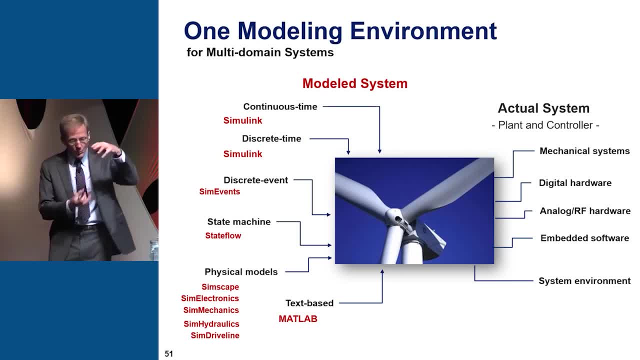 over the last 20 years to build this stuff, To build this one environment that can work all these modes together. It's extremely complex how you can do all these things. There's lots of instances of each of these different modes that are in the wild. 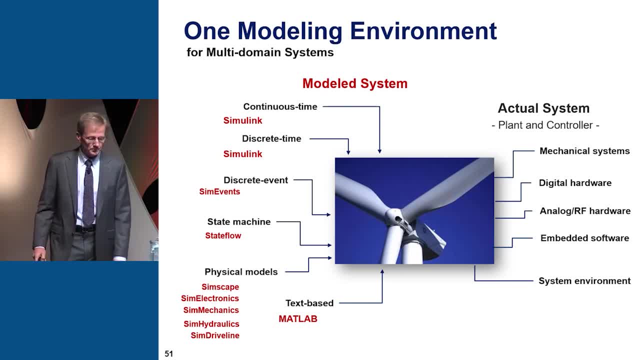 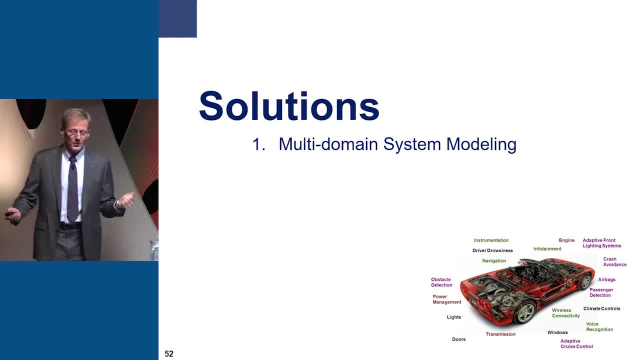 out there in different forms, But getting them all worked together is quite, quite challenging. Okay, So this is one part of the the solution to help industry towards building these complex, complex systems. The other part is a process called model-based design. 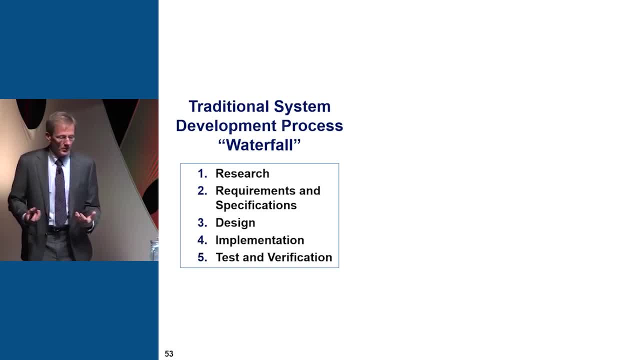 And industry prior to that had used a traditional development process. that's often called a waterfall. You know, there's some research that results in requirements and specs design. write the code, then test it And and it was fairly once through. 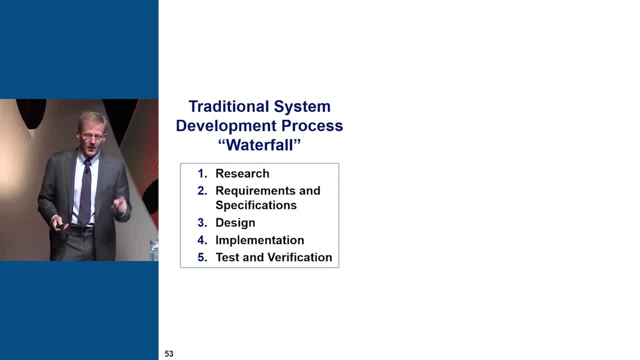 You know you had a a schedule over a year or two year period where you'd work through that. Obviously you'd have to do little loops in there, But generally it it went through that phase. Model-based design changes that process quite dramatically. 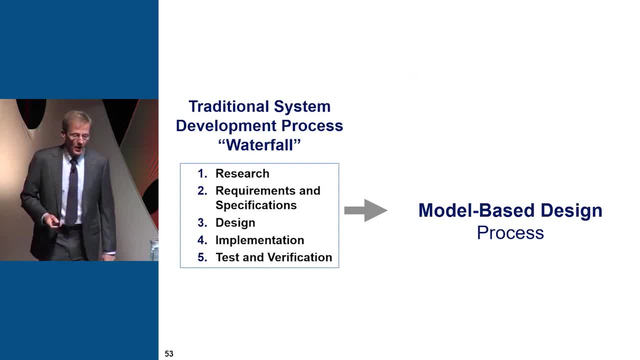 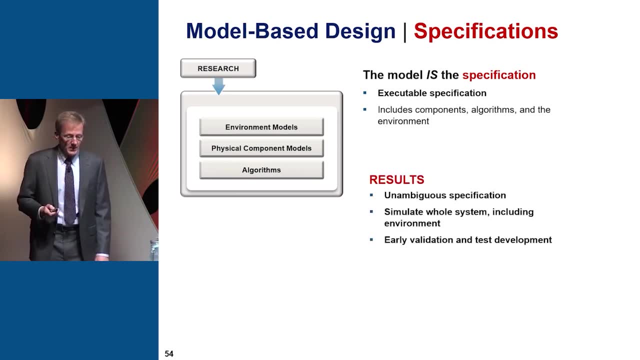 into a different approach And in model-based design, you start with specifications, But rather than writing paper, you you create a model. The model is the specification, And the beauty of that is that it is unambiguous. Okay, Because it either runs or it doesn't. 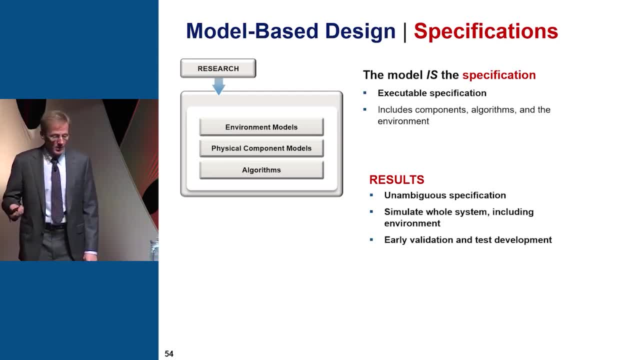 Okay, You can't have gaps in that And it's a, so it's executable. And you also simulate the, its whole system, And you start testing it. right then. That's the key thing: Don't wait till you've you've integrated it and written the code. 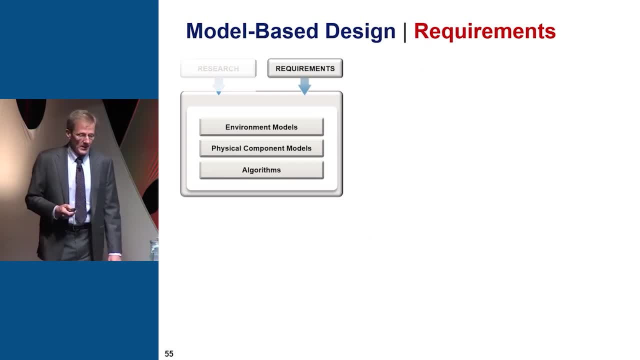 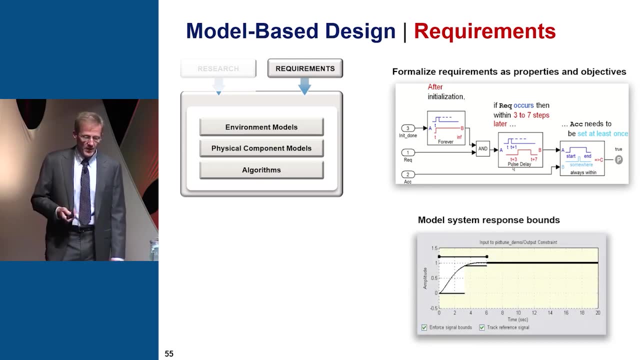 You start testing right away, validating and so forth. The next phase, requirements, are done in software. You create properties and objectives that that define the requirements, And then you can put system bounds on the outputs if you want to restrict it as part of the requirements. 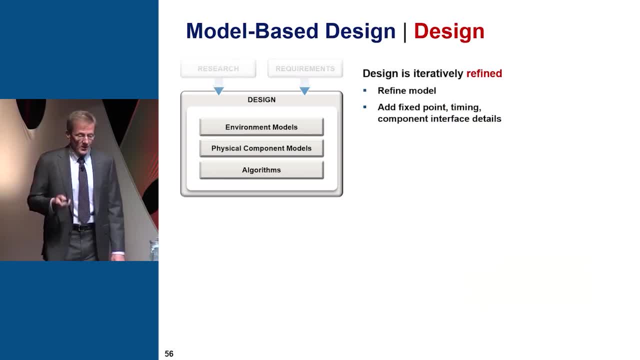 So the requirements are built in software, again unambiguous. The design then is refined iteratively. And this is part of the power of model-based design is you could do a lot of iterations in the models. It's very hard to do that in C code or once you've already. you know. 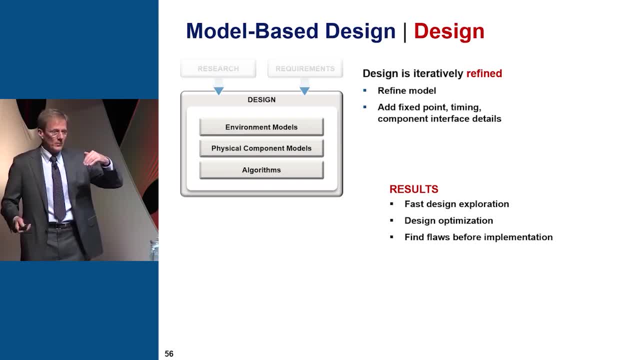 are testing it on a piece of hardware And at this point you can add fixed point effects or timing or component interfaces or or real physical things that you have to do to turn this into a design. The result of this phase is an opportunity to do, to explore many alternatives. 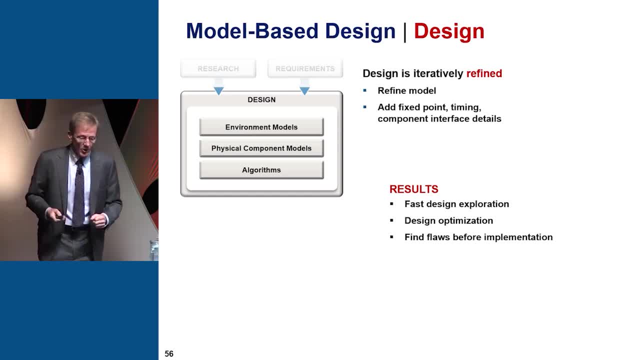 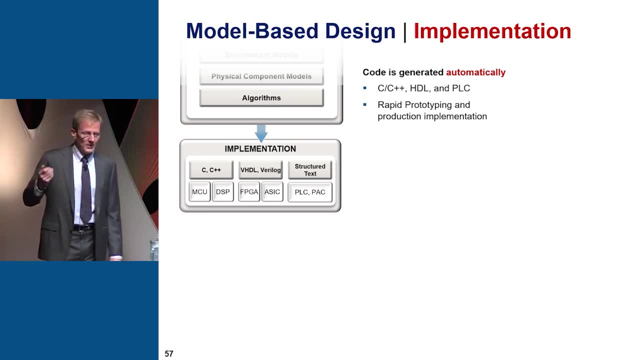 And really do a lot more innovation. You can try a lot of different fundamental ideas And also find the flaws before you implement them. The implementation stage- and this is one of the more value, high value generating sections- the code is generated automatically. 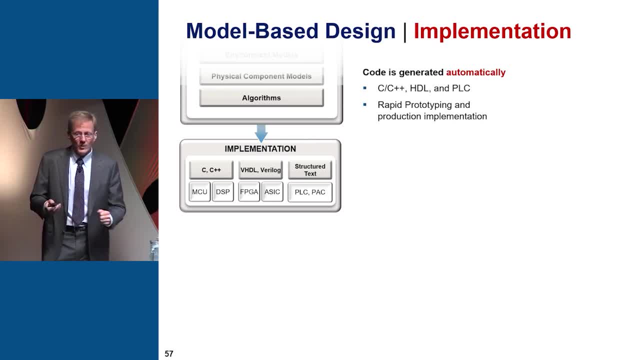 See so and and that can save you know if you write. to write 50,000 lines of code or 100,000 lines of code, extremely expensive, And so it. it eliminates the hand coding, eliminates the hand coding errors. 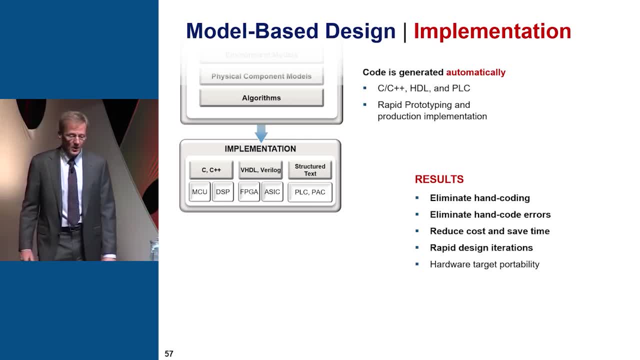 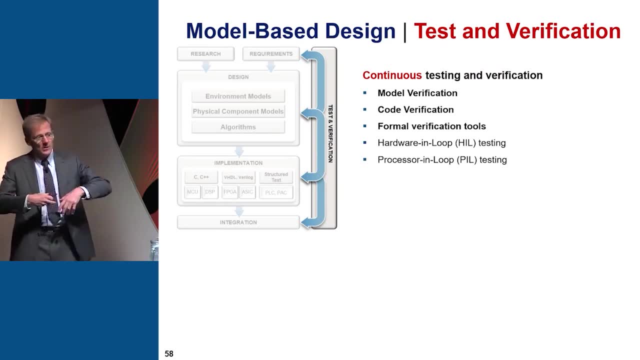 And it is a huge impact. This is one of the reasons industry really likes this, as it largely eliminates this phase And and test and verification no longer happens at the end. It happens continuously through the process And and it it. it saves money because you don't have to have so many physical prototypes. 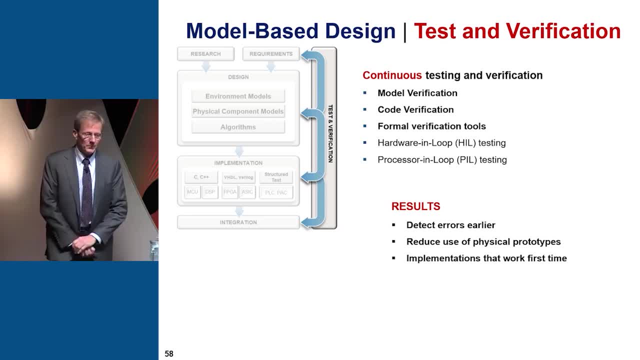 to detect errors here and so forth. I remember years ago when I visited an automotive test track in in Germany where they'd used model based design to design some active suspension software. And we got out there and was talking with one of the technicians- you know, old grizzled. 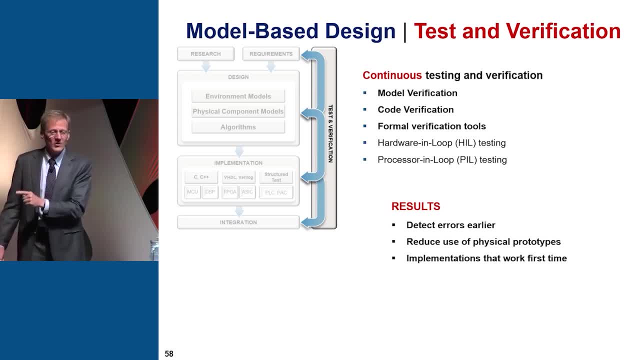 technician, technician, And he looked at me and he said: you know, this team is the first team that has ever engineering That have ever come down here and their design has worked the first time. You know he'd been there for many years. 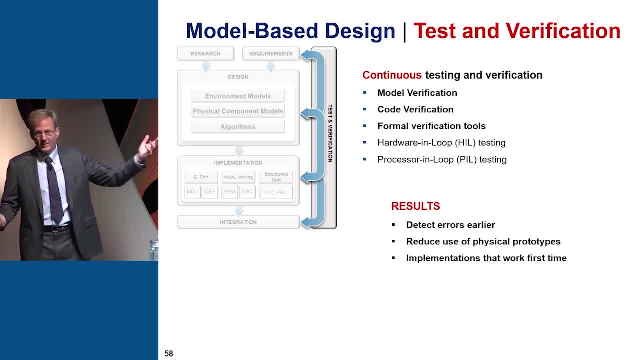 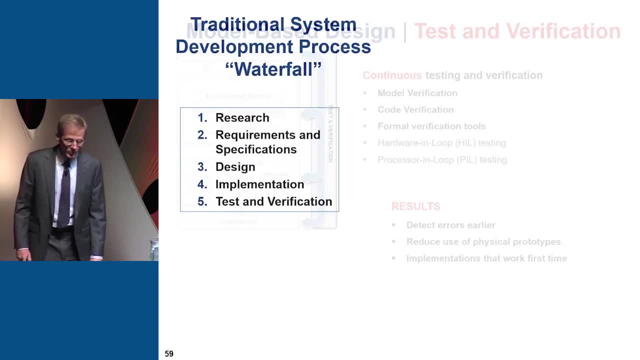 And, of course, why did it work the first time? Well, it's because they they really had simulated in the, in the lab, you know, thousands of times and worked out all those kinks, And so that's what the opportunity is. 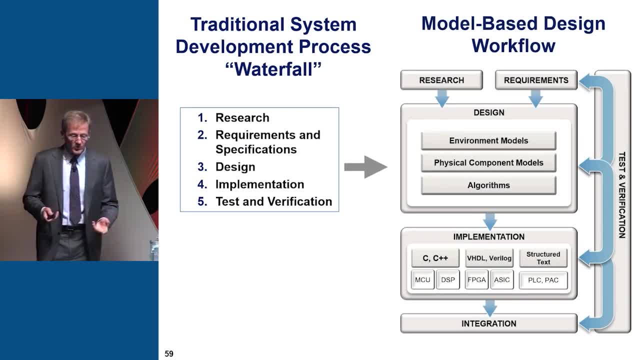 So this waterfall's replaced by this more complex picture. that's iterative. You can, late in the game, put things in and move it through there, And so the the fundamental items here are: the model is the spec. The requirements are part of the model. 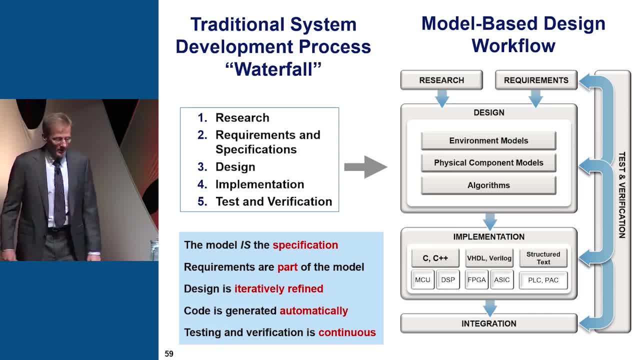 You can iterate a lot on the design. You know you don't have to write the code. This is huge for you guys. You know you, you control, control ideas. The implementation stuff is often things you're not that interested in. 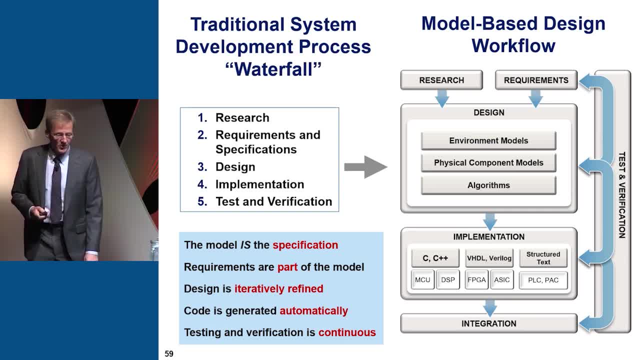 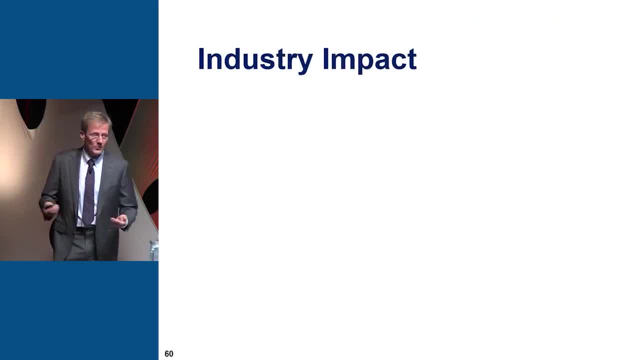 And you can press a button and have that taken care of And the testing and verification happens through there. Okay, So what? what let's? I want to talk now about some of the impact on industry and share some of the successes in industry using this. 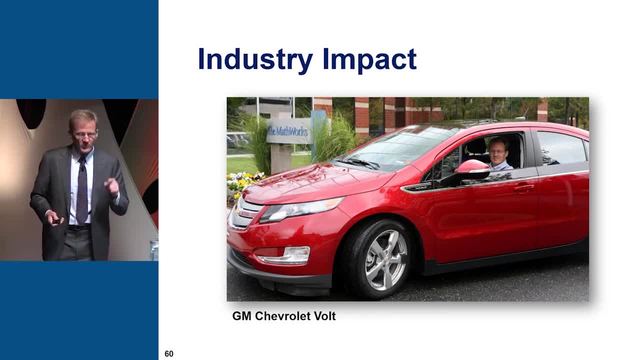 This is a picture of of a Chevy Volt. It's actually me in the Chevy Volt. This is the first Chevy Volt in the state of Massachusetts GM bought, brought an early prototype out to a conference that we had on a student competition and allowed some people to drive it around. 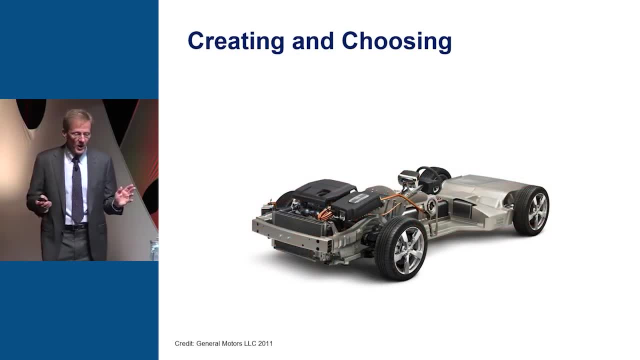 The. this was designed heavily through model-based design. They had a very crash program to design this at GM And oftentimes when there's a crash program, they'll adopt model-based design because there's no other way they could possibly hit the schedules there. 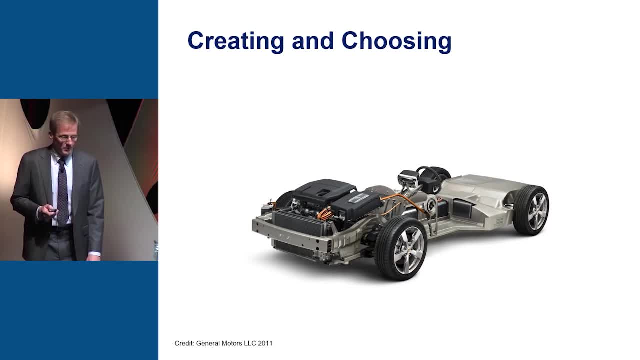 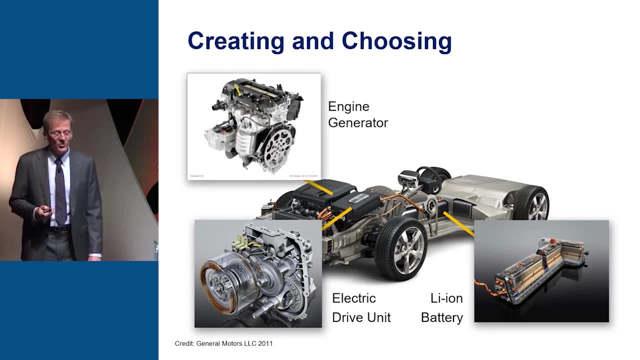 The Chevy Volt. here's a picture of what's inside the Chevy Volt. This is a. this is a electric car. Well, it has an electric drive unit and a battery to power it, But then it has an engine generator. So if you run the battery down, this engine will kick in and generate electricity, and 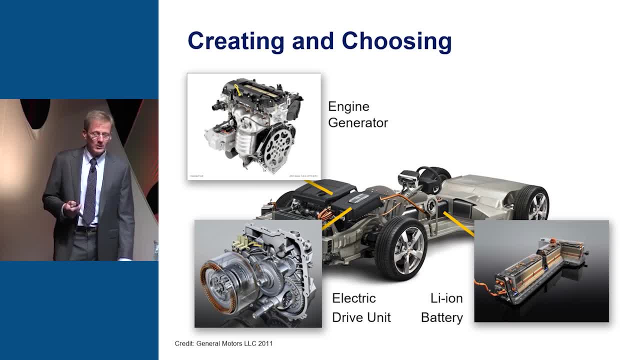 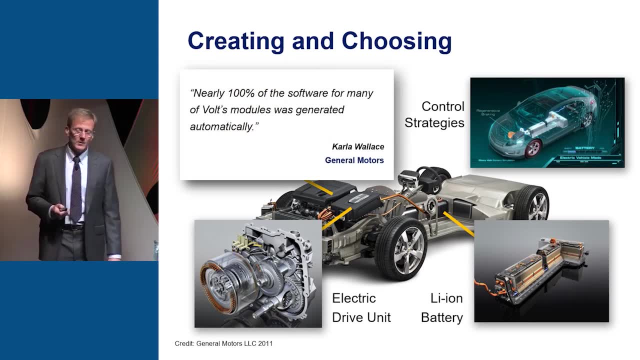 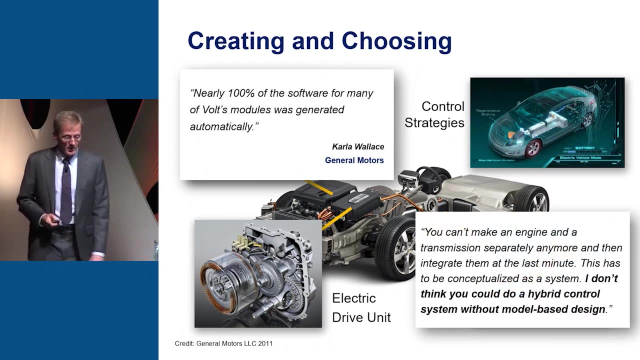 recharge the battery and drive the car, And it was one of the early electric cars that was was released. And then there's control strategies to make these all work. Here's some comments from the people at GM. Nearly 100% of the software for many of the Volt's modules was generated automatically. 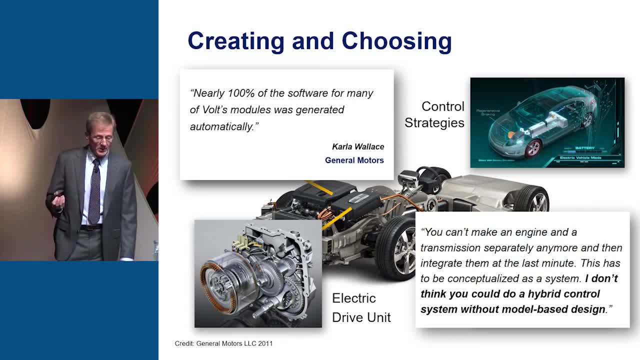 Here's another one. You can't make an engine and a transmission. You can't make a transmission separately anymore and just integrate them at the last minute. It has to be conceptualized as a system, And the comment here is: I don't think you could do a hybrid control system without model-based. 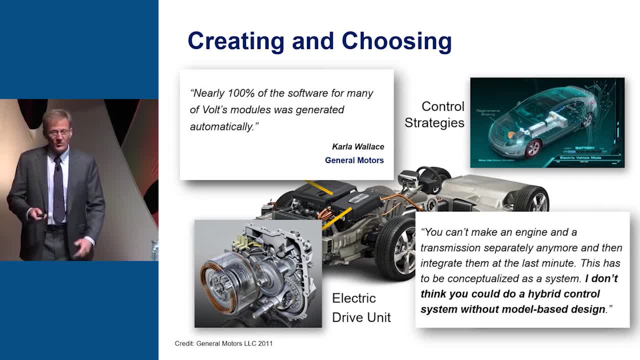 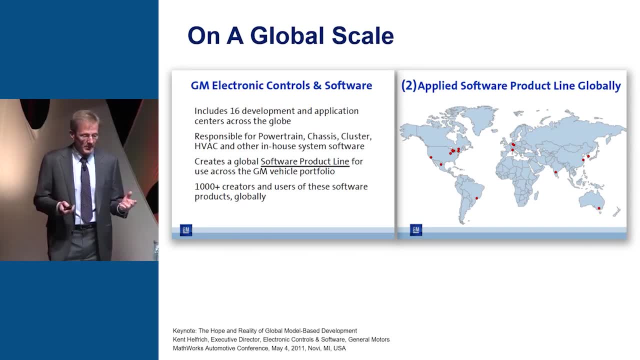 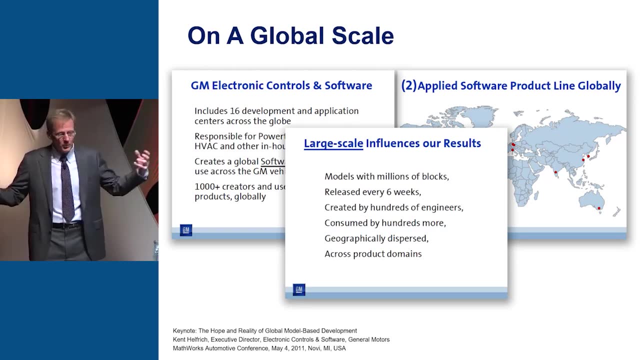 design. GM does this. GM has is using model-based design on a global scale. They have 16 development application centers across the globe that are all doing this. They have models with millions of blocks. They release software every six weeks. People push out their. you know the the algorithms for the various subsystems. 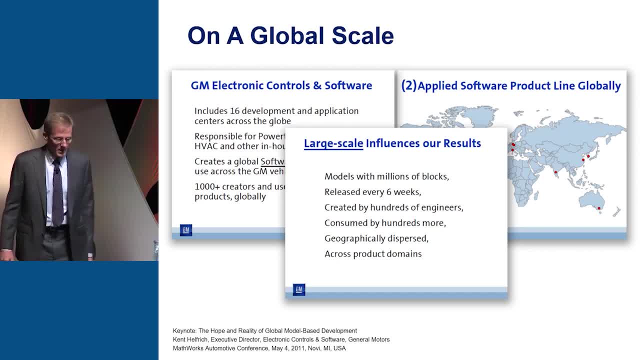 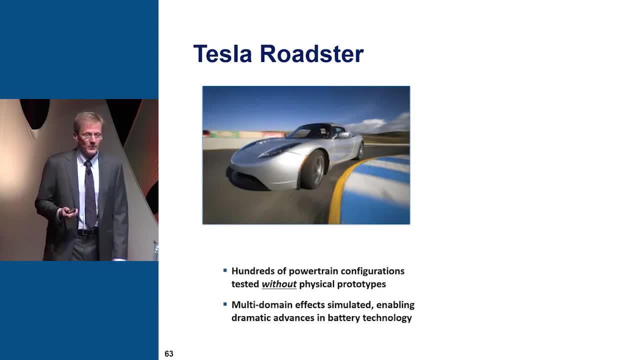 And they get integrated every six weeks for use by everybody. They're created by tons of people and across all product domains. At the other extreme, here's an example of Tesla. Tesla makes an electric car came out fairly recently. They tried hundreds of power train configurations without and they didn't use physical prototypes. 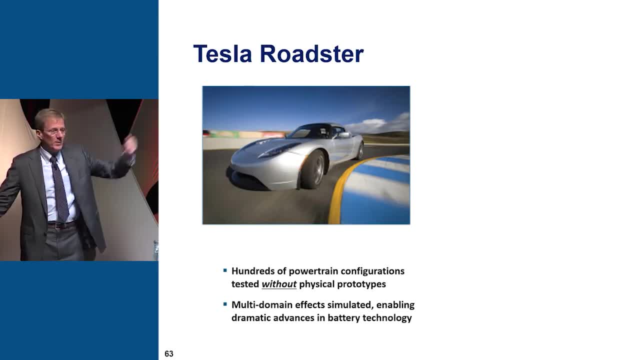 This is a startup. They're exactly the opposite direction of GM, which was a small team of people trying to design a car, And it's unusual. You know it's hard to have a startup in the automotive industry, But they're doing it. 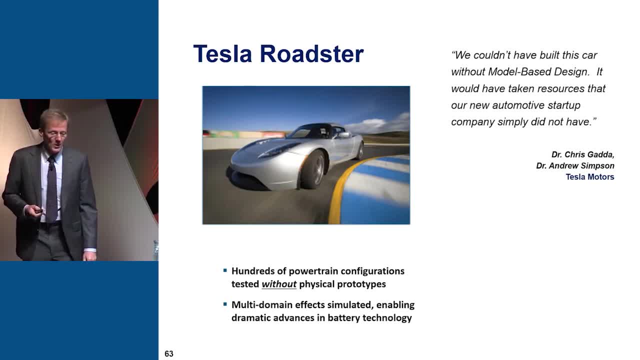 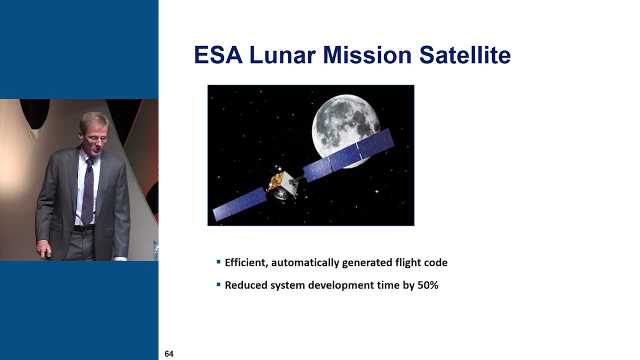 And a comment from engineers there: we couldn't have built this car without model-based design. It would have taken resources that our new automotive startup company simply did not have. This is an example from the European Space Agency, their lunar mission satellite. They generated the flight code. 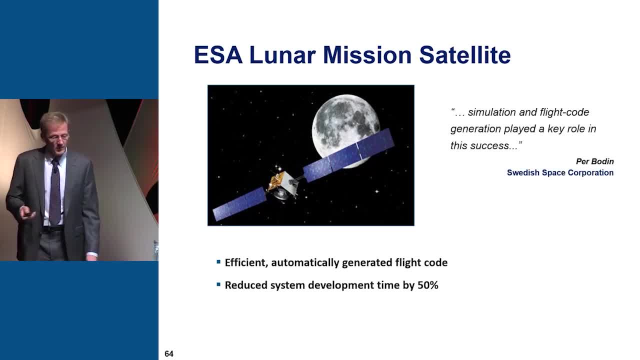 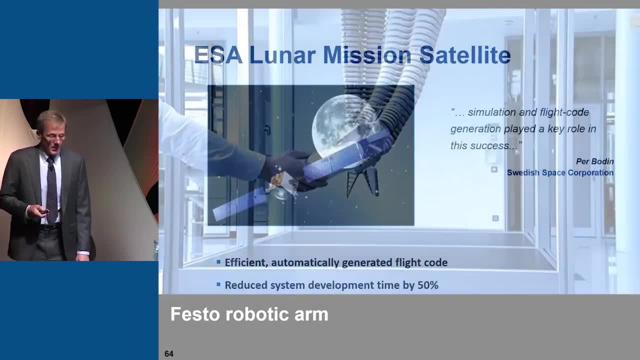 They said that it reduced their system development time by 50%. Comments here on the simulation and flight code generation played a key role in the success. The here's an example That I like. It's from Festo. Festo, I understand, had a talk earlier this week. 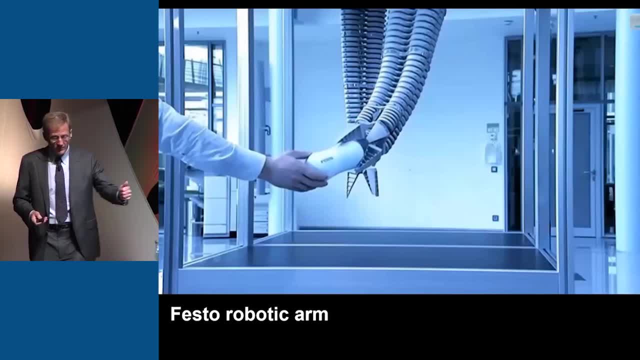 I wasn't able to attend it, But I'm a real fan of what the Festo company is doing: Lots of very innovative stuff. This is a pneumatic robotic arm that they've designed. I don't know if they showed videos earlier this week. 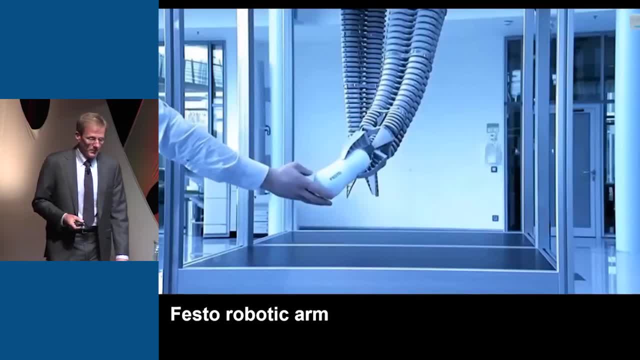 I think they focused more on their flying machines, But this was all done with model-based design to create this, the prototype that you're seeing here Now. what's interesting about this is that it's a prototype. It's a prototype, It's a prototype. 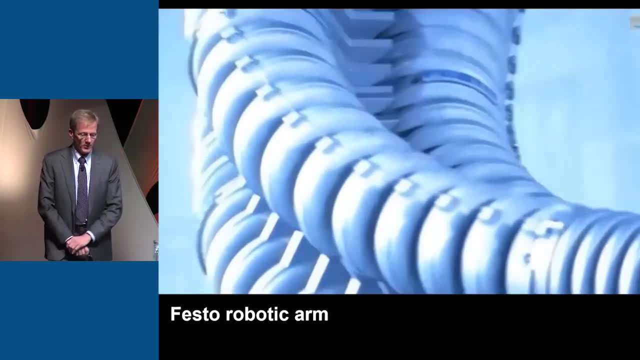 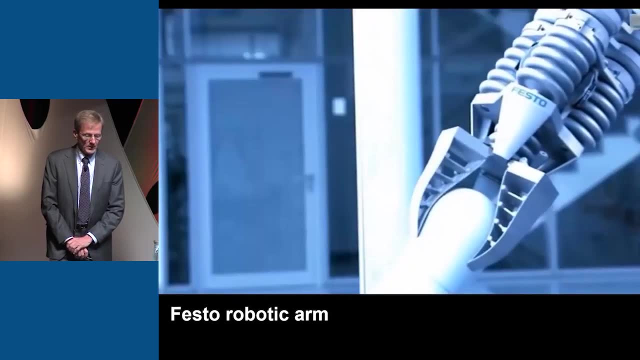 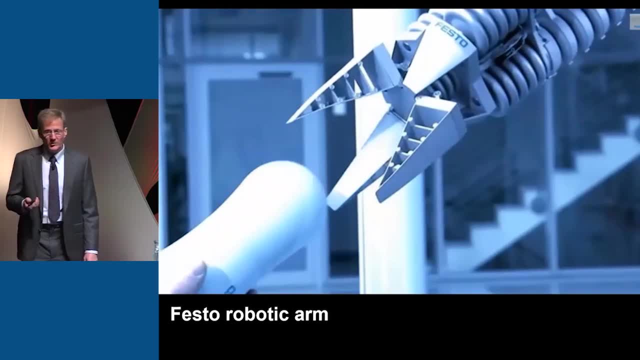 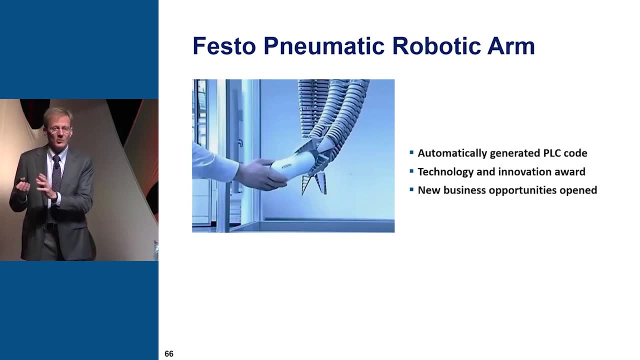 Now what's interesting for this particular design is that, rather than generating C code, which is what most people do, they generated something called PLC, or programmable logic control code. So it's the same model, but it's generating a different type of code. 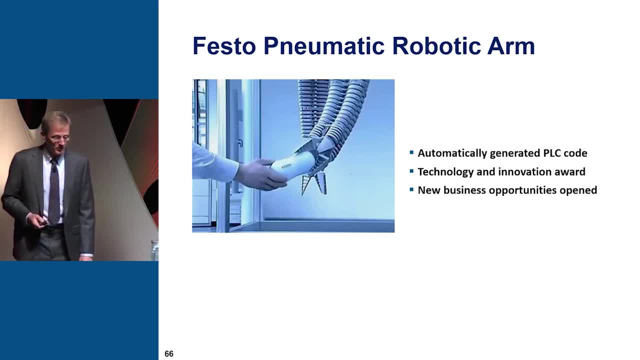 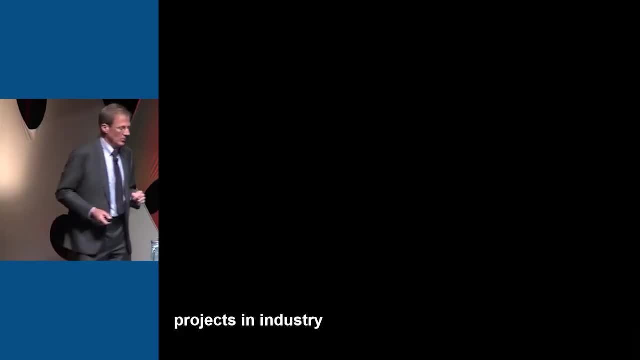 And they won some awards and started some new business opportunities. I have a video here- It's about two-minute long video- to show you some other projects in industry here And I'm going to try to talk you through some of these here to show you different places that model-based 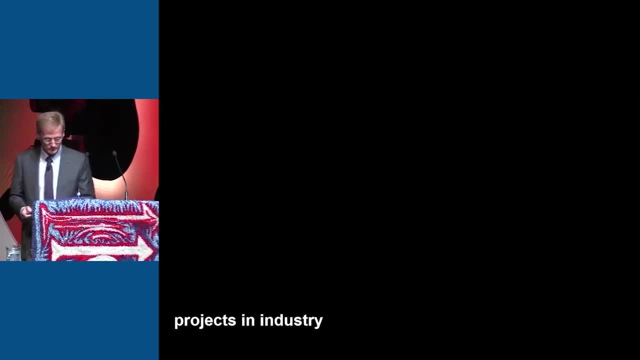 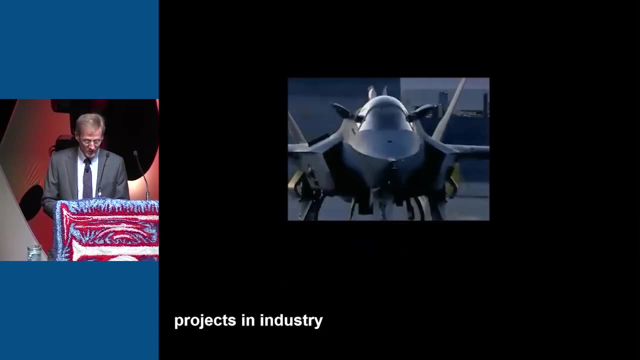 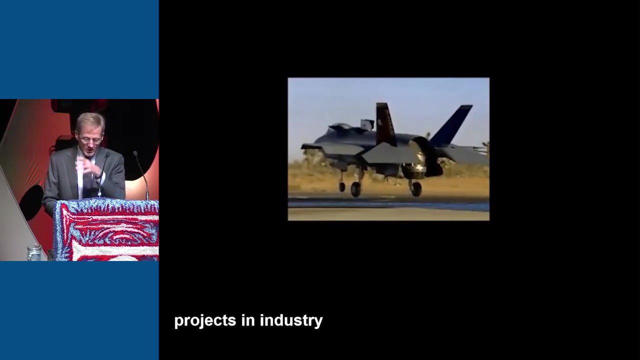 design has been used. I have some notes here on this. Okay, The first one is the F-35, the Joint Strike Fighter. This has variants for conventional operation, short takeoff and landing from carriers. Look at this now. Do you see the nozzles flip down and the control? 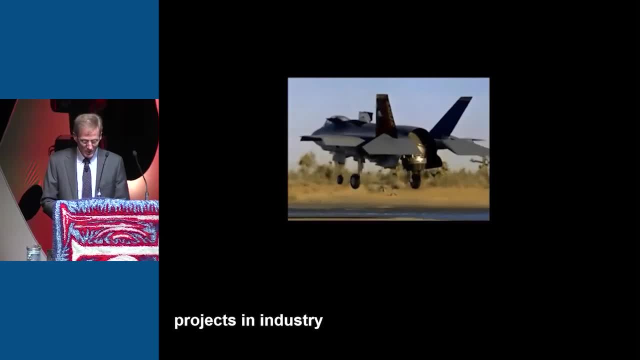 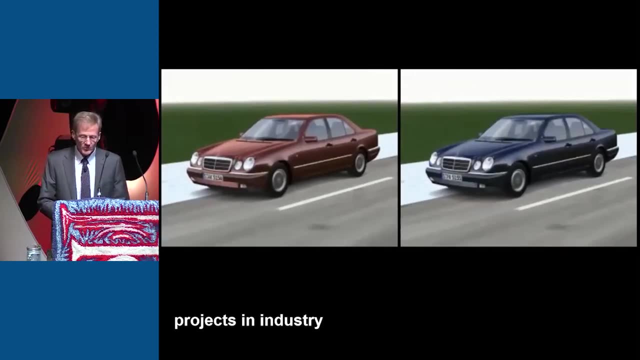 surfaces move. This is just an amazing controls problem in this vertical takeoff version here. Just a really interesting control problem. This is a Mercedes car. here The right two wheels are on ice, The left two wheels are on pavement. They slam the brakes on And 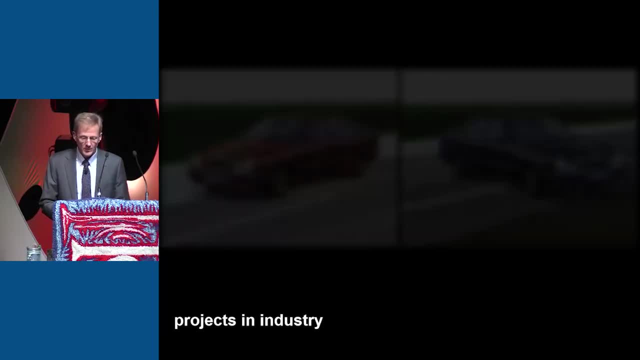 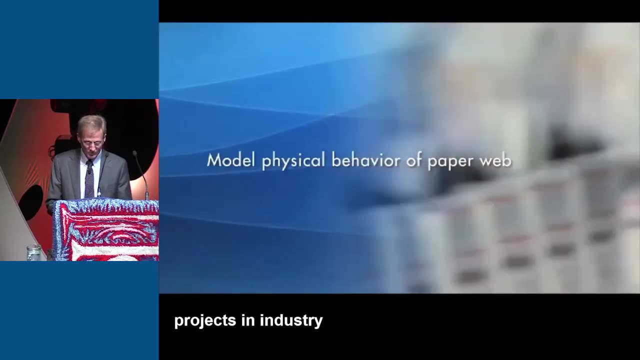 they built an active control system. They can break it on that type of slippery surface. You saw that in the car on the left. This is a ManRolland makes high-precision printing systems to develop their controllers. They simulate the paper, the control elements. 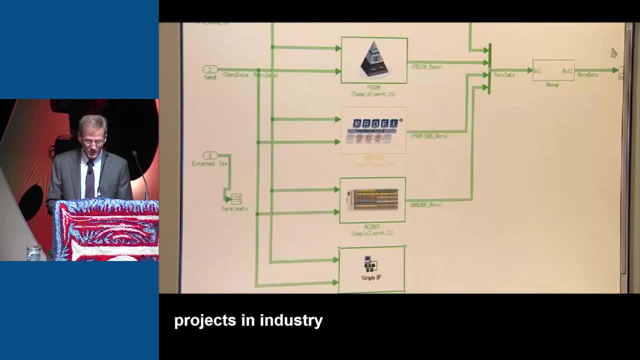 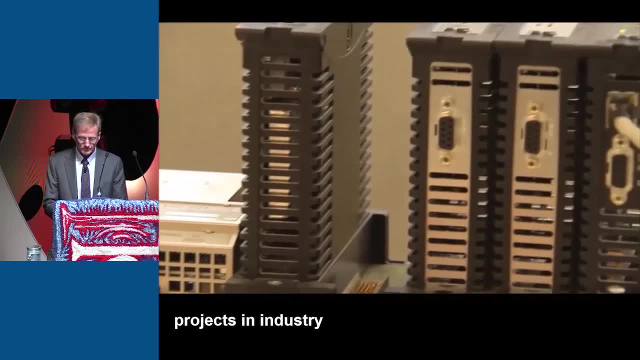 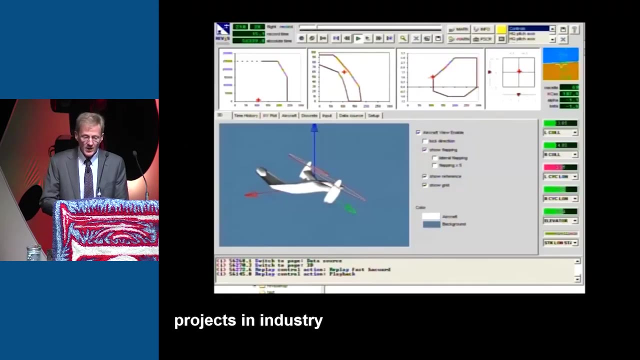 the and mechanical structures in real-time on computers. They use field bus and then they implement the controller on the hardware. This is the first civilian tilt-rotor aircraft in the world built by Bell Helicopter. They modeled it here using model-based design. After modeling it, they designed controllers. 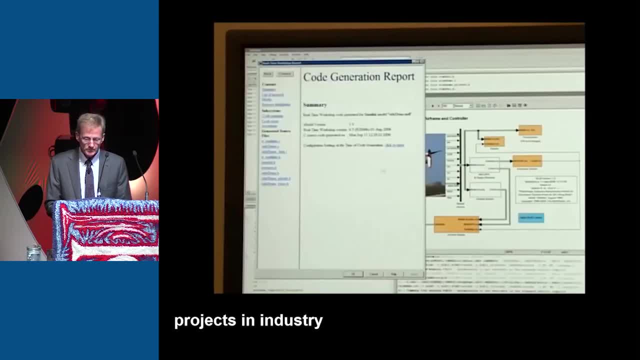 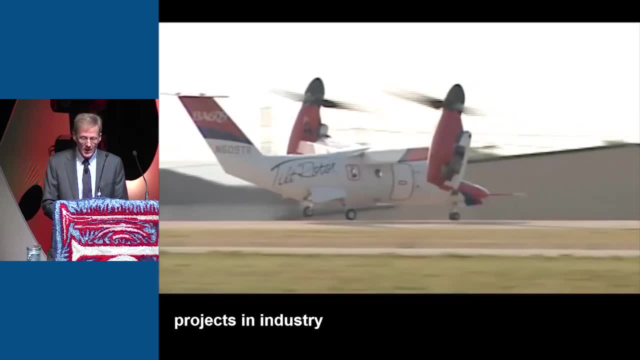 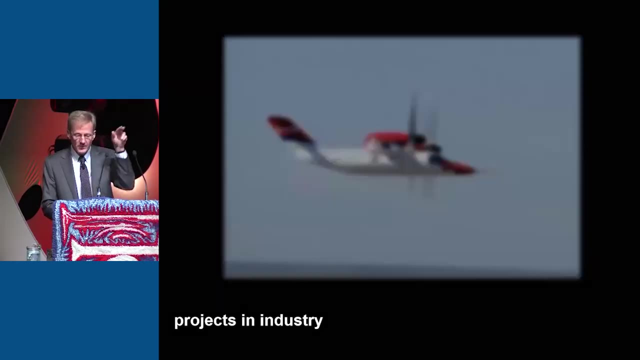 for it here. Then they generated code And then they loaded it into a simulator here to simulate it- In this case, the pilots fly the simulators- and then they proceeded to test-flight it And you can see the interesting controls Moses had. It starts vertical takeoff. 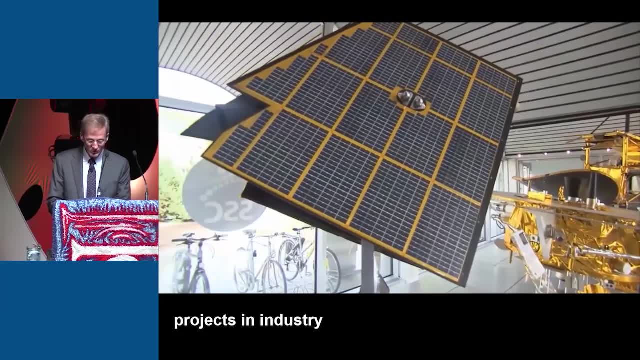 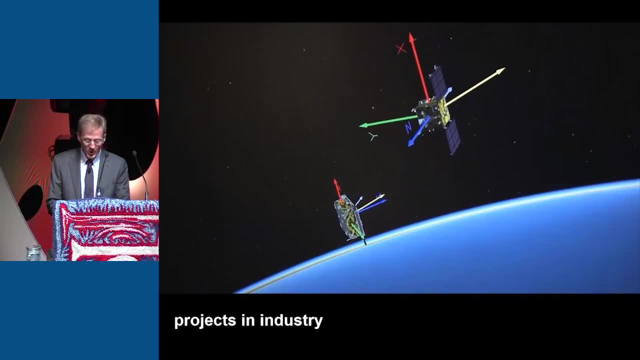 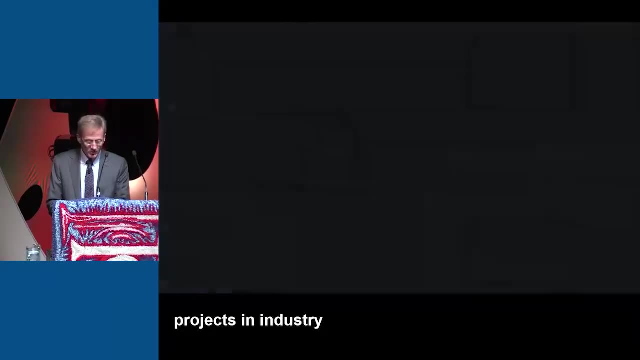 and then flies, turns into a flying board machine. Okay, this is OHB, a German company. They worked with the European Space Agency to create two satellites- They're called Mango and Tango- andto experiment with autonomous close formation flying. Here's some state-flow diagrams of different states. They partitioned 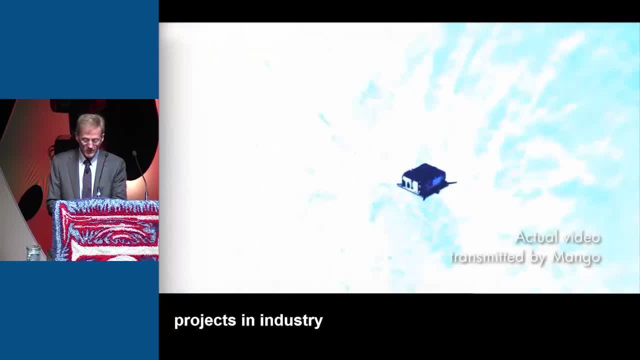 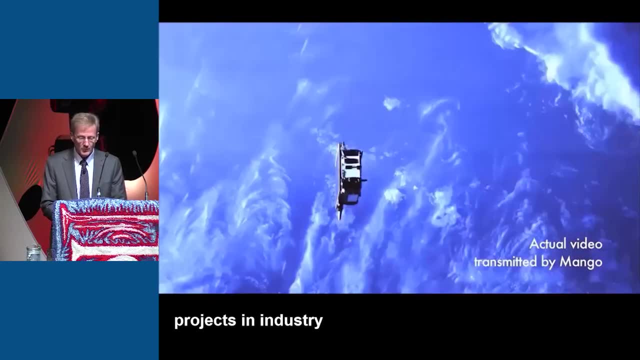 the guidance navigation control system for each building as well, And the flight engine control to three modes: formation flying, rendezvous and proximity operations. Proximity meant just a few like a meter away, And so these are doing various rendezvous operations in space. 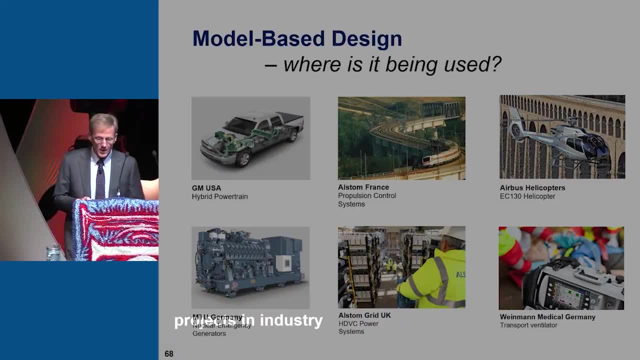 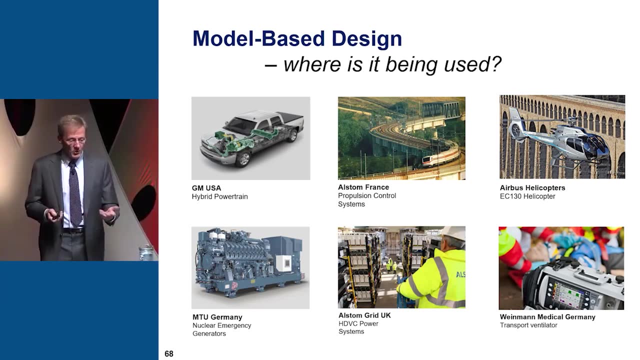 So those are a few quick examples of projects in industry. So model-based design: where is it being used? Certainly a lot in large systems like automotive, aerospace safety-critical systems. A lot of these have to be certified before they can be put into use by the public. 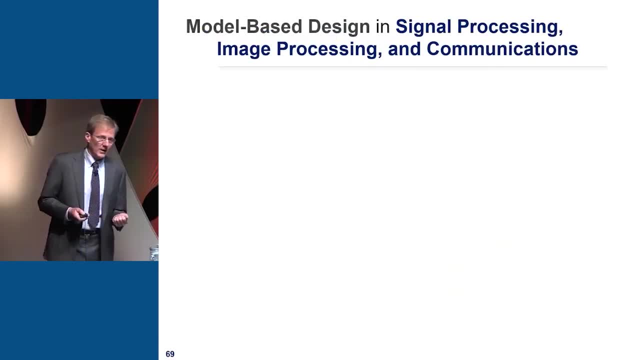 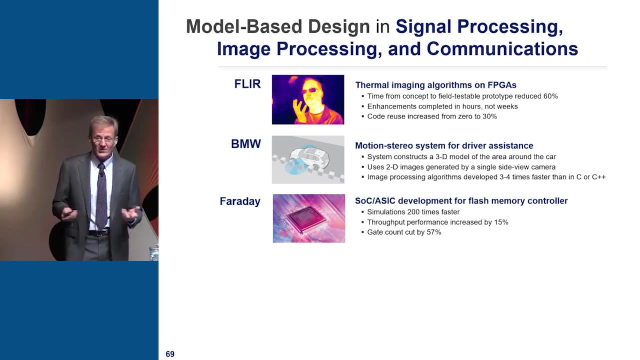 But it's also being used in smaller systems in places. you might not expect Model-based design using signal processing, image processing and communications applications that in some cases don't have a lot of control in them- Thermal imaging and FPGAs, a driver assistance software, flash memory controller. 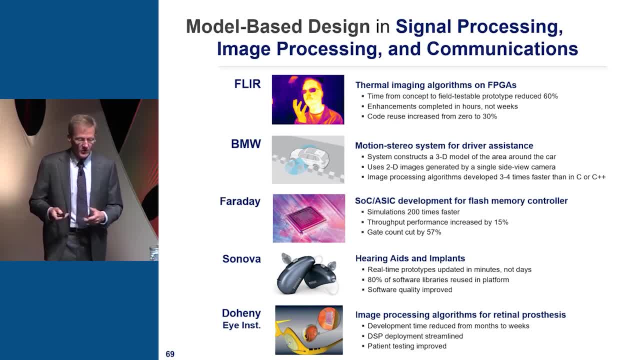 hearing aids and implants, image processing for retinal prosthesis, So a variety of things that don't have a lot of control content, but I wanted to make you aware. Of course, if you're building larger cyber-physical systems, you may be integrating with these types of systems. 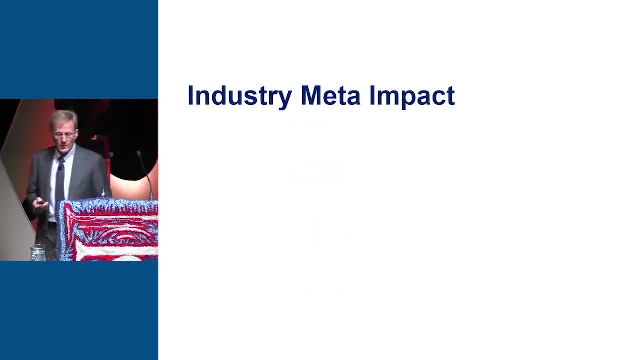 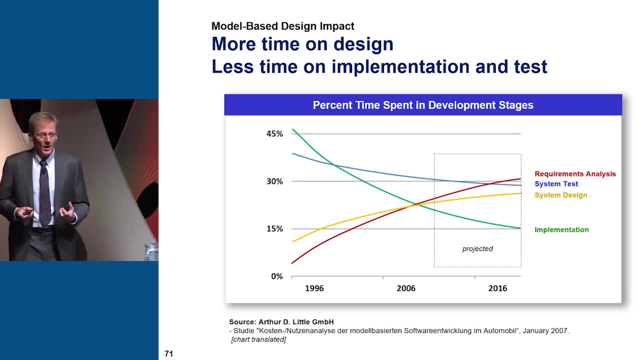 I have a little bit here now to talk about the meta-level impact on industry. This is a chart that shows the percentage of time spent in the development stages with companies that use model-based design and how that's changed If you go back a few years. the largest portion of time was spent on implementation and test. 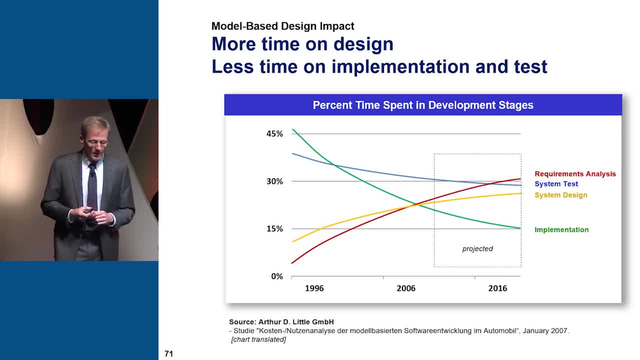 And you see, as you shift here forward in time, the implementation goes down dramatically and the requirements and design moves up. Now engineers like to work on the design stuff. The design stuff is the fun part. That's where you get to do the innovation and do the cool things. 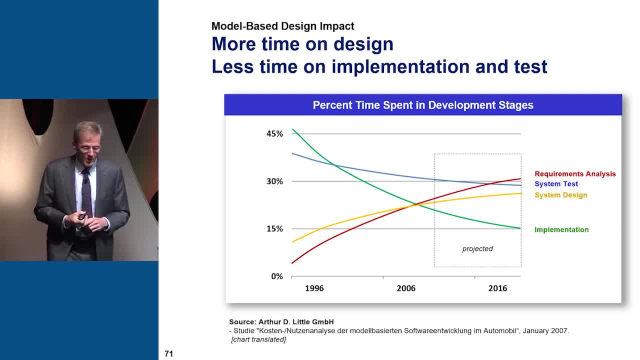 So this is a great change and really improves things. You'll notice that the test remains high. The test is remaining high because a lot of these tests are really important. A lot of them are safety-critical systems and things like that, so the test has remained high. 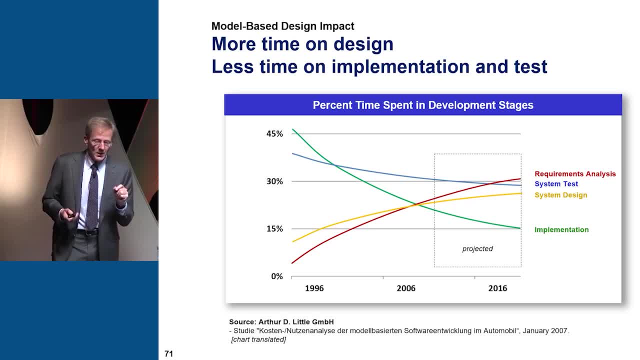 It is one area that industry has told MathWorks that they would like help. They would like help on verification and validation and testing, because that's now a very expensive part And in some ways it's not value-added to the customer. The design is value-added, but the system test. if they could reduce that or eliminate that, they'd be very happy. 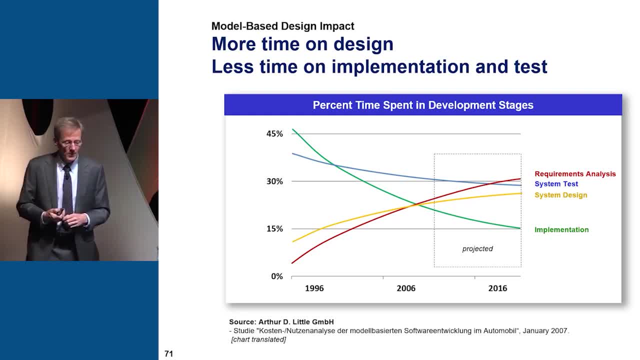 And it's actually a very active, open R&D area And there's ideas from industry very much appreciated by industry in this area because at this point that's their priority. They're very happy with the innovation and the design and the implementation, but the test is getting them. 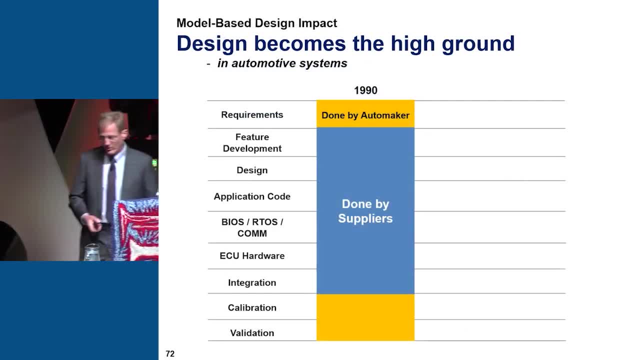 The next chart that I was going to talk about here, which you'll see in a second, is showing how it talks about in the automotive industry how the work breaks down between the manufacturer- the automotive manufacturer, sometimes called an OEM- and then the suppliers. This automotive industry has major. you know, like General Motors and Toyota are the the auto manufacturers and then there's suppliers that work there And it's part of model-based design is there's a. it has shifted there to the more time spent on design by the automotive manufacturer. 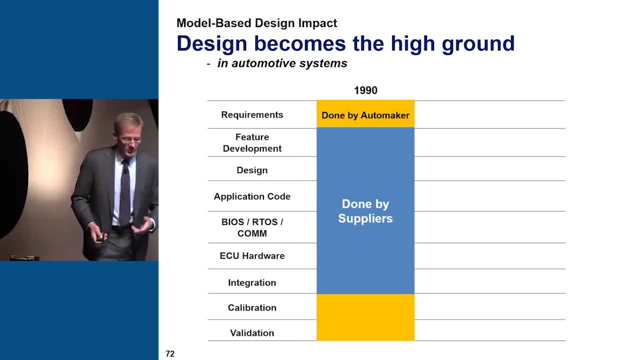 and less away from the suppliers In 1990,. this is the breakdown of the work done by Automaker and the work done by the suppliers And you can see that previously the requirements were specified by the Automaker but the suppliers did most of the work. 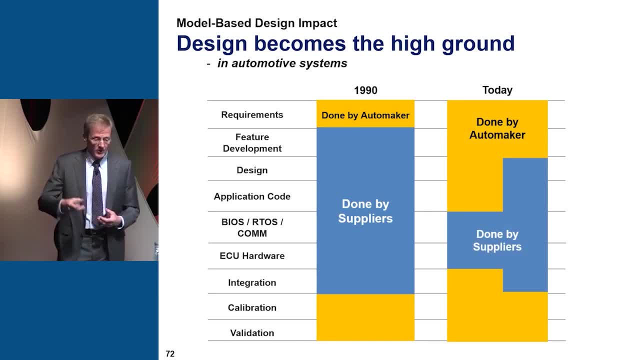 the work there and that shifted today with model-based design to the automaker doing the feature development and the design and even generating the code through the code generators and and the suppliers are being moved to more commodity types of things here and the you know the comment I have on this is: 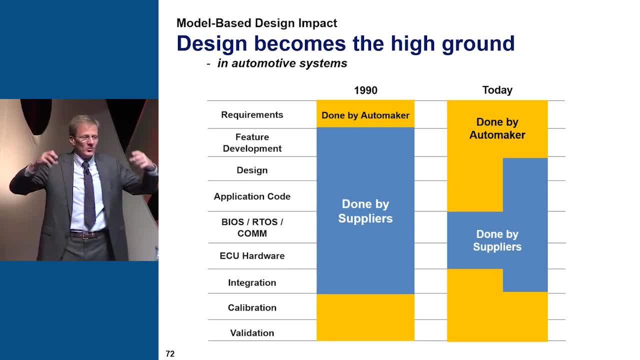 sort of design becomes the high ground. in other words, if you're, you know, design is where the intellectual property, where the IP, where the innovation comes at it, really can. it makes you choose between one car and another, okay, and the automakers want to own that, not have the suppliers creating it and sharing it. 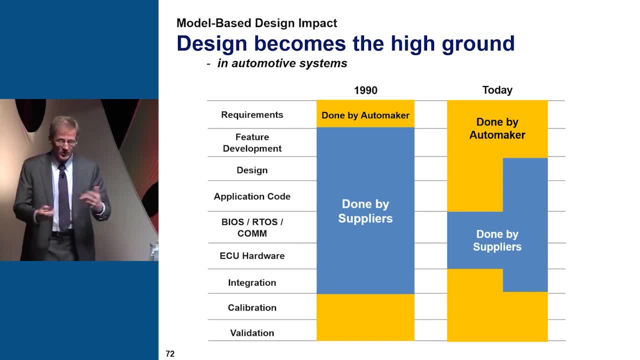 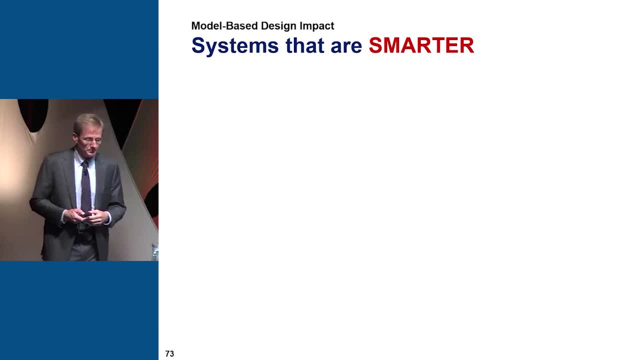 across all the different automotive makers. so this is a shift that we've seen in time here, as model-based design has enabled the supply, the automakers, to do more of that. it's also because a lot of the simple things are handled better here. it's allowed industry to move to systems that are smarter. they can you. 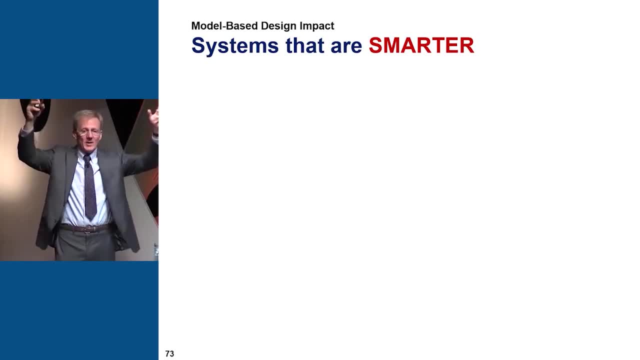 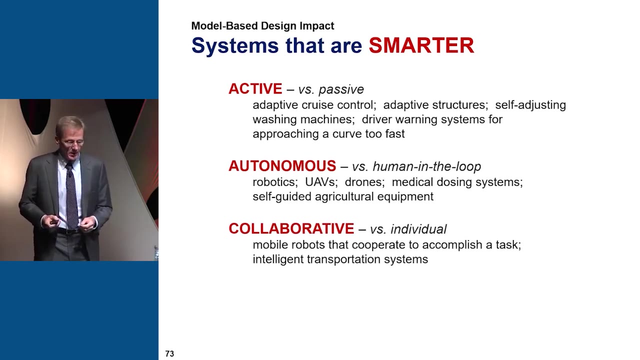 know, admit it, something gets easier. you can start to make it harder by doing more. okay, and so one of the ways that obviously are happening in the world in terms of making it smarter, well, certainly more active versus passive systems, more autonomous systems, you know UAVs, robotics, you know, those are, those are happening. collaborative systems, where 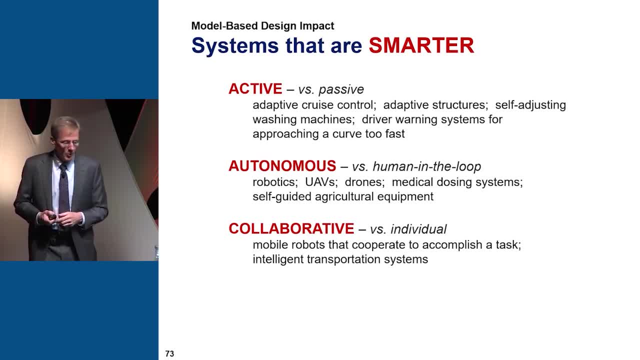 there's cooperative behaviors between robots and so forth, and then multifunction things like the hydroelectric hybrid electric vehicles. I think every hybrid electric vehicle in the world is being with model-based design because it's complicated here and and has multifunction versus single function, so it's enabling 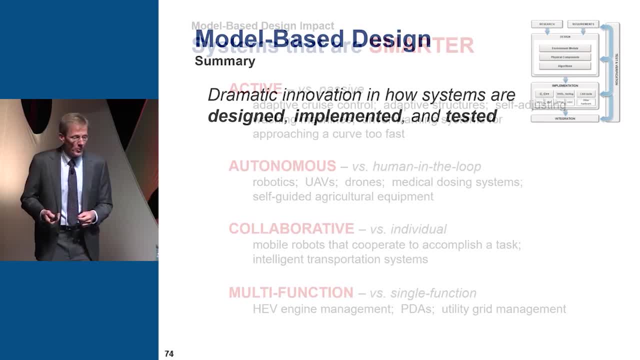 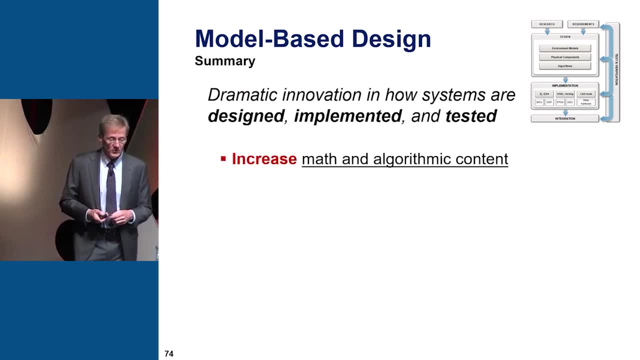 development of systems that are smart- smarter. so, in summary, model-based design is a big innovation in industry, and how systems are designed, implemented and tested. the fundamental elements are: it's allowed more math and algorithms to be put into systems. allows you to be more innovative because you spend more time. 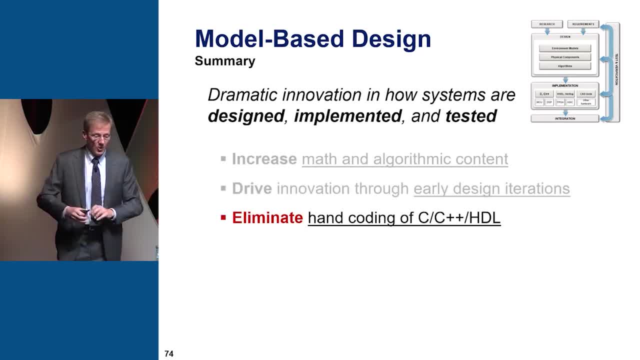 in the early design iterations where the innovation goes in, it's largely eliminated the hand coding that's so expensive and the quality is higher for these complex, often safety critical systems, because you're verifying and validating it early in the process. It allows collaboration across different mechanical, electrical engineering through the models and then. 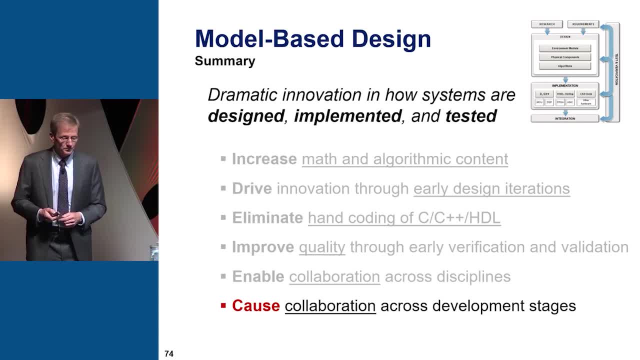 across the development stages where the models are used, shared throughout all of those. So it's a big change out there. Okay, I want to now. that's. that's sort of bringing you up to the present here in terms of what's happened in industry. I. 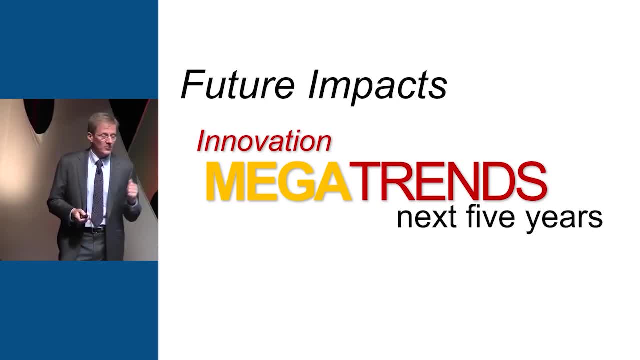 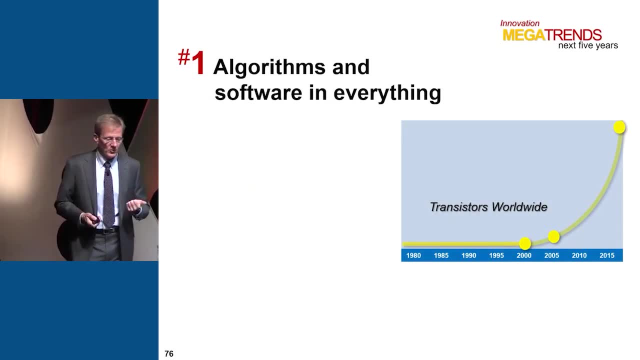 now want to shift to talking about some mega trends going forward the next five years that affect industry and, I think, affect you all- And the trend- I got four of them for you- for these technology mega trends to share. First one, that the algorithm and software and everything keeps continuing. This is a chart that 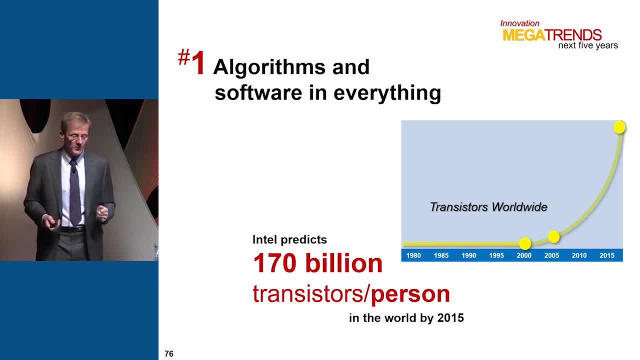 shows the growth in transistors worldwide. Intel predicts by 2015 there'll be a hundred and seventy billion transistors per person in the world. Okay, now what's interesting is in 2005 there's actually an inflection point in this. 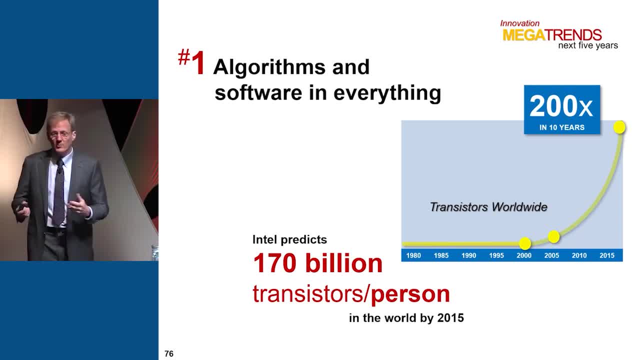 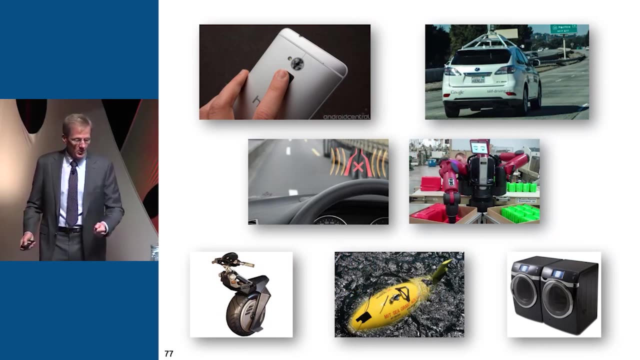 curve and is an increase of over 200 in the last ten years. So just extraordinary growth here. and of course this is all running software and largely embedded systems. We're just putting processors into everything You know: autonomous cars, your washing machine. you know you're enabling new, new systems like a. you know. 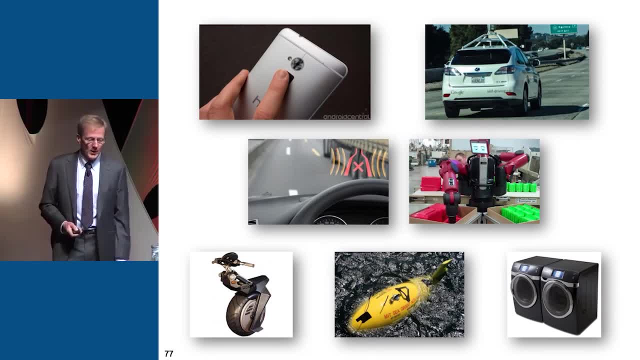 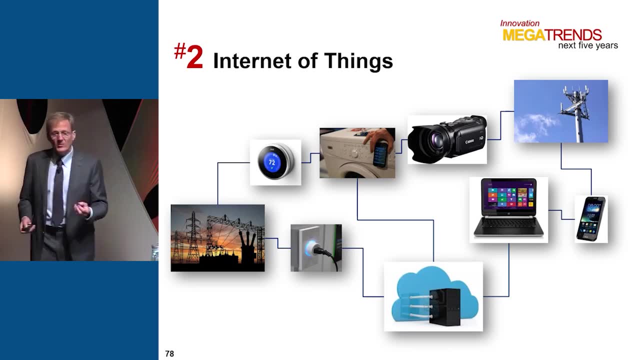 motorized unicycle. there It's just, it's just really it's going every place. Trend number two takes it up step further, and this is, of course, the Internet of Things trend. Now, this is basically putting going to take all these things that have processors in them and basically everything with an. 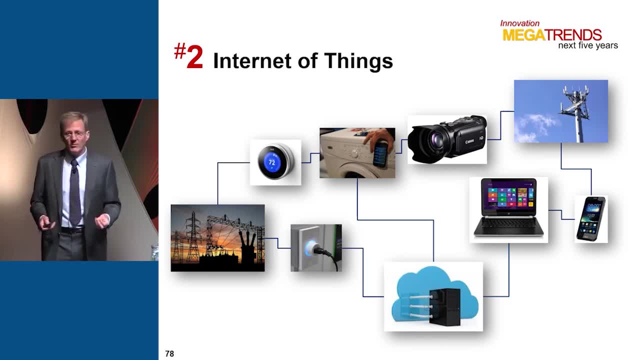 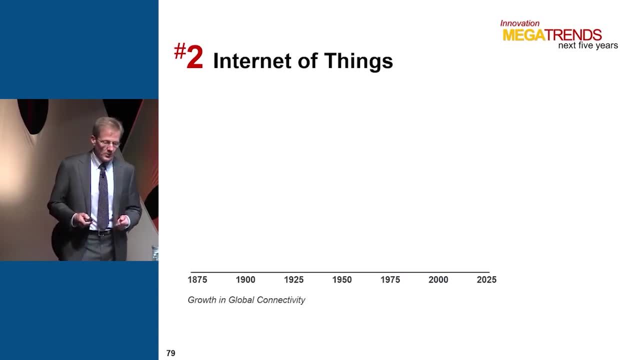 on-off switch is going to get connected to the Internet. Okay, everything with an on-off switch or a sensor is going to get connected. There's a great way of visualizing this that I really like here that I'll share with you here You can. 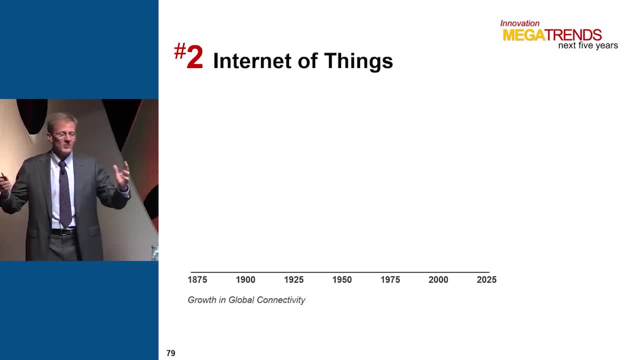 look at this as sort of the connectivity of the world, and there's there's three basic phases that have connected the world. The first phase was the connection of places. This happened over the past hundred or so years where transportation systems- you know, ships, airplanes, trains, cars, things like that- connected the 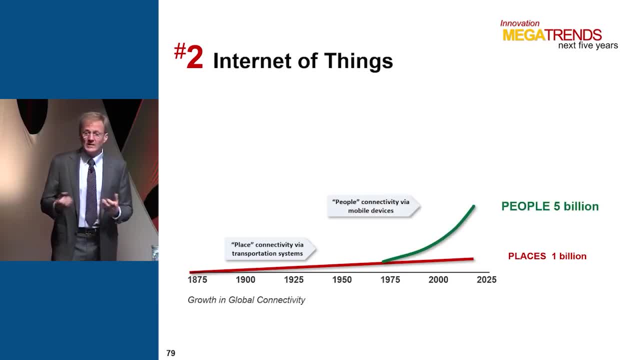 world's places. Let's say there's a billion of them. Trend two was connecting the people. This is actually relatively recent. It was the internet that came along and actually, in the last five years, smartphones. It's hard to believe it, but the Android isn't. 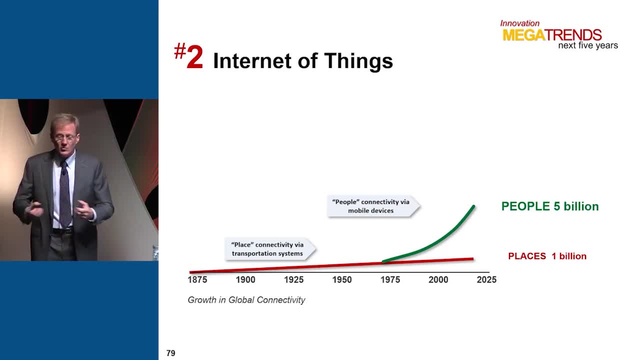 even five years old, Okay, and the iPhone is like six or seven years old, and that's truly made it so. every person on the earth, or many of them, can be connected together and communicate. It's an amazing transformation in just just a very short period of time. But the third wave is connecting not just the people in the 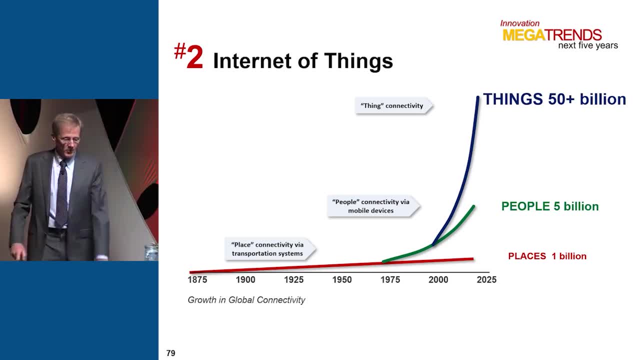 places, but all the things And, and there's at least 50 billion of those, and so that's really what's going on here, And so these are relatively recent trends. Nobody really knows where this internet things have gone or how long it's going to take or what the 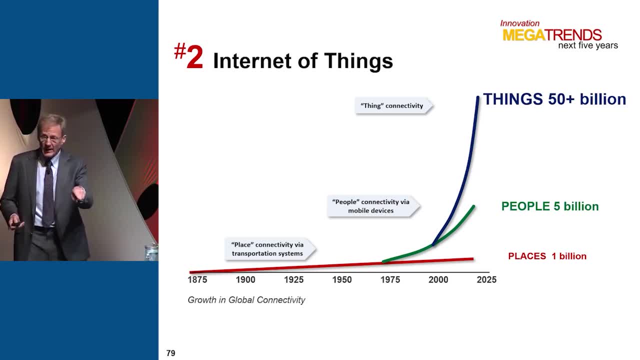 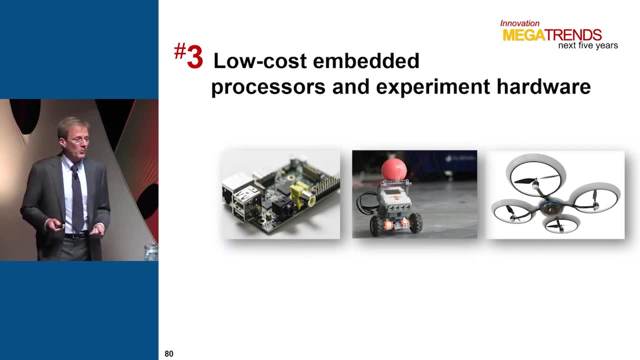 impact is, but it's definitely going to happen And it shows in the case of the people that happened pretty quickly and and the internet and the things you know, nobody really knows. My trend number three I want to talk about, which is very relevant for this community here in the room, is this growth of low-cost embedded. 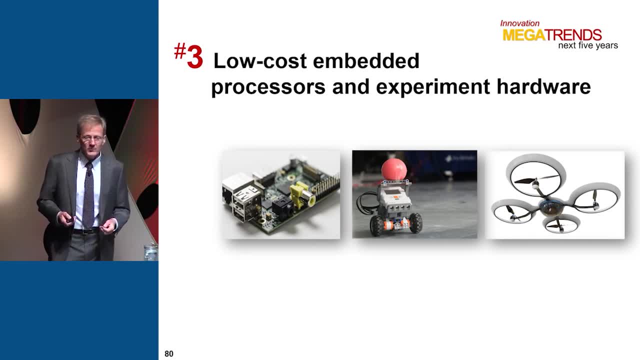 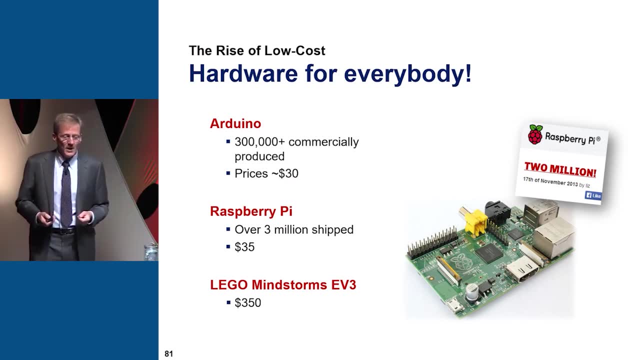 processors and experiment hardware, And we've developed these hardware support packages that connect to all sorts of things- webcams, and connect systems from Microsoft, things like that- But we have data from what the most popular low-cost embedded processors are, and those are what we affectionately call them ARL. 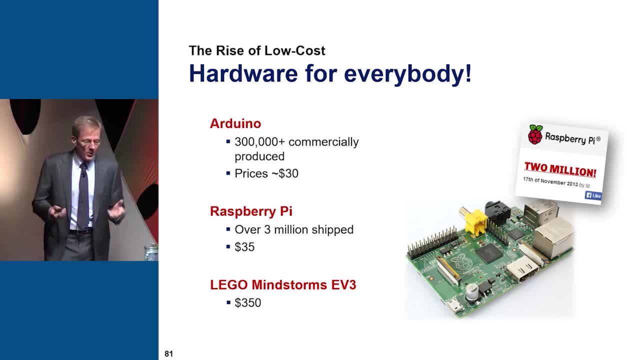 Arduino, Raspberry Pi and Lego. Okay, these are all very cheap. you know $30 for these processors. The Raspberry Pi didn't exist two years ago, they just actually cost three million, like in the last month or so. And you know very cheap processors that enable hobbyists and everybody to do it, And this is a huge. 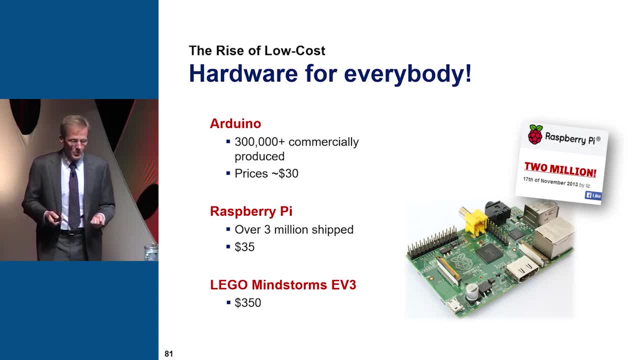 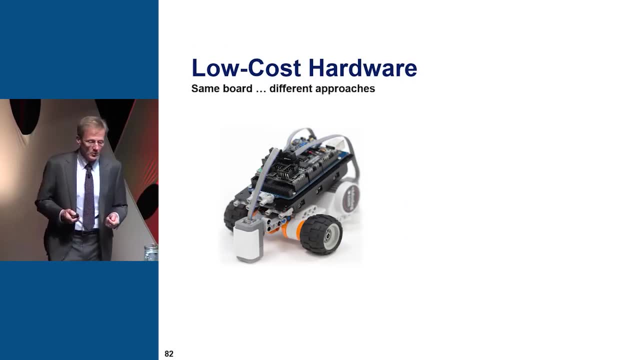 trend. I'm sure you know. a lot of you guys have seen this and that I really want to, you know, call to your attention here because it is changing things. At MathWorks, our approach has been to, in terms of how we support it, there's two. 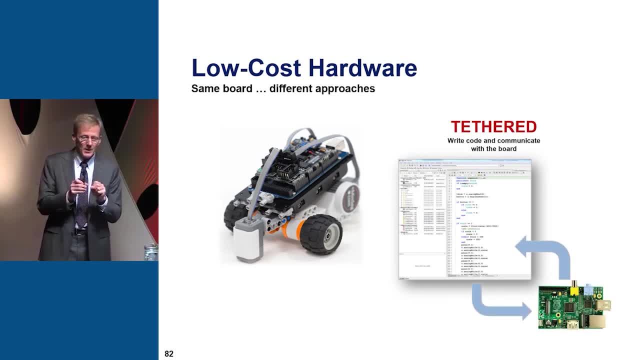 basic modes. There's a tethered mode where you can sit in that you can have MATLAB and write MATLAB programs that speak over communication- usually Wi-Fi or it could be other things- to the hardware here, in this case a small robot. Okay, that's one form. The second form is through Simulink, where Simulink 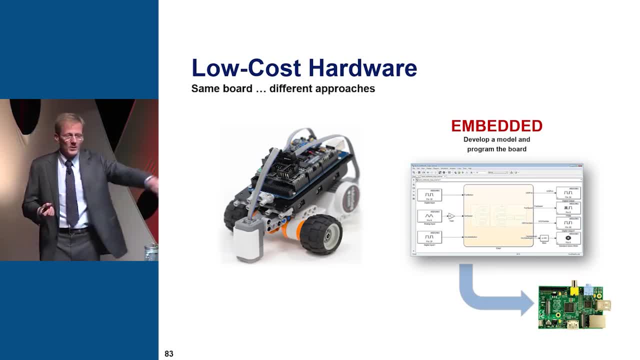 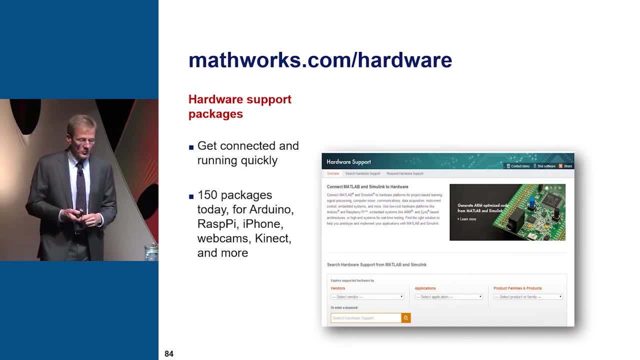 generates embedded code That gets downloaded to it and then it's autonomous and can run off and do its own thing. So there's two basic ways And we've worked to develop these hardware support packages. we have like a hundred and fifty of them. they're free, they're. 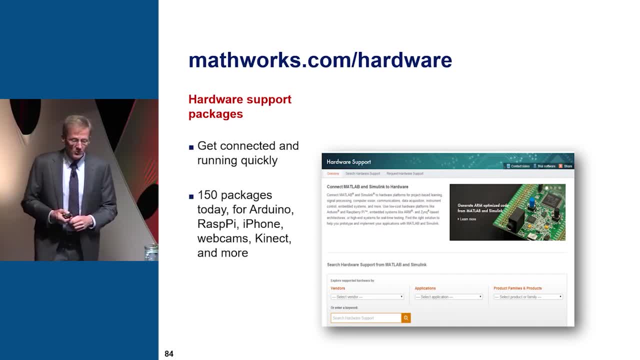 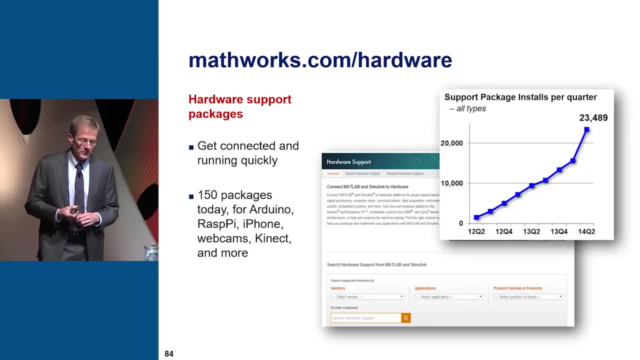 available on our on our website and they connect it all up Now there just to see the trend. you can see that this is a trend of that. this is sort of internal MathWorks data of the downloads we have in the installs And you can see it. you know, basically started very recently, just two years ago- and as the 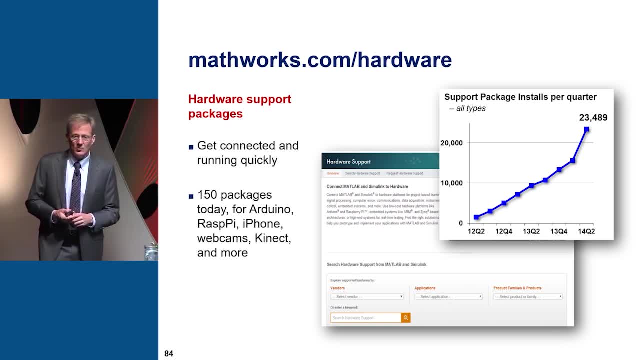 last half year there almost 40,000 or so downloads in the first half of this year, So it's a very rapidly growing trend here. as people are experimenting with with these You know we have- we have a couple of them running in our exhibit. They're 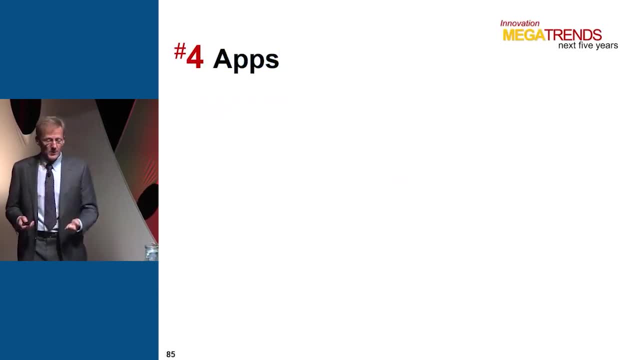 being used all over the place, And okay. and then the fourth trend I want to mention here is the growth of apps. You know, years ago with mainframes, there were thousands of applications Moved to the PC. there were tens of thousands of applications. The world has now moved to a third platform: mobile, cloud, things like. 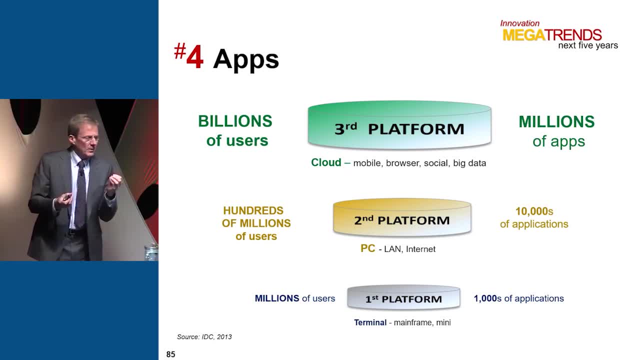 that and they're literally millions of apps, And the message is that each of us have- the world has has created a lot of little point applications. We all, we all use apps you know in to solve lots of different problems. We're used to having a lot of them and using them, And in a moment I have a message to you guys. 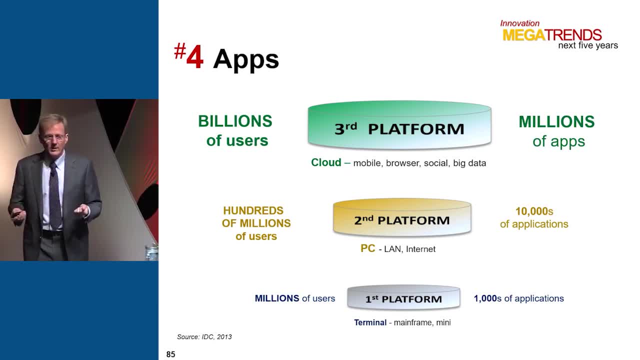 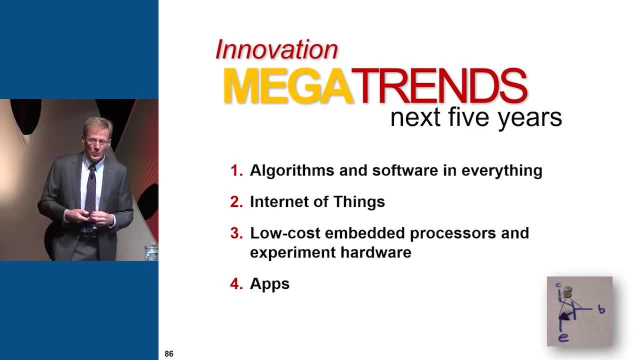 about, you know. I think there's. I think there we could use more apps in the control area. That's where people are expecting to have them, their knowledge, contained and built. So here the four mega trends that I want to share with you here that I think are really important. I think control, you know, is 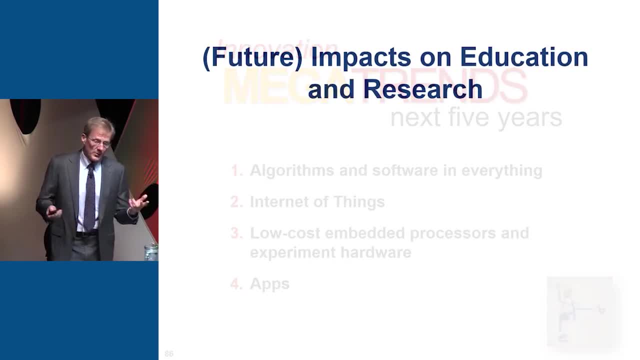 really important and these are important trends for the community, And so now I'm going to shift to talking about some of what I think the impacts are on education and research from these trends. I put the word future in parenthesis because some of you are going to look at this and say we're doing this. 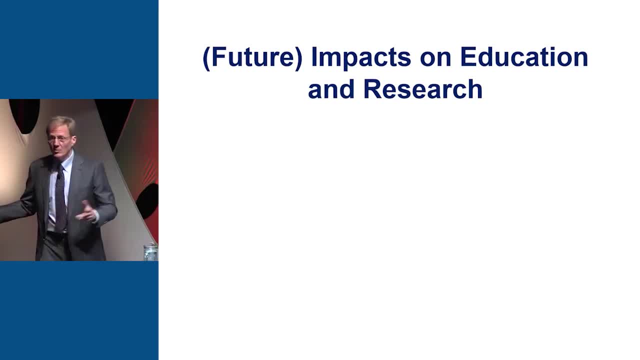 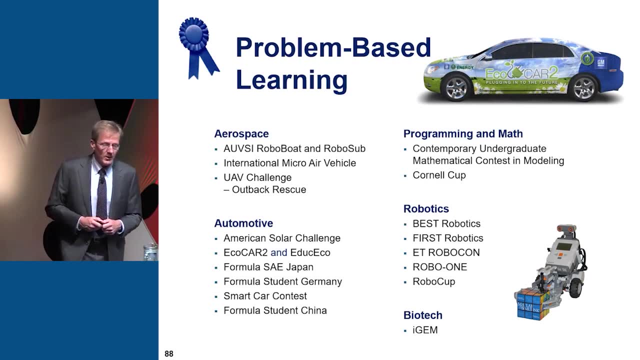 today, And absolutely you are. There's people doing this stuff, But I think the opportunity to do a lot more is really important and could be transformative on education in a lot of different ways. So one one area of particular low-cost hardware it's it's growing up, but it's also driven by model-based design and 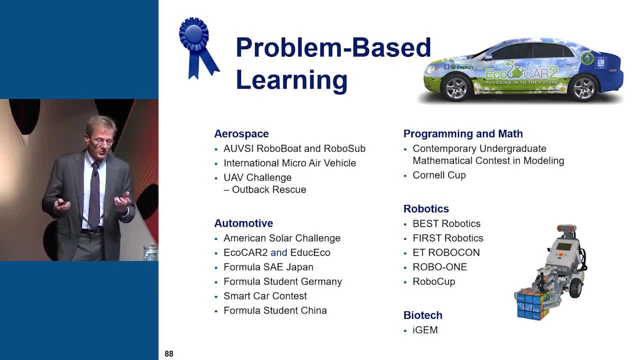 other things are this: this problem-based learning. Okay, these are a bunch of different competitions. This is just the list that Nath works. We support these, We donate money to them, We donate, have people that support them and put their time into it, And so you know these problem-based learning, these. 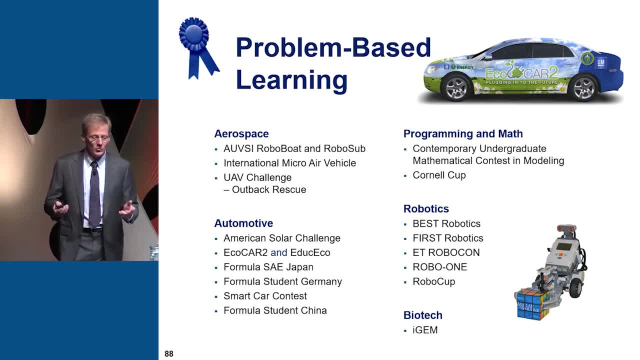 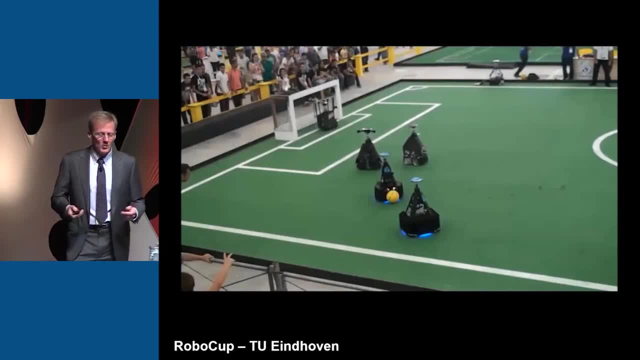 competitions and projects are just popping up all over the place. Major trend. Here's an example. I have a couple examples to share with you. This is RoboCup. Many of you might know of that. RoboCup is a contest that is trying 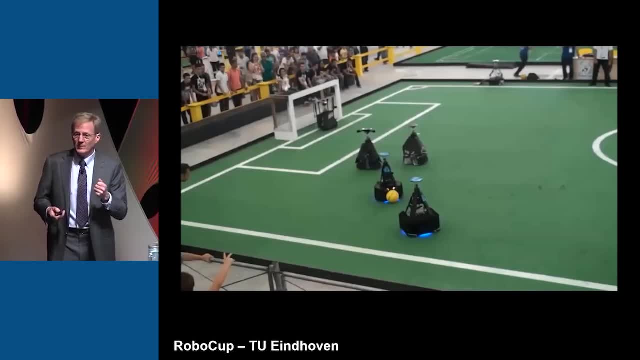 to, by the year 2050, create robots that can beat the World Cup team, The World Cup finalists in the world. So that's their ambitious goal, And and so so I'll show you, I'll run this video. This is an example, in June, of the contest here, And 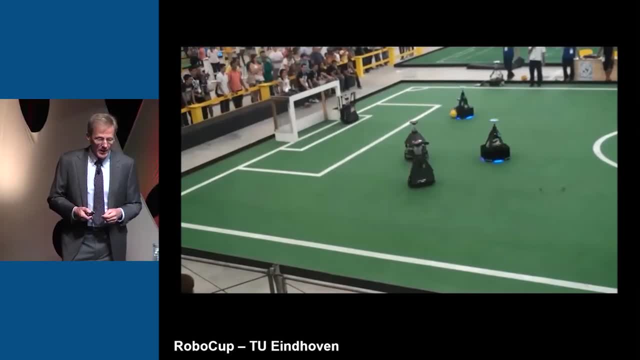 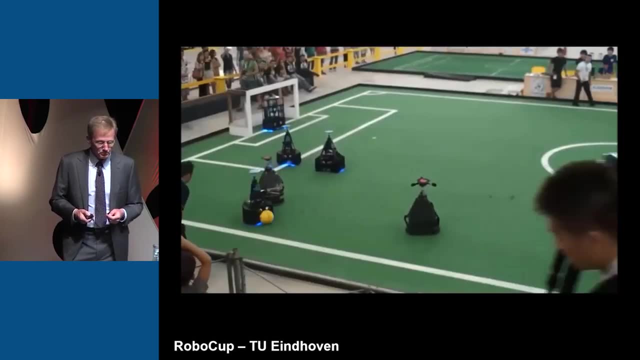 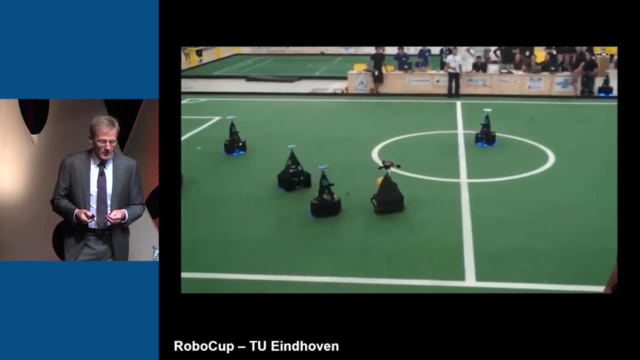 it's really quite amazing. These, these things are, are driving around. They're able to shoot it, They're they're able to avoid each other, Pass, They have strategies, So they're working together. They're moving around here. You know, it kind of looks like the German team right there, So, and it's 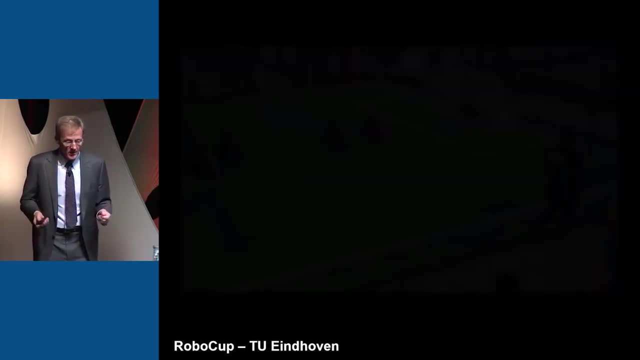 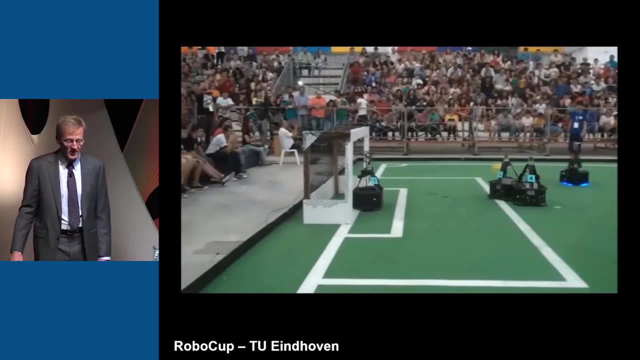 really very- if you haven't seen this before, it's, it's truly amazing. This is: this is, you know, all the stuff that's going on And these are: this is this is educational institution that's building this. Then this is sophisticated stuff. You know these guys. these guys are playing with the big boys in terms of 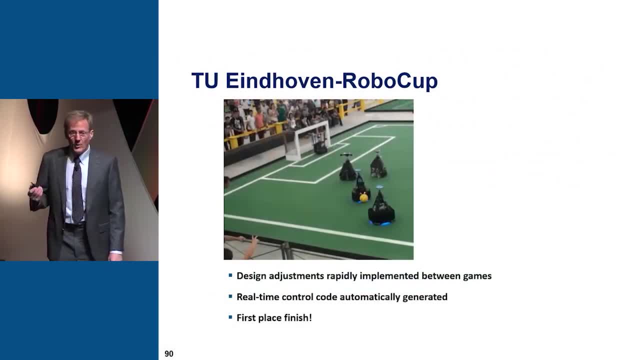 strategies. here They're using model-based design, One of the things that enables them to do. they have an advantage on that. Not all teams do that. enter that do that. One of their advantages is because they're not writing all the C code to there that they can do design. 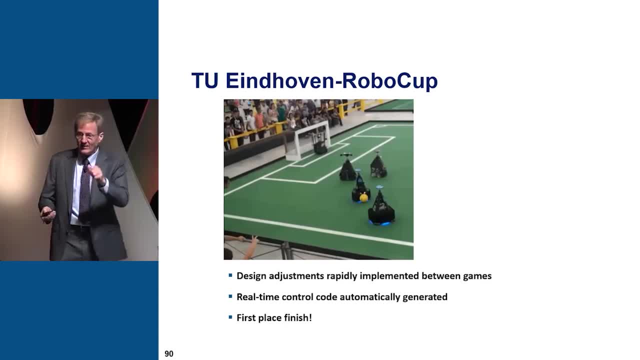 adjustments between the games. You know, like if a game is two hours apart, they can go change their simulink diagram and change the structure, not just parameters, and then regenerate the code And they finished in first place, finish in among their division in in June. Anyway, it's amazing stuff, Our comment. 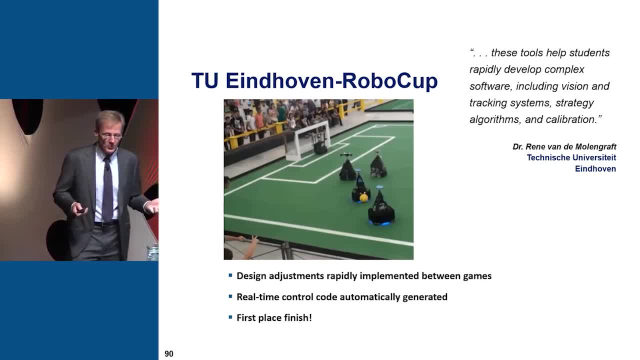 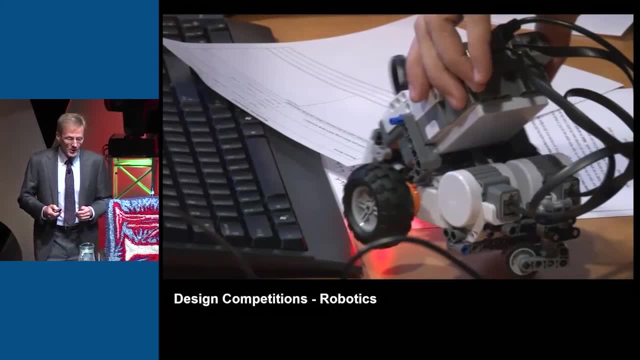 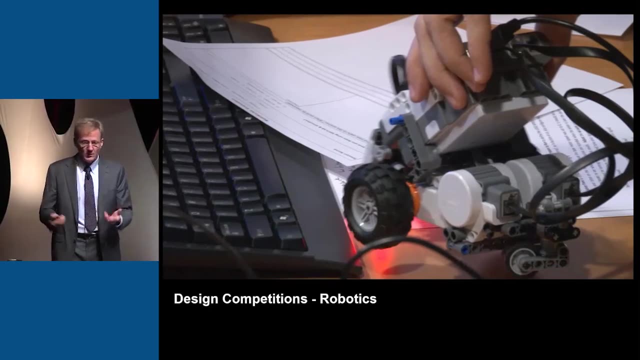 from a person involved with that is. these tools help students rapidly develop complex software, including vision tracking system strategy. There's all sorts of stuff going on here, Very interesting stuff. Here's another design- these, so these design, competition and robotics are having help, are happening everywhere. Here's a less expensive version that you 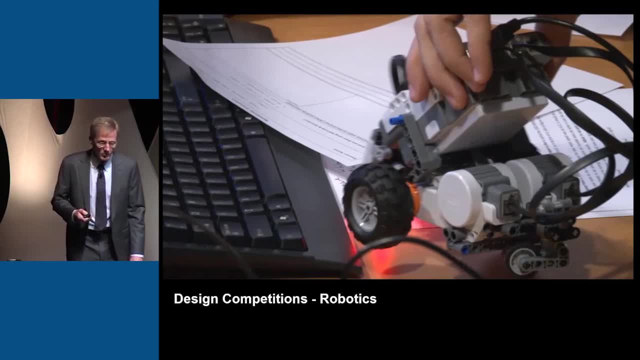 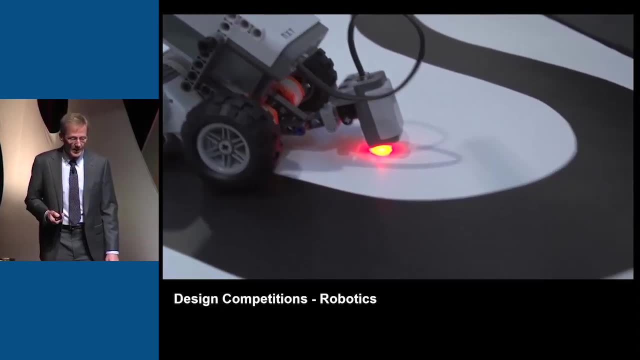 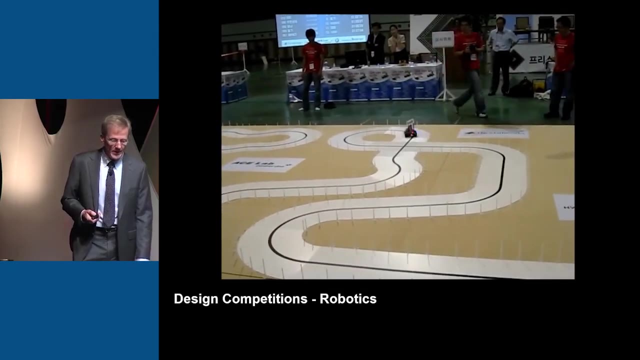 guys could could do yourselves. This is the these, the Lego kits. The reason Lego is so popular is it's very inexpensive. Using the hardware support package, you can build a simulink model. This one is uses a light tracker and to follow a line here, And this is a competition in Japan that they have on this, But they're 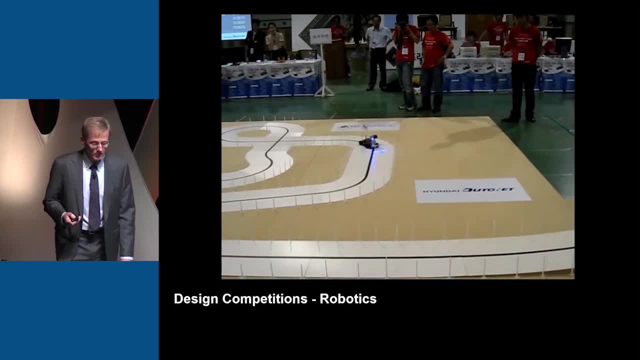 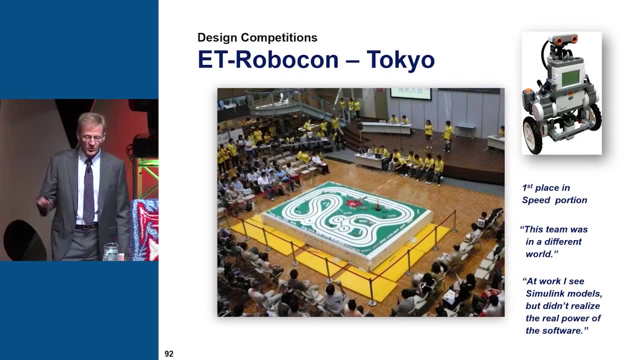 running all over the world to do that. It's relatively easy to organize. People get really into it. The there was a team that used model-based design here, there at first place in the speed portion, Some comments from other people. This team was: 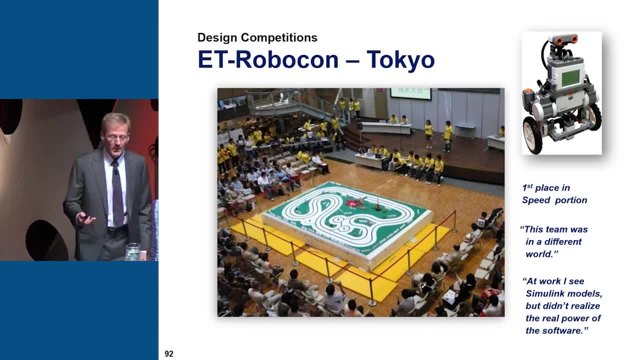 in a different world. The comment was at work. I see simulink models Didn't realize the real power of the software. Just enabling to you know they actually had models of the track and models of the car and all that were as opposed to so. 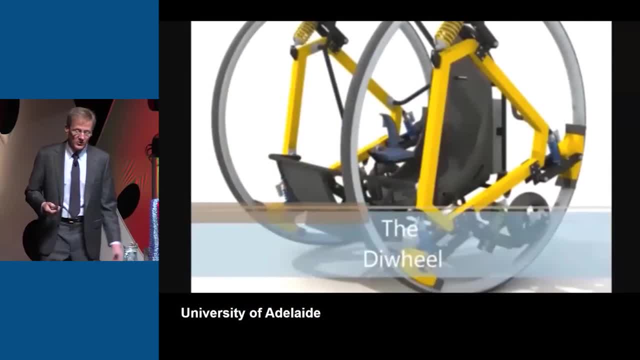 they use speed forward control really, rather than just just feedback. Here's an example. It's not a contest, but it's a project that I think is going to be a lot of fun. This is the die wheel and it's from a University of Adelaide. Let's. 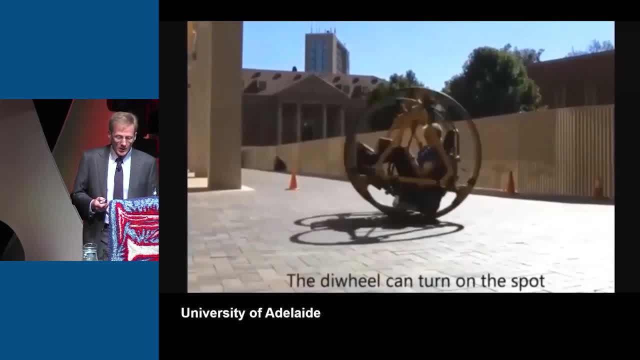 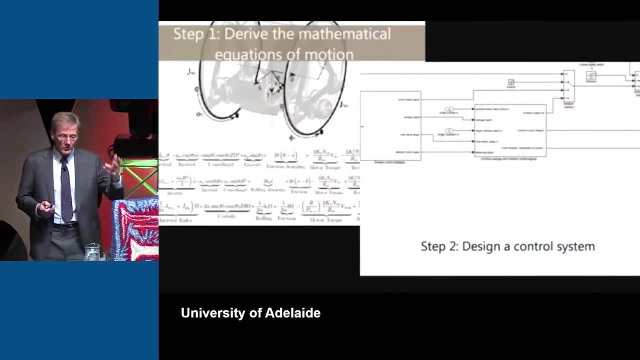 run this thing here. This is something. this is open loop now and you can turn on the spot, but it's really hard to drive because it's just unstable in terms of the passenger. So in their project, step one was to drive mathematical equations of motion. Step two is design a control system. Step three: 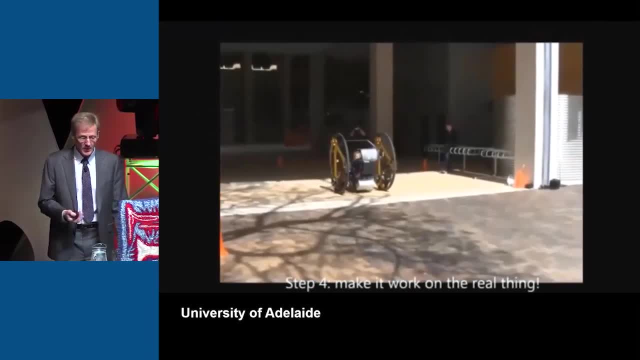 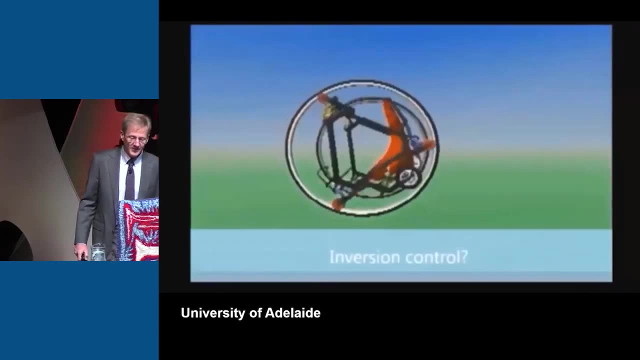 is to, to simulate the control system. Then step four is to generate code and to run it, And there you have it in a stable form. Of course, there's always a step five, which is to show off, which, in this case, is to, you know, invert. 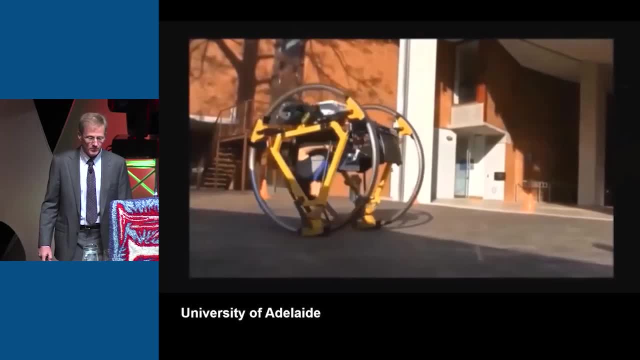 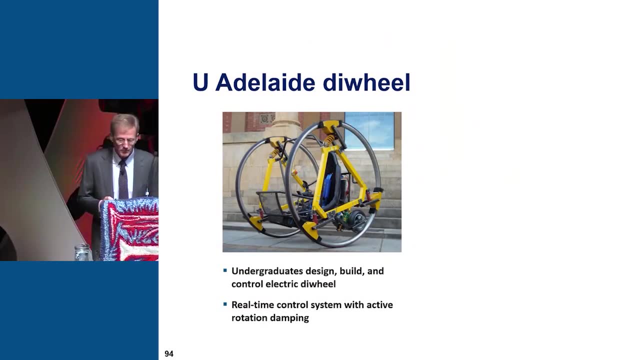 the thing and be able to drive it upside down. So now this is a fourth year project. that's done was done at the University of Adelaide. Great, you know, fun control problem. A comment from the professor involved with this. he said some of the more accomplished students after doing this project have the skills. 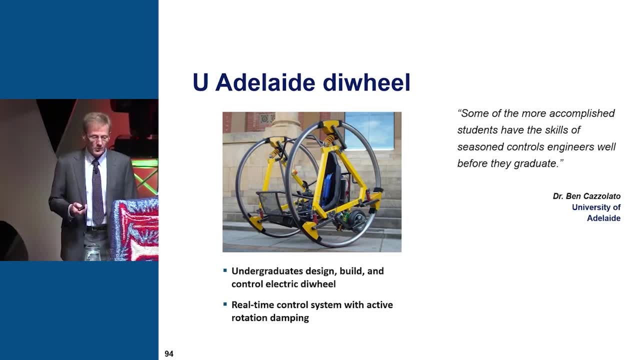 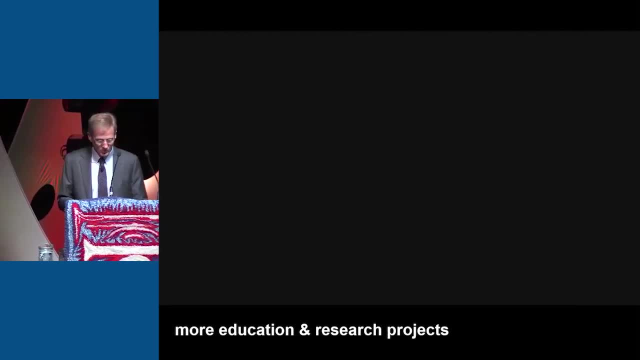 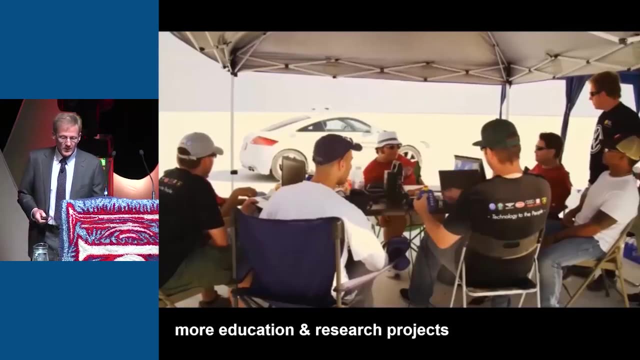 of seasoned controls engineers well before they graduate from doing a project like that. I have another sort of two-minute video that has some other education and research projects here that I'll try to voice over and walk through. This first one turn up the volume a little bit This. 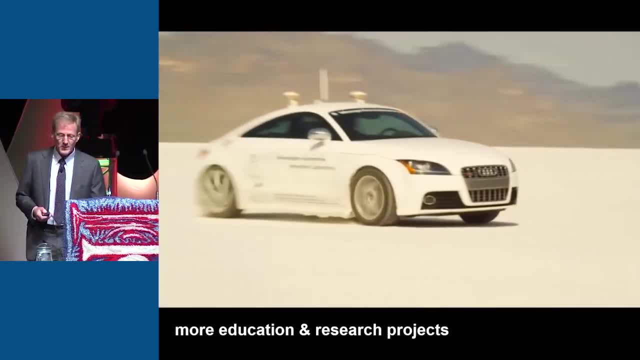 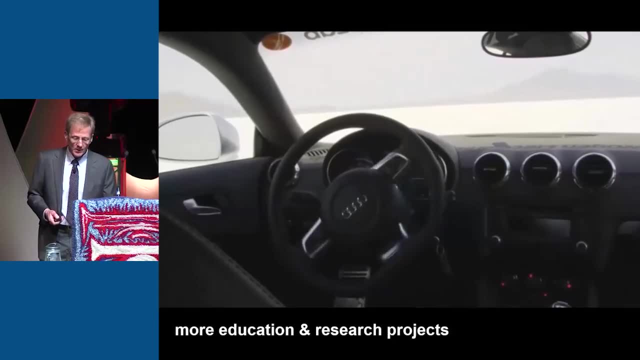 is Stanford University. They're building autonomous cars to race. They're trying to be professional drivers. Okay, look, there's nobody driving that thing. Okay, they're trying to take this around a track and actually compete against professional racers. It's a project at Stanford University and that they're. 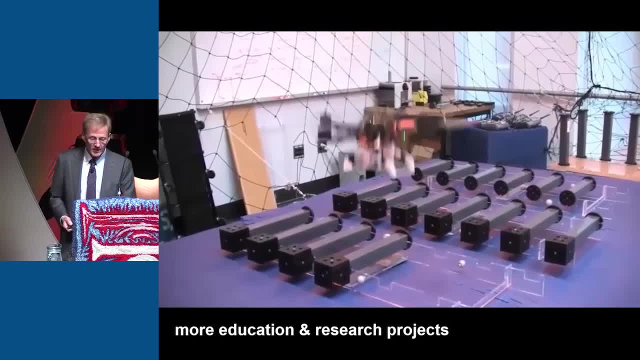 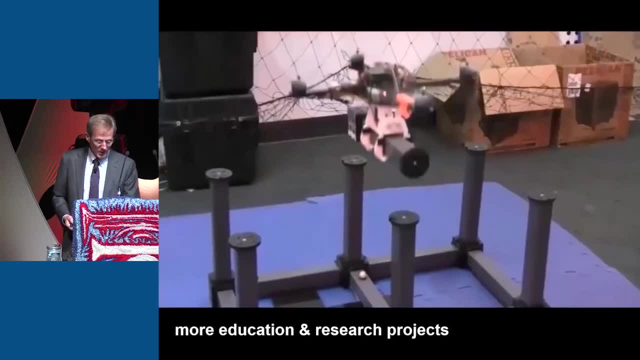 working on. Of course, quadcopters are really popular. Everybody's seeing that around This particular sets from the GRASP lab at the University of Pennsylvania. They're exploring how quadcopters can collaborate to construct- construct structures quickly. This is now speed up. 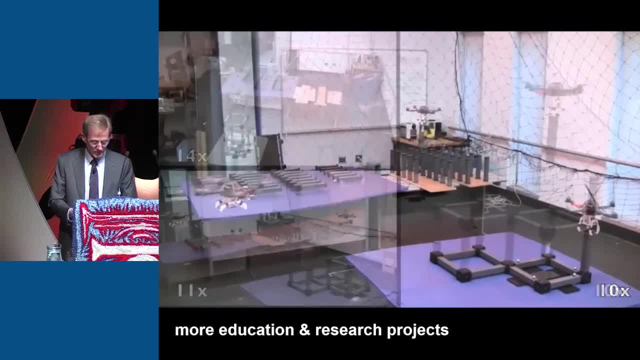 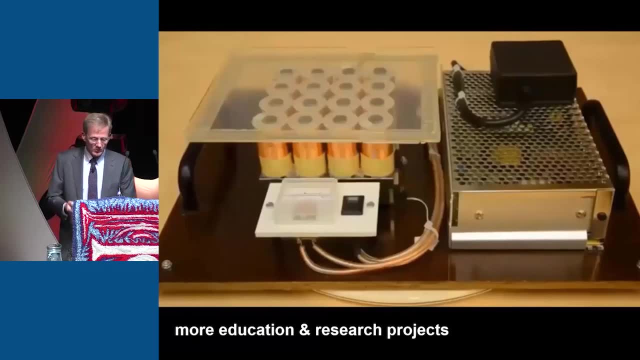 there It's sped up so you can see. you know what happens when they move more quickly. Again, quadcopters are full of all sorts of things you do. Here's a. we had a simulating student challenge. This student, by themselves, built this simple. 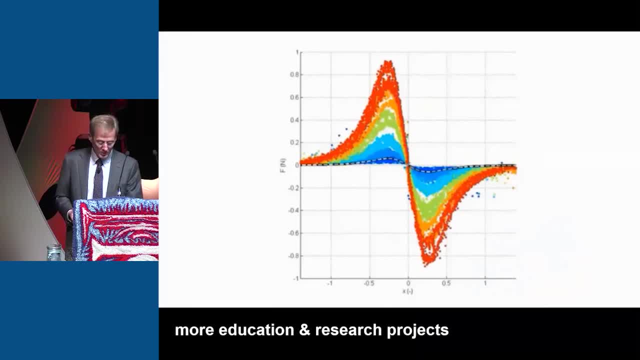 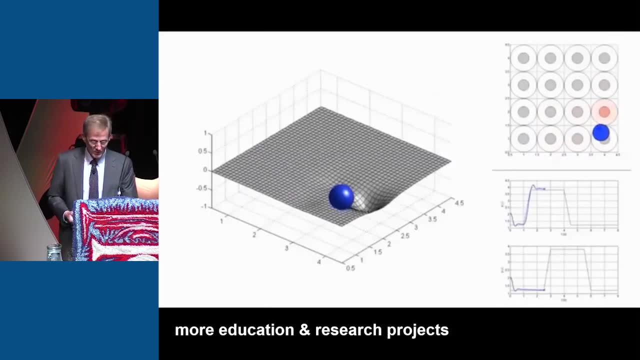 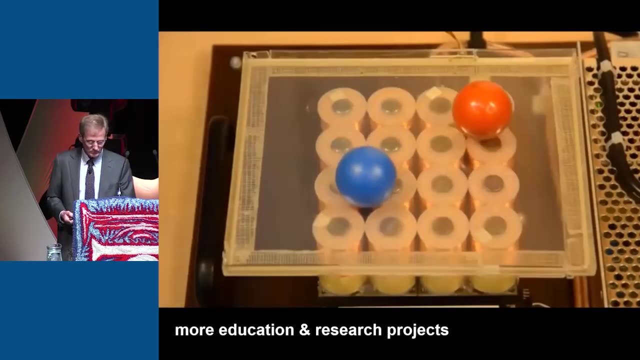 system to use electromagnet to control the position of a. He used computer vision and system identification to design his controller. The deflections in the plane show where the magnets are activated. So this is an impressive student project here doing this, This is the Formula Student Germany Competition. 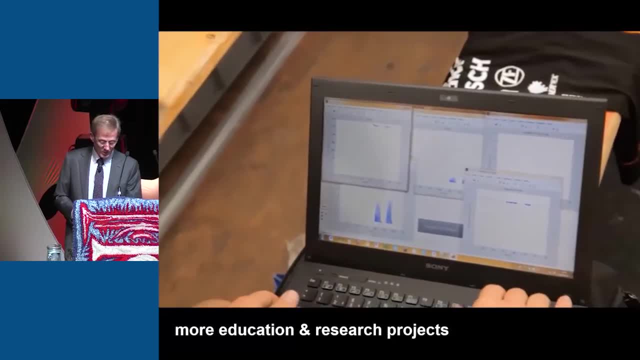 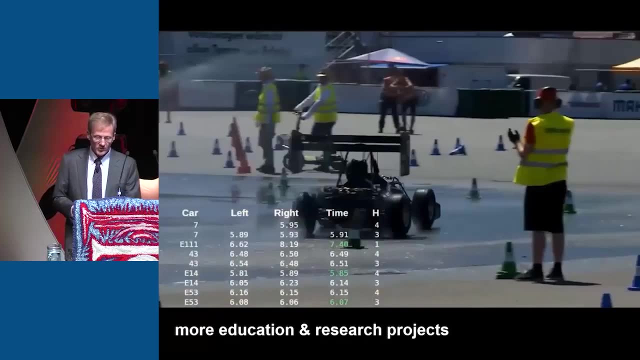 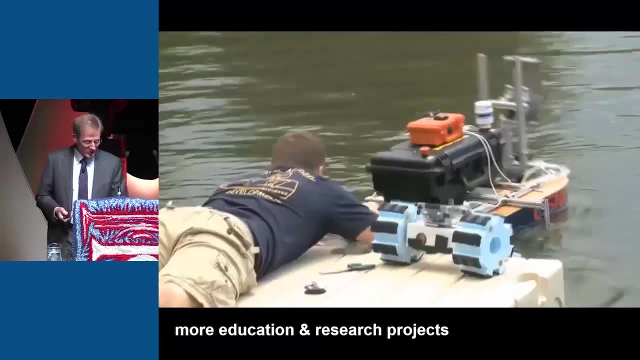 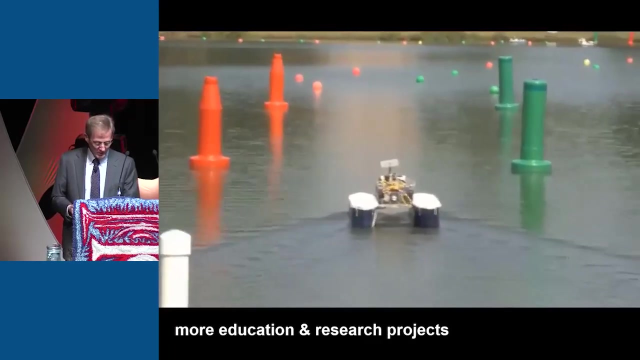 115 teams from 25 nations. They're using model-based design to simulate strategies, analyze performance, design experiments, implement controllers. This looks like a ton of fun. Let's see why the students like this. Great way to learn control If you don't want to spend that much money on a race car. this is RoboCup, where they're working on autonomous channel navigation here. 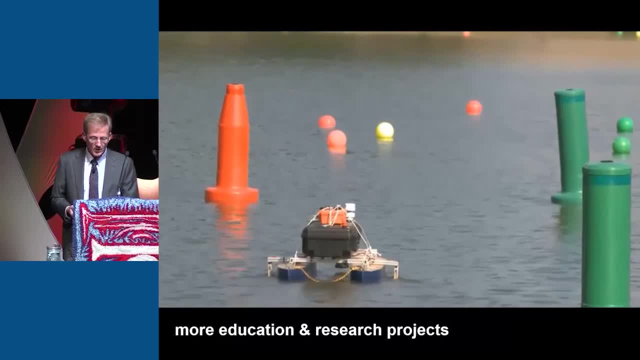 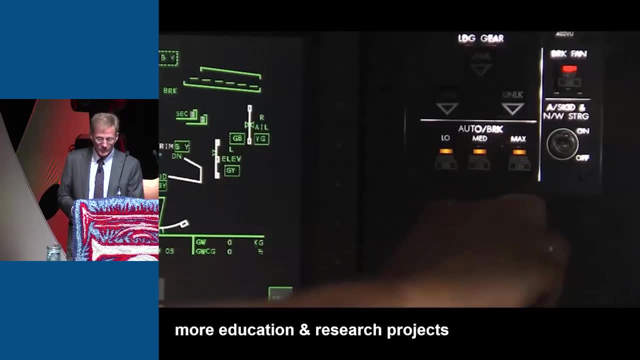 A much more low-cost rig here, But the same thing, teaching different control strategies. This is the Technical University of Munich. Students in this program design flight control systems, But then they get to fly them in a realistic flight. This is a flight simulator. 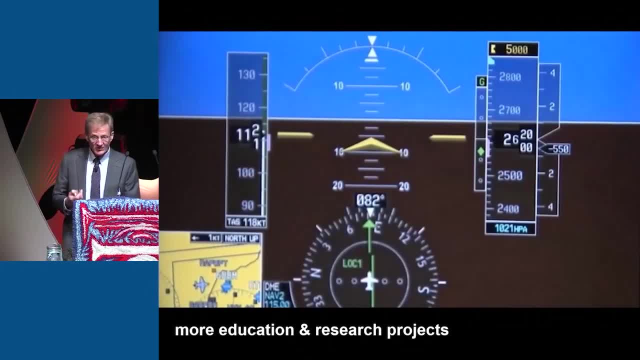 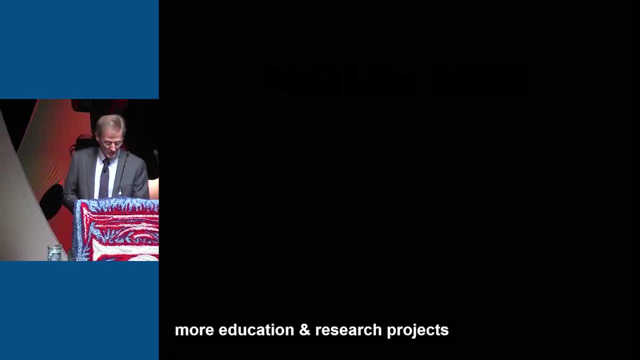 So the student has gotten into a flight simulator they have in the lab And he can actually fly his own control algorithm. So it's a great way to experience what control means and the different elements of that. Okay, Now a little bit on MATLAB apps. 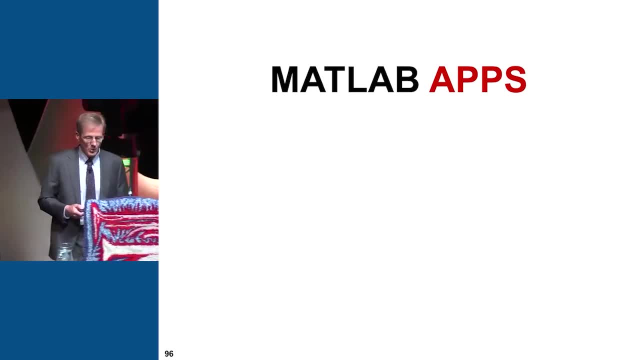 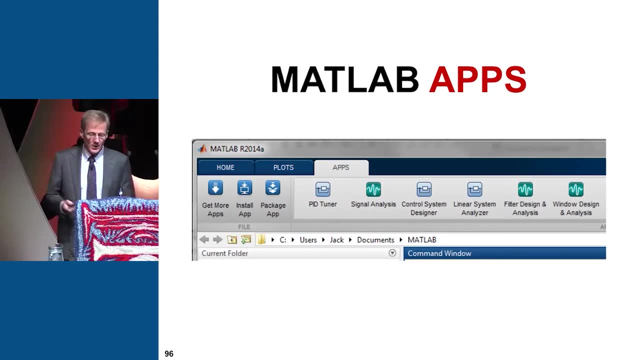 I mentioned the growth in apps, So we've recently tried to make it easier for MATLAB users to build apps and to make them visible. There's a new tablet- It's called MATLAB- on the tool strip where you can see the different apps. They used to be called GUIs in the old terminology here. 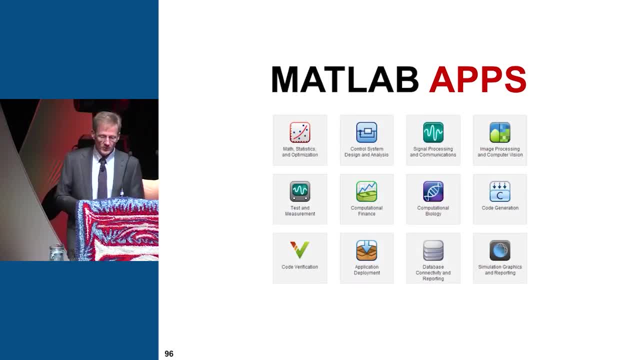 But we brought them forth and made them more prominent, And there's all sorts of different apps available now that are available quickly and easily through that tool strip. What I'd like to do is share with you an example of an app that was developed fairly recently at MathWorks to hopefully inspire you into these types of apps here. 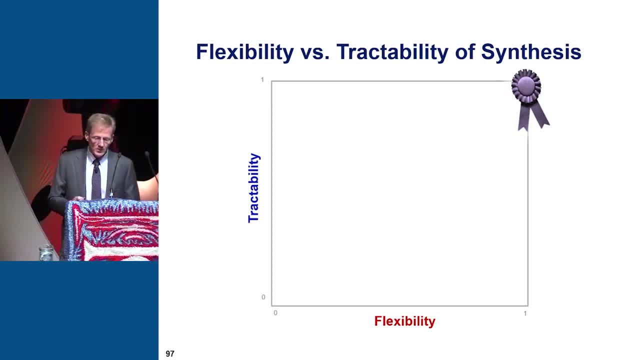 And this one is robust control synthesis. This is a chart that's going to – I'm going to show you sort of an axis here that has the tractability of the control solution versus the flexibility of the solver. You can put classic mu and LMIs, you know that, have good theory, tractability, but not necessarily that flexible. 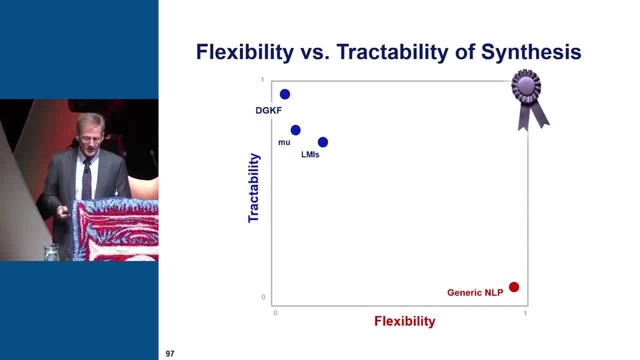 On the lower right side is generic nonlinear programming where you can throw it at anything And that doesn't have a lot of theory, but it's obviously very flexible. Anyway, Pascal Guyenet from MathWorks and Pierre Apcarian at the previous IFAC published a paper where they called structured H-infinity synthesis. 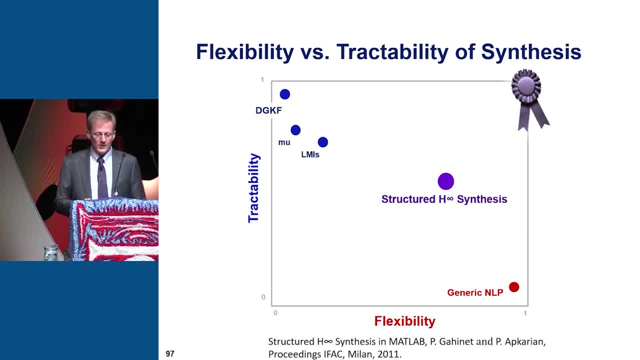 And this is a chart. This is the H-infinity synthesis that tries to put something in the middle there on that picture And basically you know part of what this new technique does is. it says: you know, this is the way – this is Pascal speaking here. 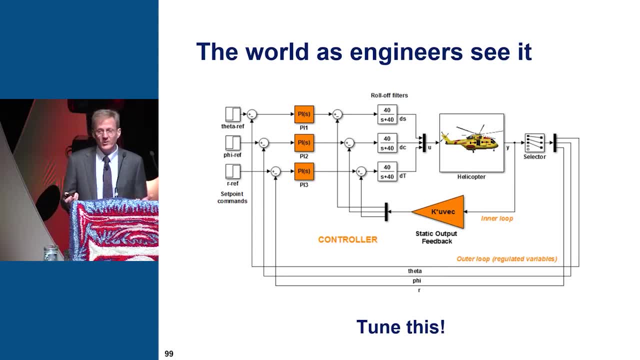 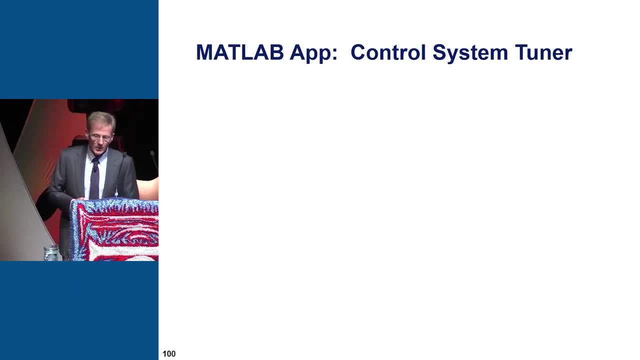 The world is robust. Control theorists like to see it, But the world's engineers see it who are working inside Simulink, and it's hard to connect the dots between those. So what Pascal and his team built is a MATLAB app which is called Control System Tuner. 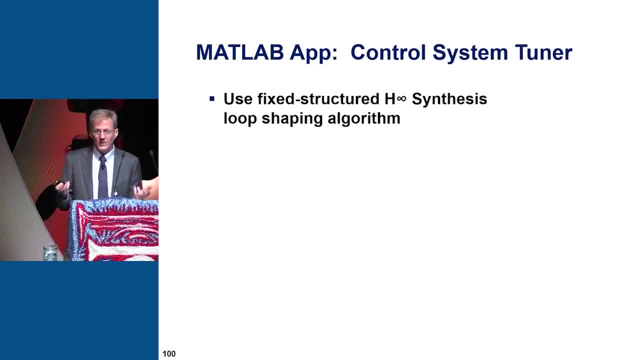 And basically it's going to use this. And basically it's going to use this fixed structured H-infinity synthesis algorithm And it's going to use it to tune a controller in Simulink. You'll specify the blocks. you want to do the goals. 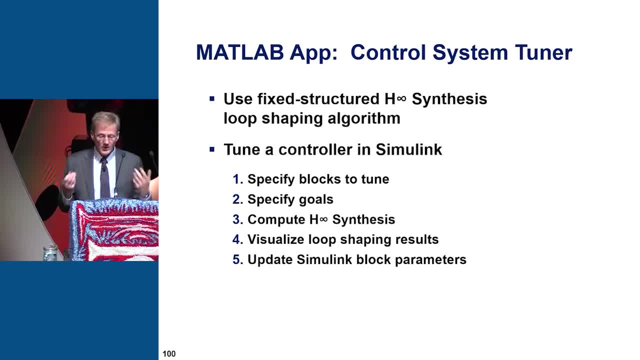 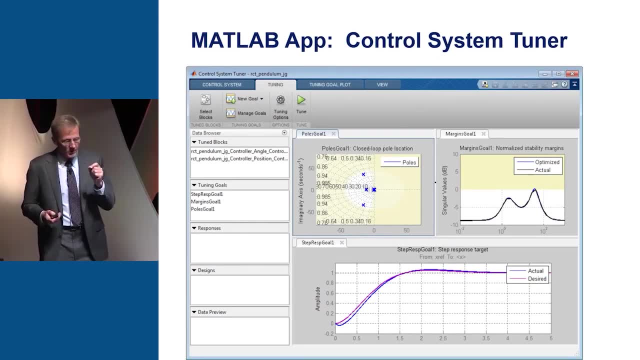 You do the synthesis, You visualize the loop shaping results And then update the Simulink block parameters and rerun the simulation. Okay, So you're going to see robust control design now in 50 seconds. You're going to have to watch close. 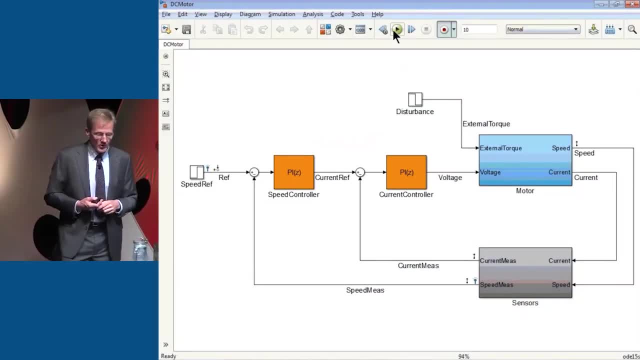 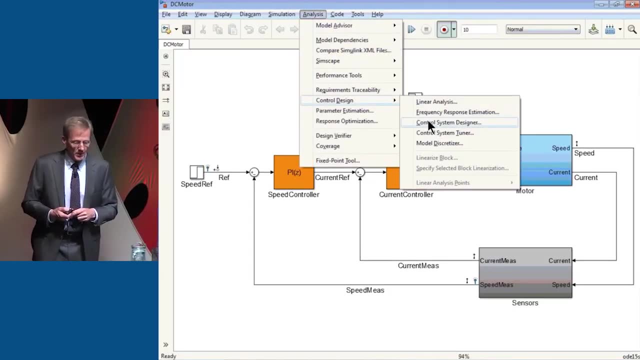 Okay. So here are the blocks to tune. Okay, So if you run a simulation, you can see it's a poor match to the reference input that's shown there. It doesn't do very well, So we're going to start the app. 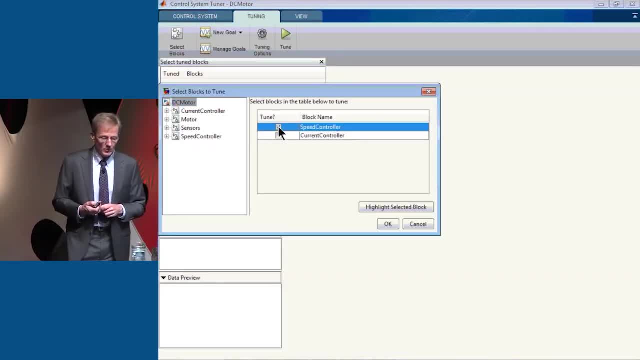 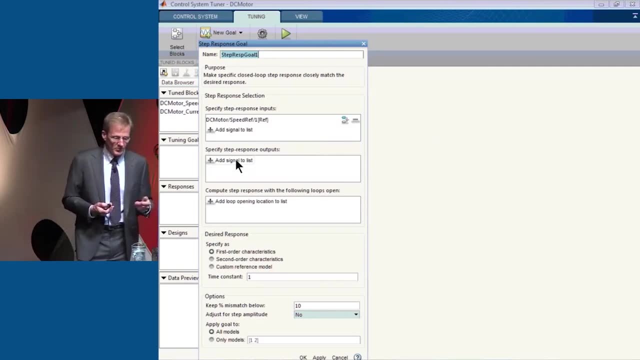 And the first thing we have to do is specify the blocks we want to design the controller around. Then we need to say which inputs we want to do, And then we say we want it to match the step response there, And so we add the signals there. 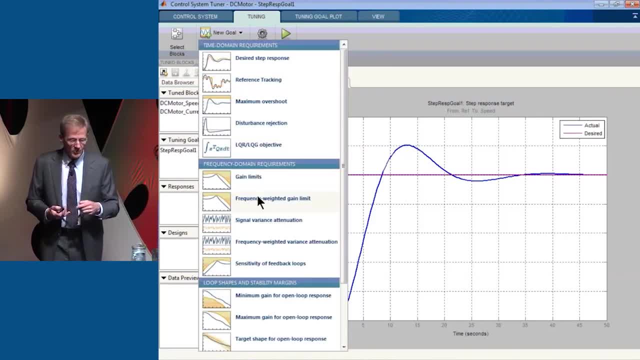 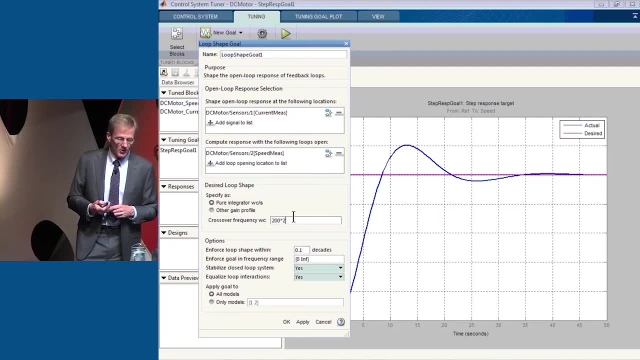 We specify the time parameter on that And there's the shape that we're looking for. And then we want to do the open loop response for the stability margins. So we specify the open loop shape and the crossover frequency there And we can look at it. 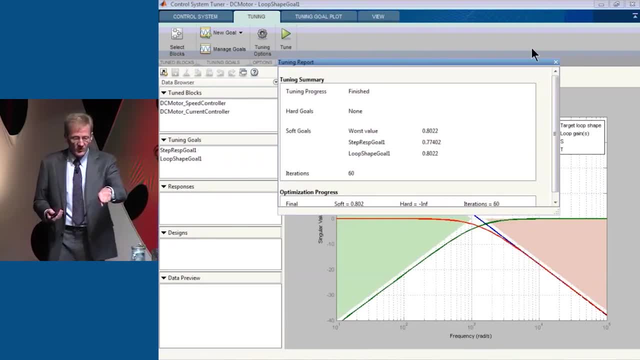 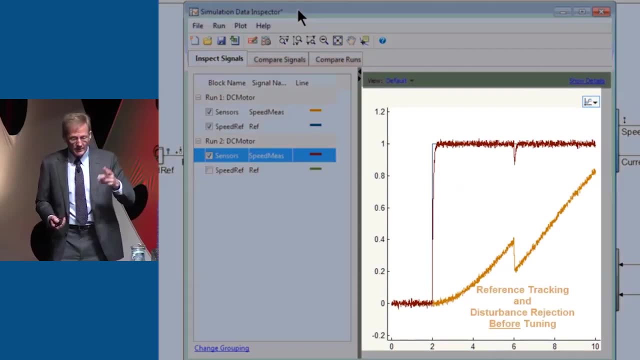 So we want it to appear in the correct versions there. Then you run the synthesis- That takes almost instantly on today's computer. Then we upload the model parameters, We rerun the simulation here And voila, there's the disturbance rejecting after the tuning there on the above. 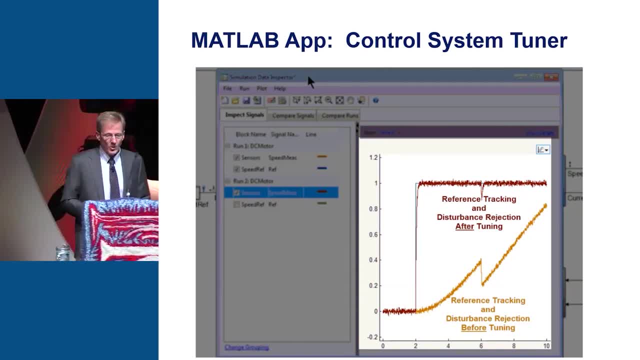 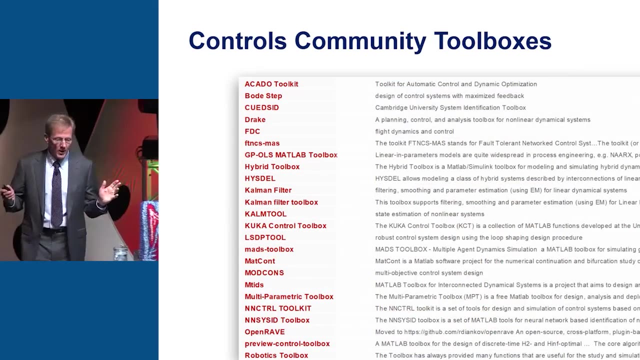 So it matches the step response and has better disturbance rejection. So we show that to people in industry and they just love it because it's so hard to do otherwise. And this app wraps it all around that. So the controls community has built hundreds of toolboxes to do different things. 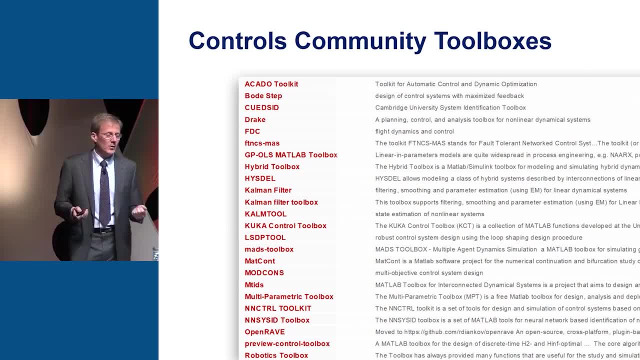 They're mostly collections of functions. So a suggestion here is: there's an opportunity to take some of the theories that have been developed and make them in a much more usable form here, which will make them more broadly there. The world is starting to expect that. 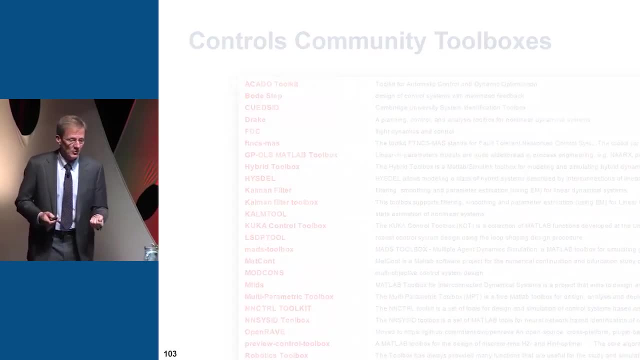 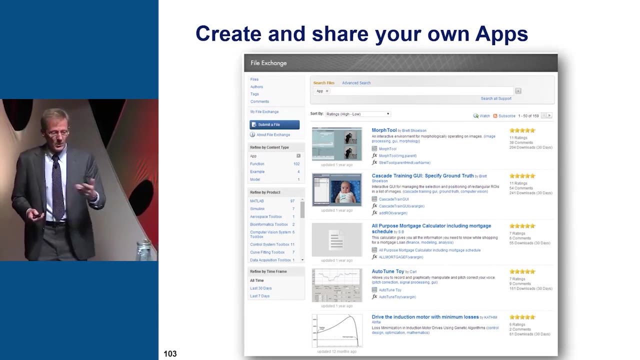 We've been spoiled by our Androids and our iPhones and expect to have an app to do these things simply and not have to program to do that. The file exchange on the MATLAB Central is a place where you can create and share your own apps. 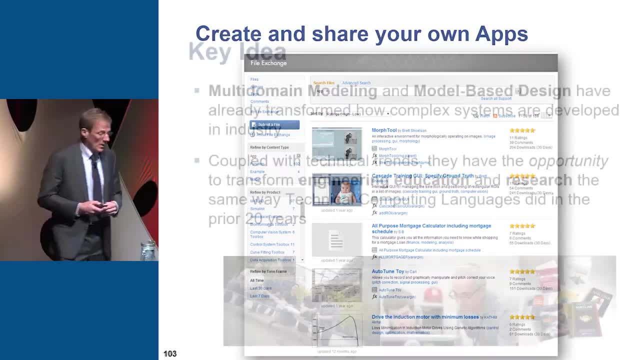 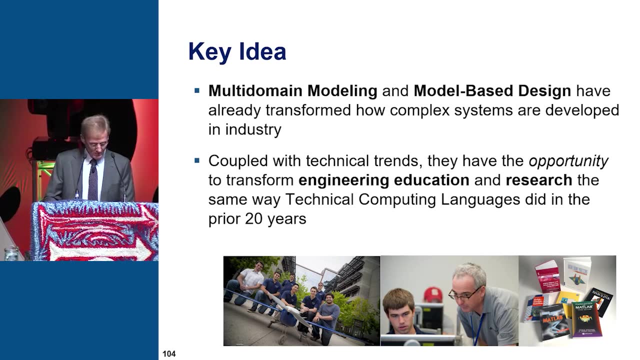 There's lots of different apps that are up there already. Okay, This brings me to near the end of my talk here. The key idea that I have been talking about here is about how multi-domain modeling and model-based design have transformed industry here, and how complex systems are doing. 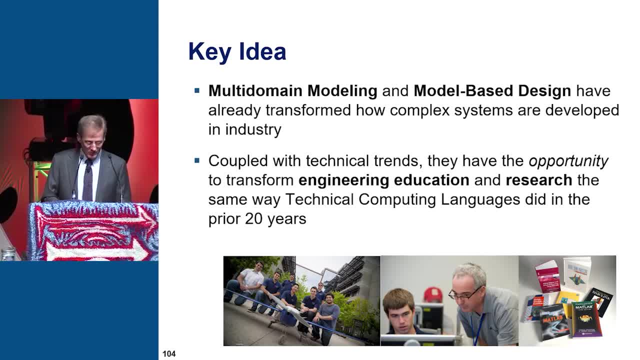 And I think there's an opportunity for this to have this. A similar type of transformation is in education here, So I guess, in summary, the current technology megatrends that I shared here are really outstanding for control applications. I think that the rise of multi-domain simulation and model-based design is going to have a far-reaching impact in education. 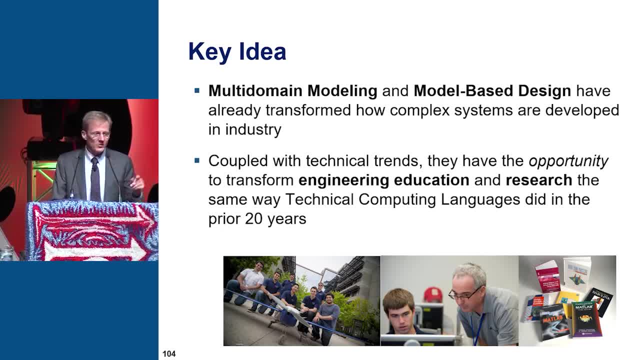 You can work at the mathematical level here with your algorithms and your ideas and concept. Push a button and it takes care of the C coding so you don't have to do that. The you know Some things I think this could mean, And I'm going to sort of be far-reaching on this a bit here. 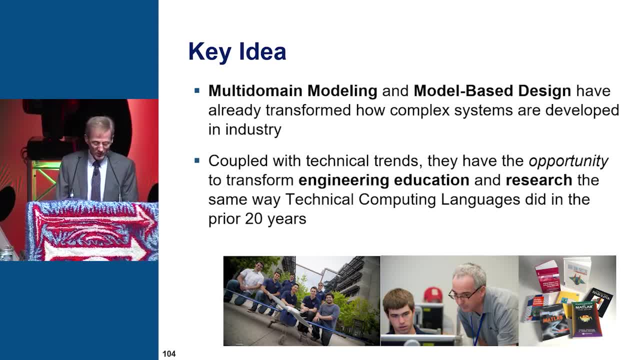 I think that hobbyists around the world, through maker fairs and other areas like that, are going to be tinkering with automatic control systems, sharing software designs and apps over social media. I think this could be the beginning of an explosion of innovation. small-scale development.